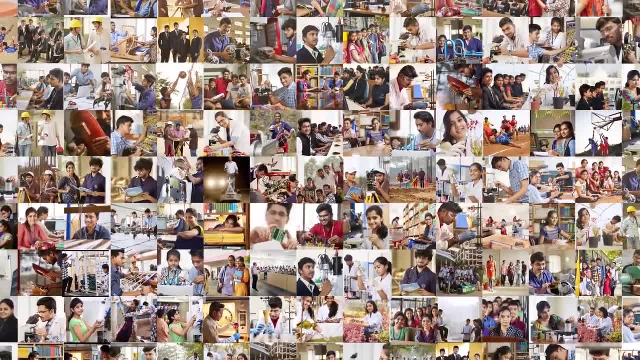 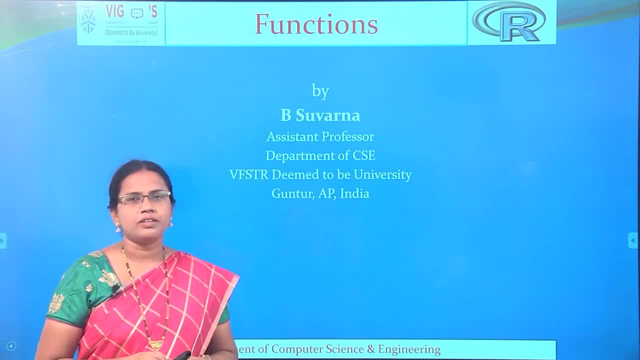 Hello, all this is B Suvarna, working as a STEM professor in the department of CSE, VFSTR, deemed to be university. In the previous lecture, we have seen what is R programming and what are the applications of R programming and what are the features of R and how to. 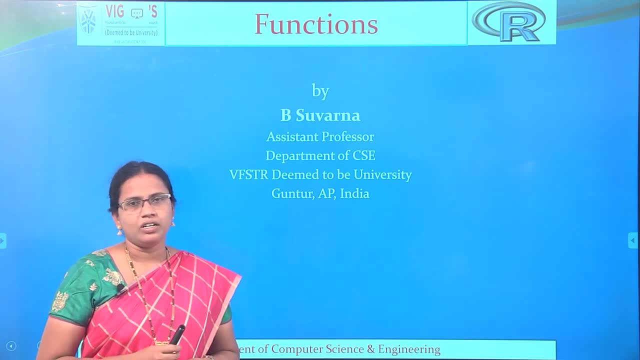 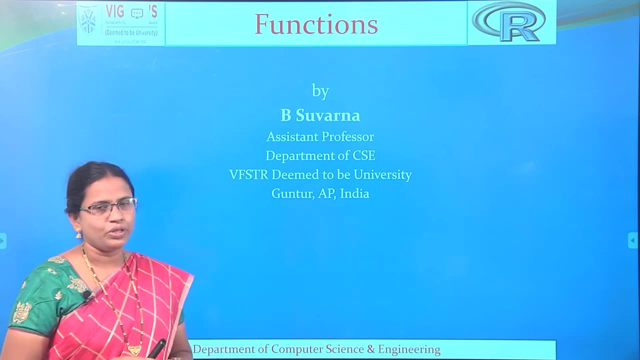 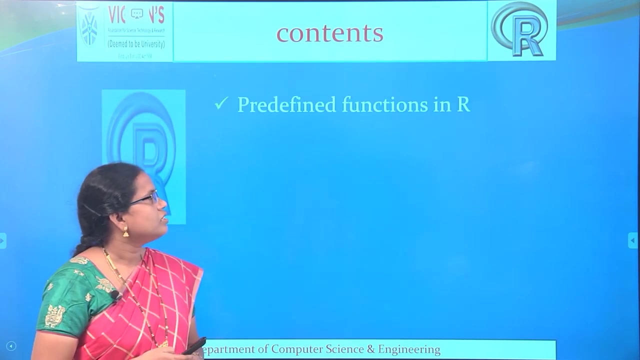 install R program, how to install R software and R studio, and after that we have seen how to work with R as well as R studio. So for the today's lecture, we will see the concept of functions. So these are the contents that I am going to display. So these are the contents. 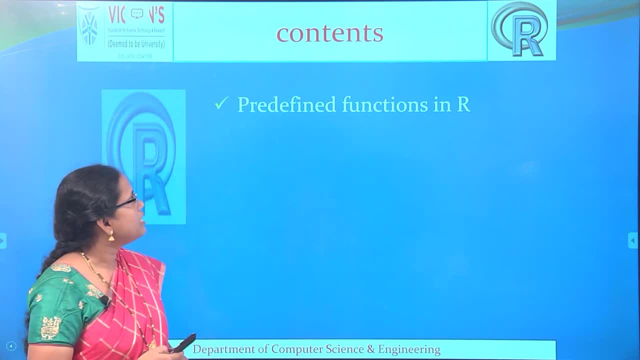 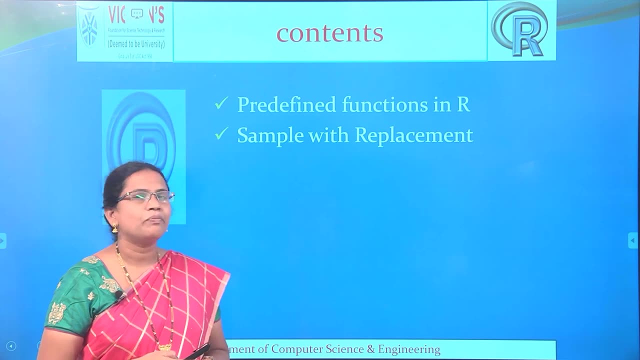 that I am going to discuss for the today's class. So we will be discussing about the predefined functions in R and after that we will be discussing about the sample function and also sample with the replacement, and we will be discussing about how to create our 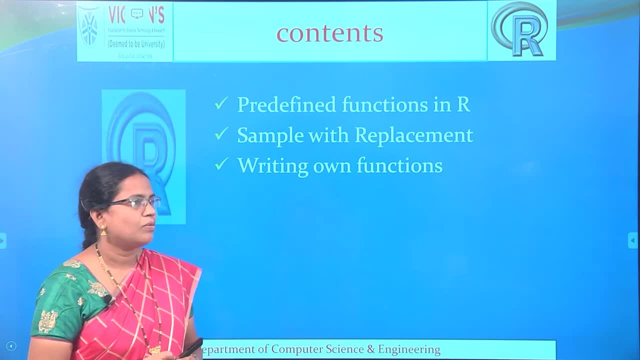 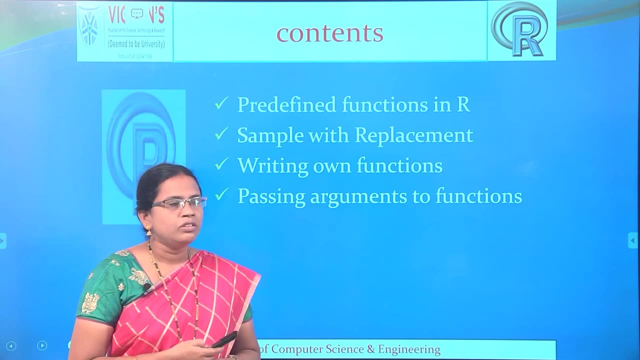 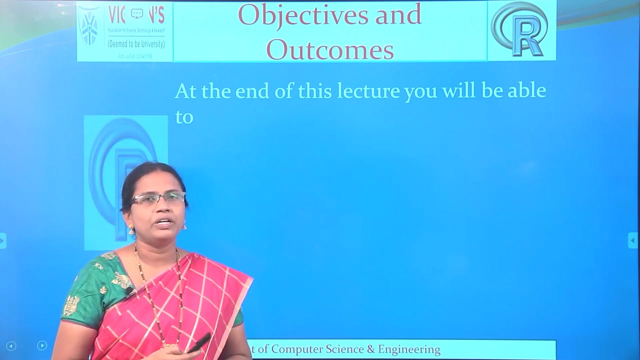 own functions in R programming and we will be discussing about how to pass the arguments to the functions. So at the end of this lecture, these are the outcomes. At the end of this lecture you will be able to know about some predefined functions that are available in 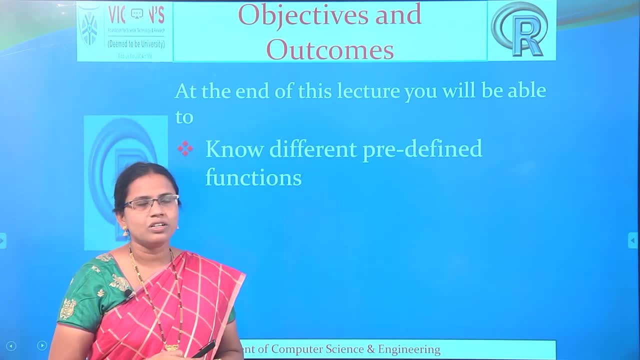 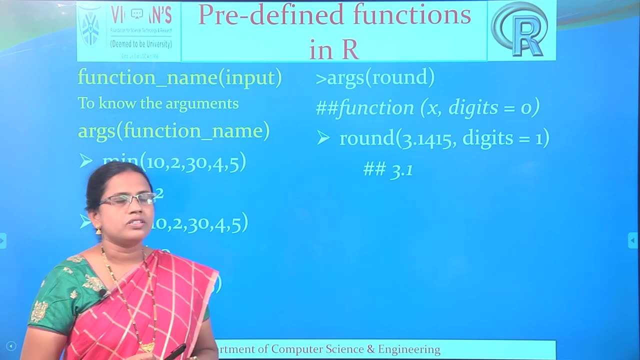 R and you will be able to create your own functions. So it is a very simple project in which we will be able to work with your work with created functions whenever required. See first. for the first, we will discuss about some of the predefined functions in R programming language. So, for example, if 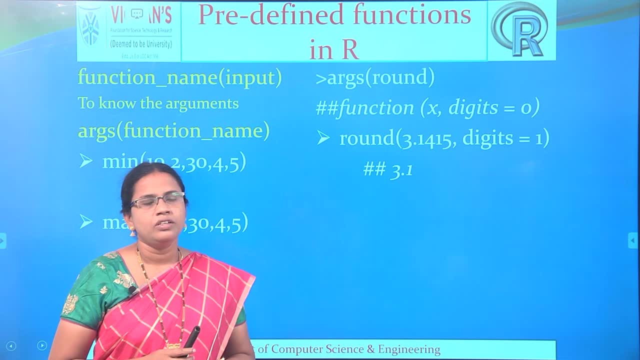 you want to find the minimum element for your given set of elements. so if you are working with arrays, so then if you want to find out the minimum element for the given set of elements, then you need to write minimum 20 lines of the code. so here in the R programming you 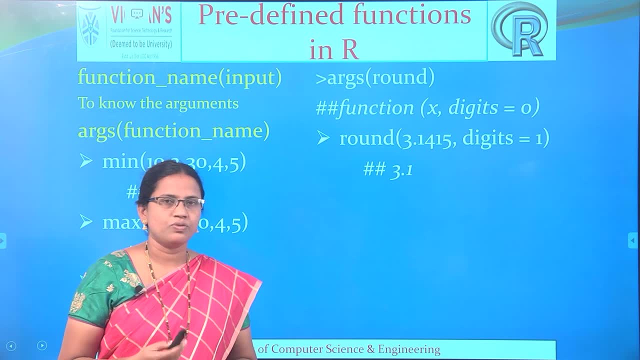 need not write all 12 lines. So I am going to show you two ways where the minimum elements all those 20 lines of code, okay, all those 20 or 30 lines of the code. So instead of that you will write, you will perform the minimum element for a given set of element within. 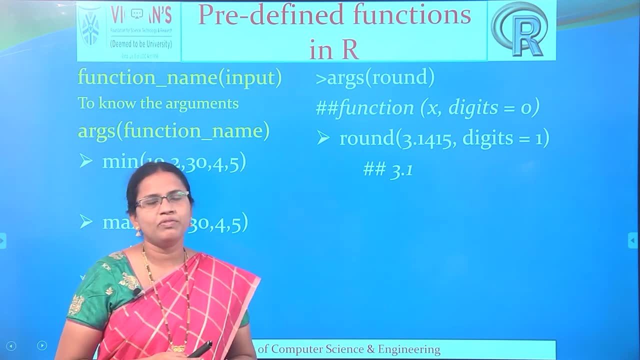 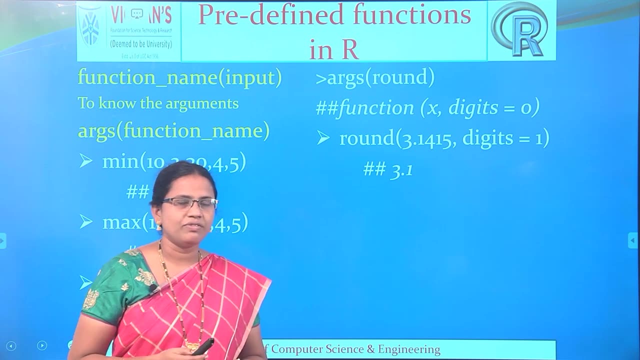 one line, So okay. so by making use of the minimum function, we will find out the minimum element of the given set of the elements. okay, So for everything, there are predefined functions in R. by making use of that, okay, we will make our job very easily, okay. 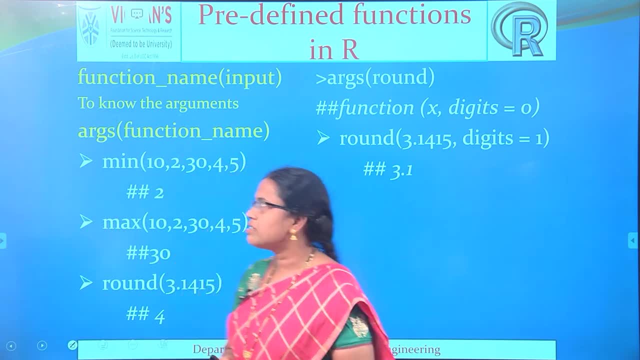 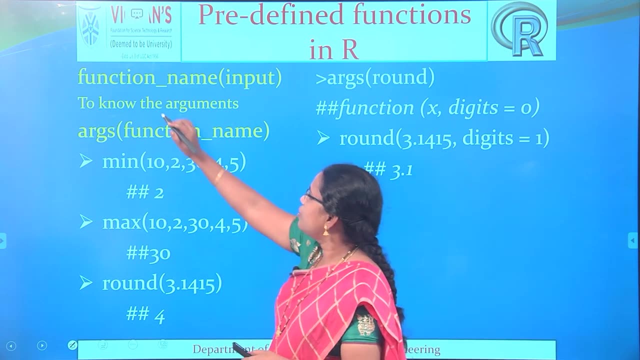 So next to find the minimum element. okay, first let us see how to write, how to make use of the functions, the predefined functions in R. okay, So the first one is: you have to follow this syntax: so: function name of the input. okay, So, function name of the input. okay, So. 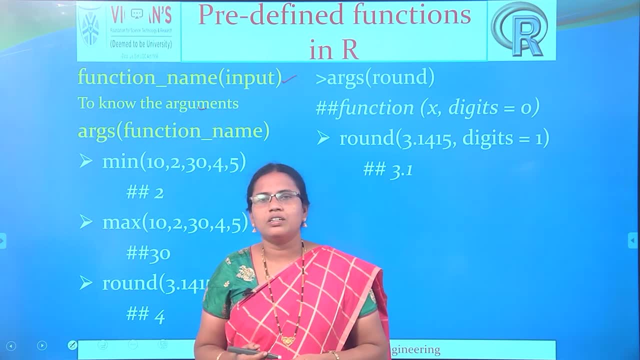 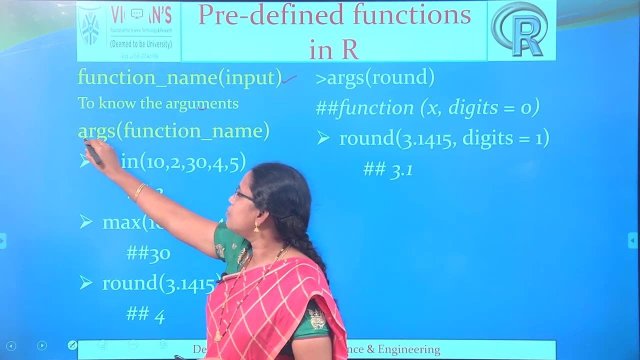 and to know the arguments. if you don't know how to use it and what are the parameters for that function, then there is a command that is called as arguments of the. okay, So then there is a command. okay, So if you don't know the arguments, then there is a function. 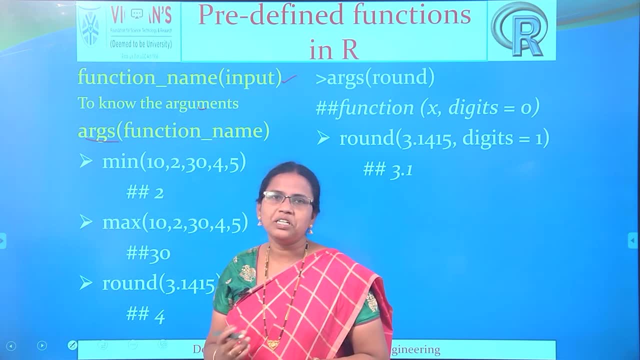 a command that is called as args. So args is nothing but arguments function okay. So by using that function, you will be able to know what are the parameters available for that. arguments function okay. So args of function name: okay. So you have to make use like this: 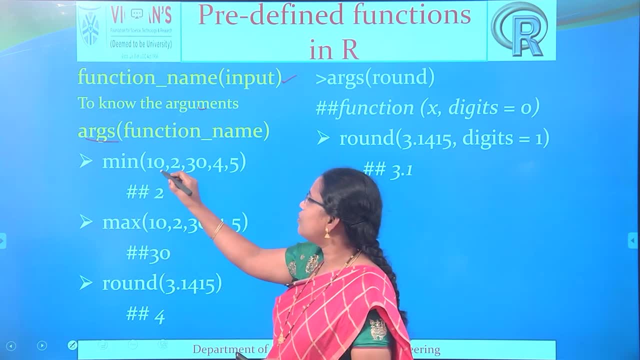 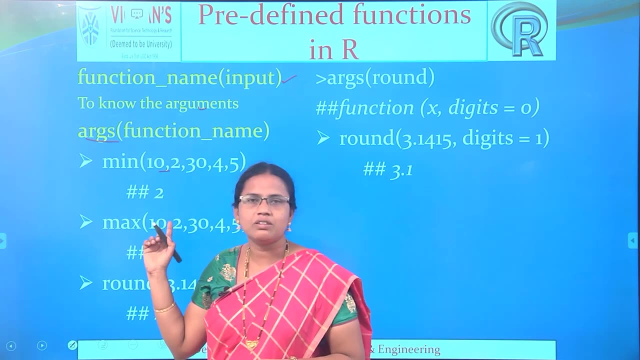 So, for example, to find the minimum element for a given set of element: okay, So these are the elements. okay, So these are the elements 10,, 2,, 30,, 4 and then 5.. So this is the given set. 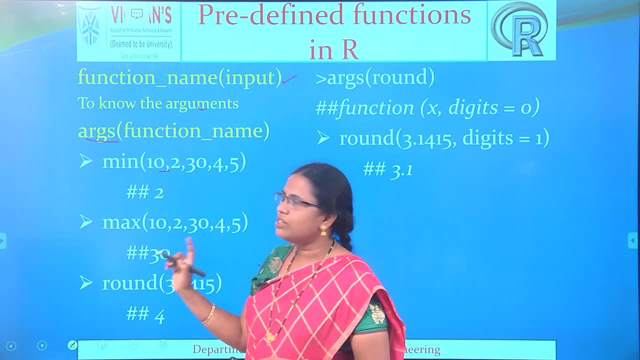 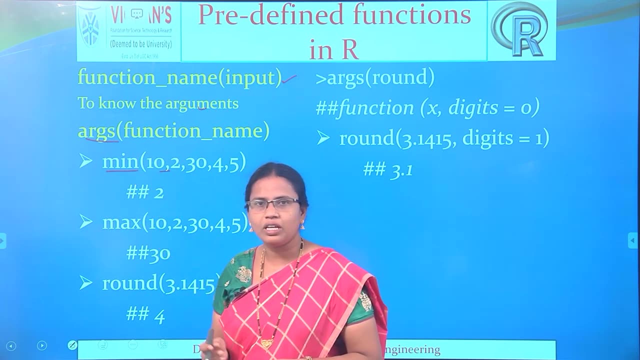 of elements. If you want to find out the minimum element for that, okay, So you have to make use of the function that is called as min. So min of you have to give your input. okay, You can give the input here or you can give the variable for the input. okay, So I have given set of inputs. 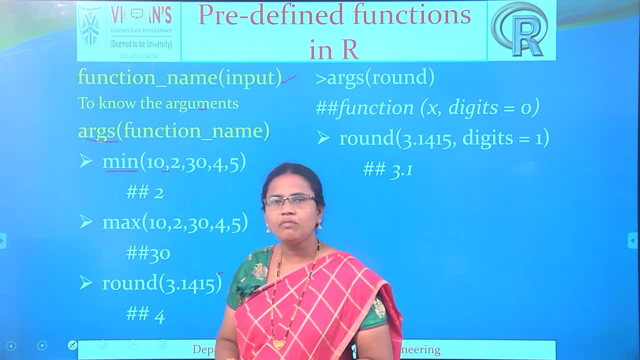 here. So 10,, 2,, 30,, 4, as well as 5.. So when you execute this command in R console, you will get okay. So you will get the output like this: What is the minimum element for a given set of? 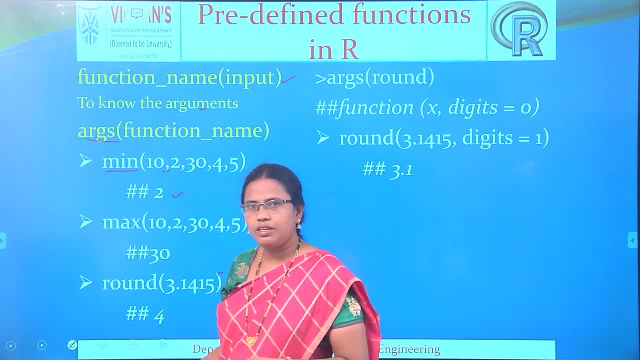 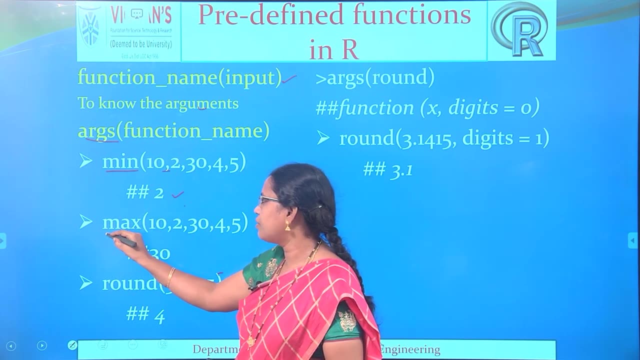 elements. The minimum element is true, okay, So next let us see max Suppose. if you want to find out maximum element, okay So, maximum element. for that we have a function: max of. okay, So, max of. you need to give the input like this: okay, So, this is the input that I have given. okay, So? 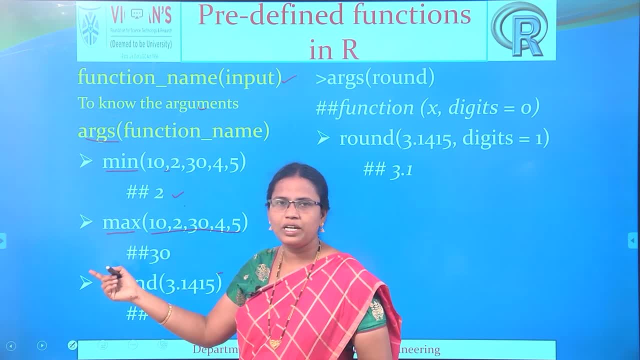 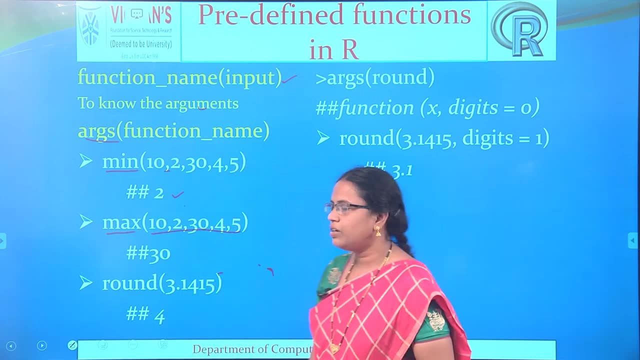 when you execute this in R console, you will be able to get the maximum element for a given set of the elements, And next let us see other function. okay, So that is round. okay, So this is my input: 3.1419.. 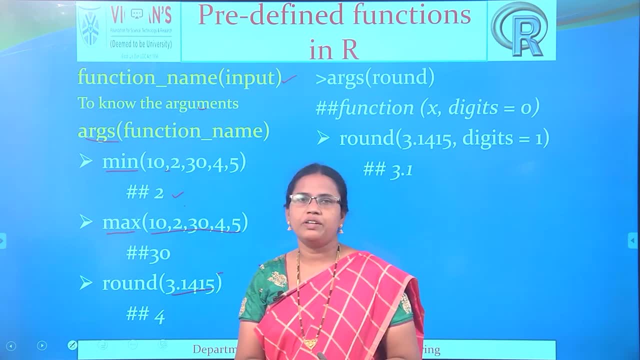 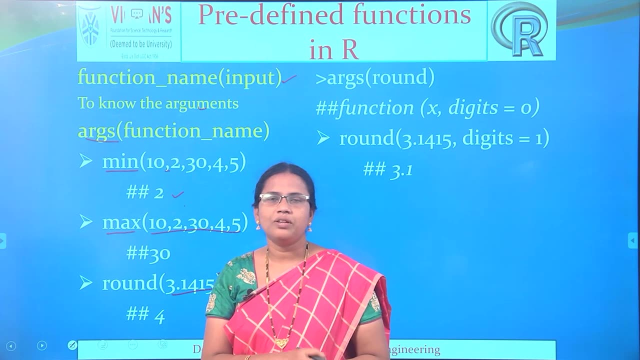 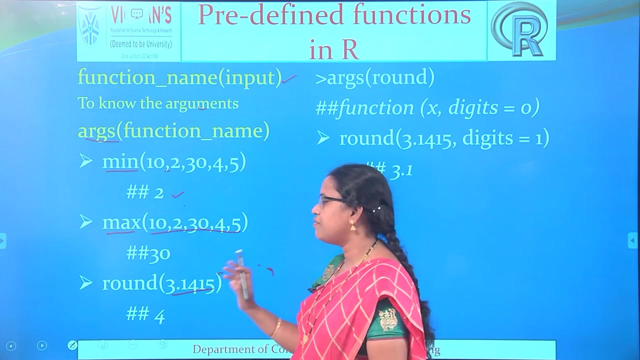 3.1415,. okay, So, whenever you have a floating number, okay. So then if you want to find out the round value of that number, then you can make use of the round function. So, round of okay, if you give some number. okay, So 3.1415, it is rounding the okay number given number. 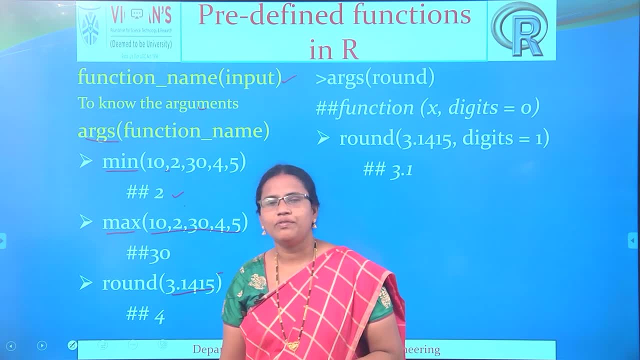 And then when you give this, when you execute this command round of 3.1415, it is printing the value as 4.. So that means it is rounding the value. So after 3 point: okay, So it is making the. okay. So floor seal round. okay, So 3 point. 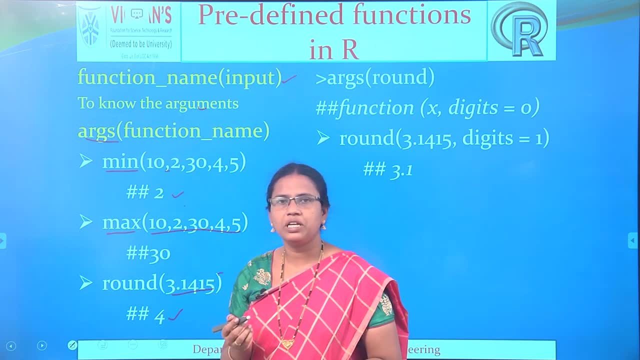 after the 3.1,. okay, So after the point, whatever we have, it is doing the sealing round. okay, So 3.1, it becomes the 4,. okay, So I do not want to print all these elements. 3 point: 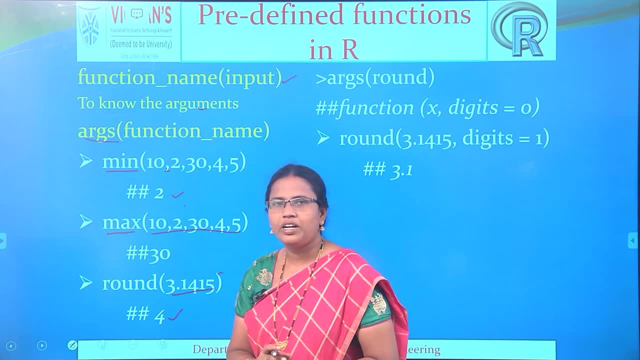 if I want to see the actual number, okay. So 3 point: what is the thing? what are the numbers that are available? after point: If I want to see, I can print the number, okay. So 3 point: 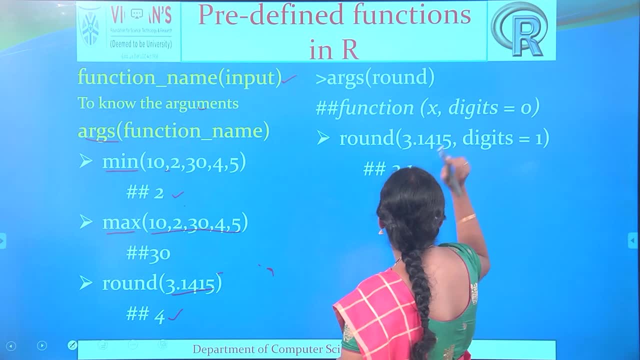 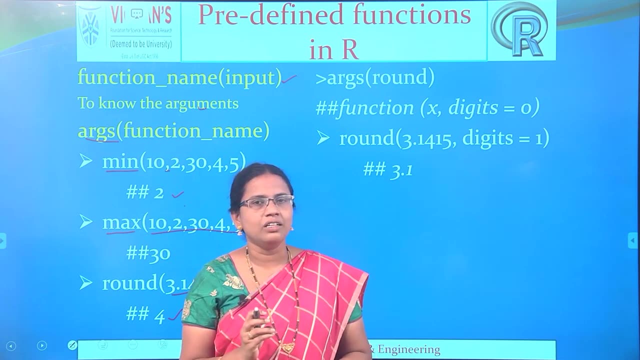 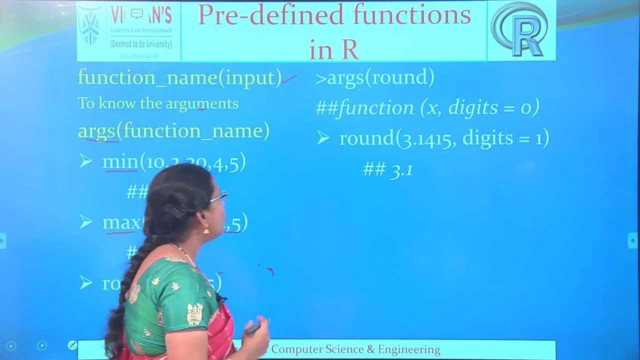 then at that case I have to, okay, So I have to give the digits, So how many digits that you want after the point, then you can specify it by writing those. okay, by writing the numbers, the required numbers, in the digits. okay, digits parameter. So I do not know about what are the 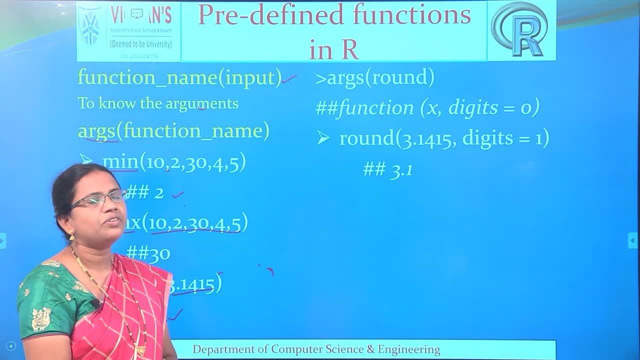 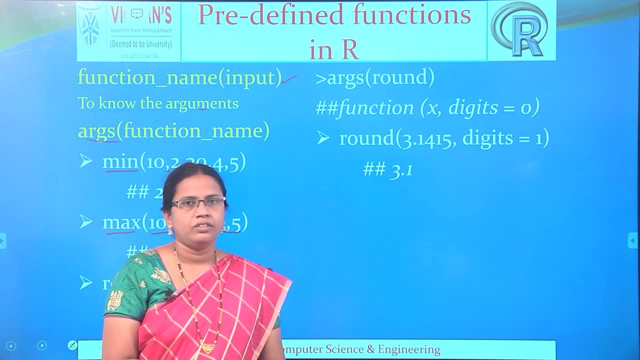 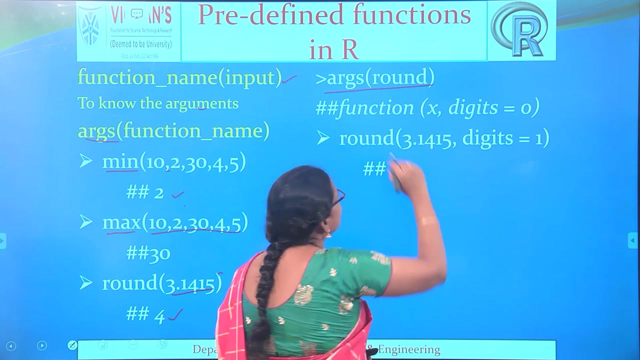 parameters available in the round. I have already told that. what is the command for for: to know the parameters of a function. okay, So args is there. So by using that args function, we can know that what are the parameters available for round. okay, So when I execute this command or when you execute this command, 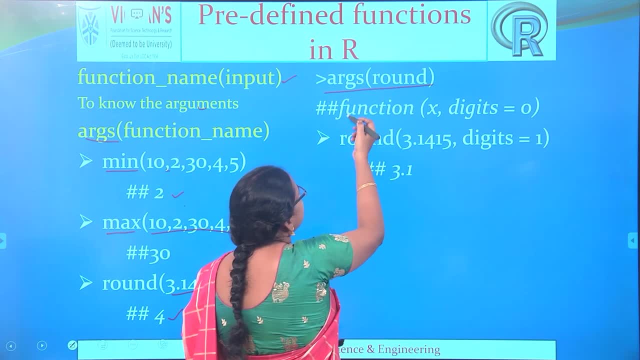 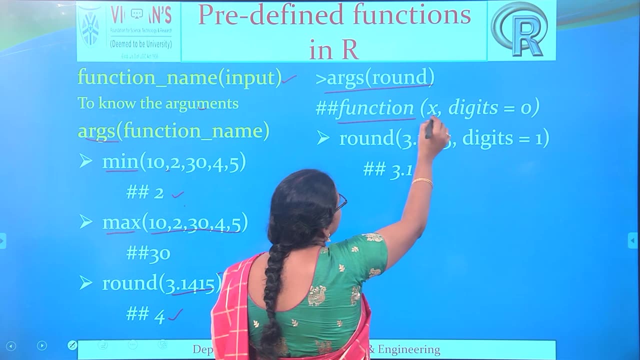 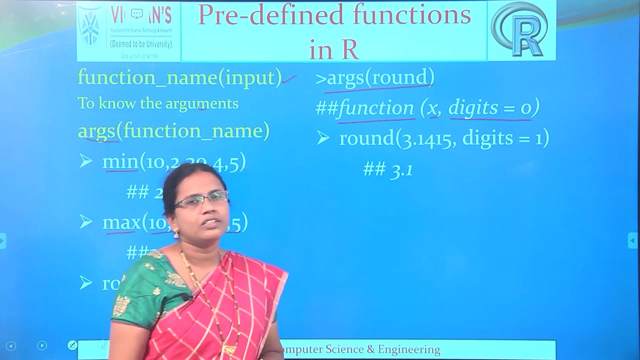 args of round. okay. So then it is printing okay like this: So function of: okay. So of course, for everything it prints like this: function of x comma. So this is the input. okay, So you need to give the input here and then digits equal to 0.. It is printing like this: 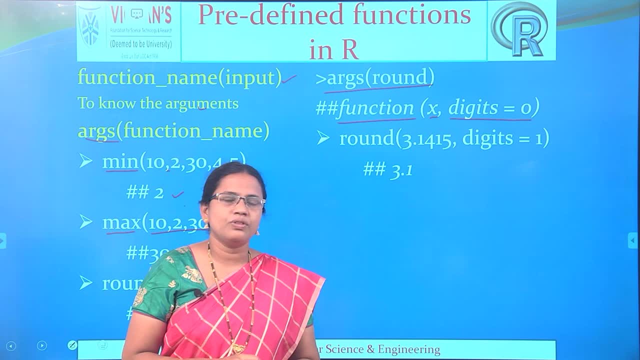 By default. it takes the input. okay, So you need to give the input here and then digits equal to 0. It takes the digits as 0, okay, So that means 3 after it will not print or it is doing the. 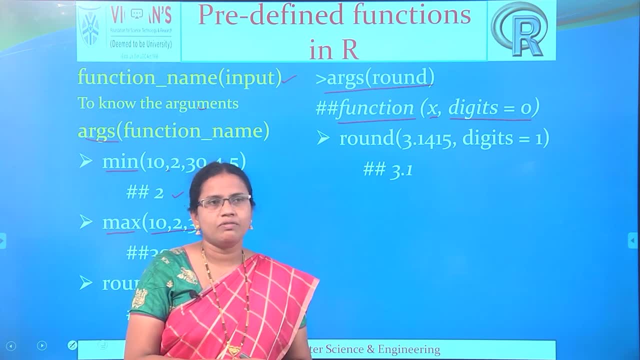 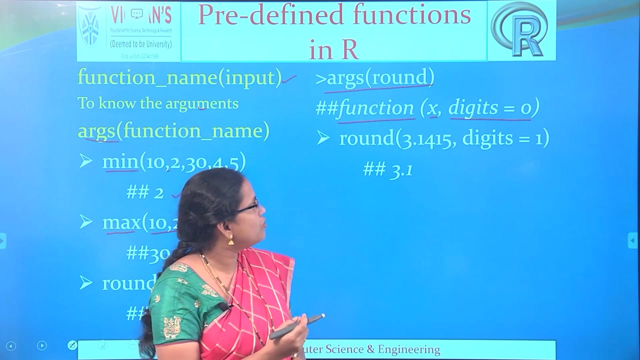 rounding operation. So by default, its digits values are 0.. If you want to print after the 1, after the point, if you want to print after the point, then what you will do, You have to specify the digits Here. see here: I want to see, okay, So 3.1415,, I want to see 0.1. Then, at that case, 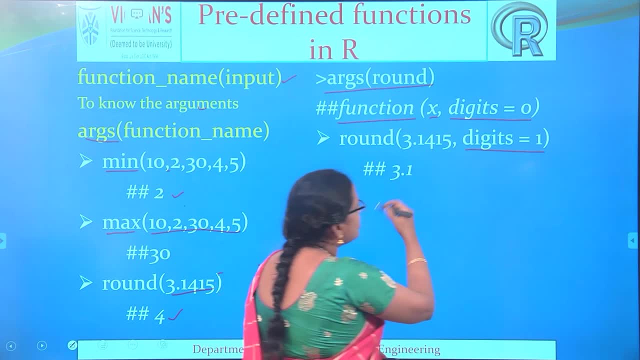 you need to specify the digits So you can remember here after the point: I want the next number, okay, So I want the next number, So that is 1.. So at that case you have to specify the digits- is equal to 1.. Suppose: 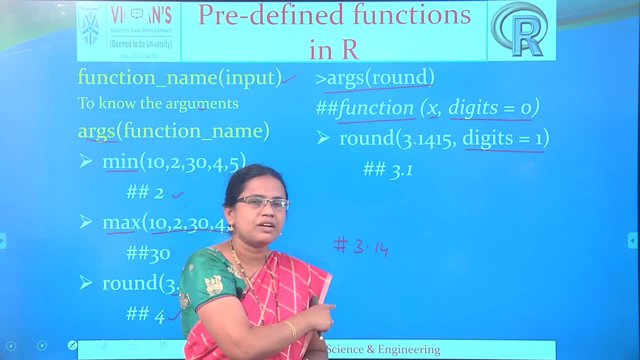 if I want to print the number as 3.14.. So that means after the point: how many numbers are there? There are two numbers, okay, So for that you need to write the command like this, okay, So? 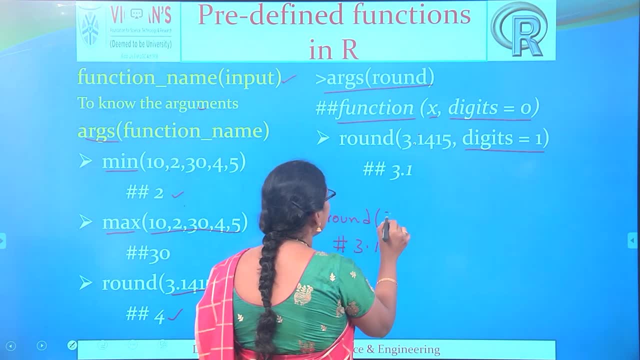 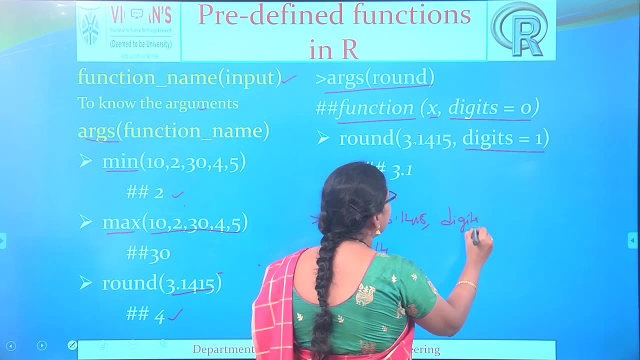 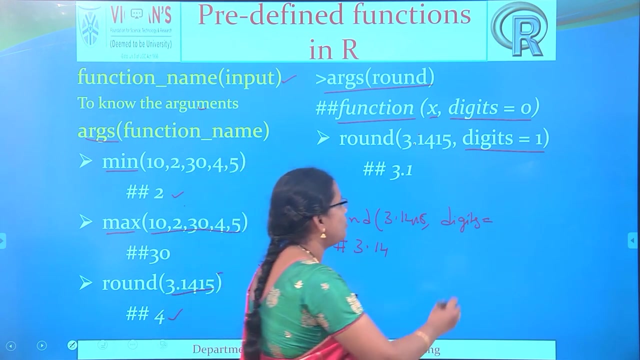 round off. this is the function. okay, So round off. 3.1415 comma. okay, So digits is equal to okay, So how many digits we have to write? How many digits we required? We required two digits after the point, okay, So at that. 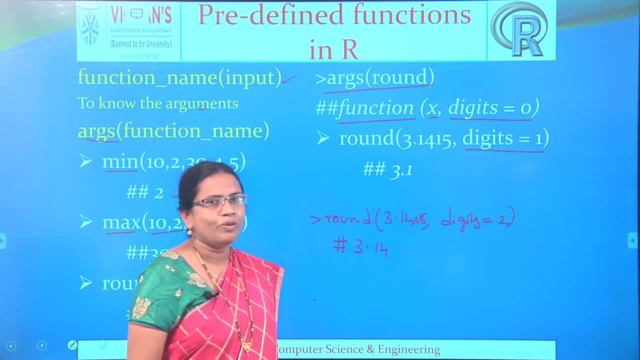 case you need to specify digits- is equal to 2.. So when you execute this command, you will be able to get this 3.14,. okay, Suppose, if you want to see three numbers after the digit, then what you will do? You have to write the command like this: So at that case you need to specify the. 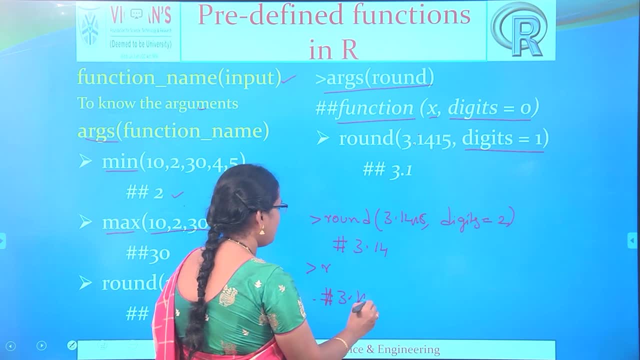 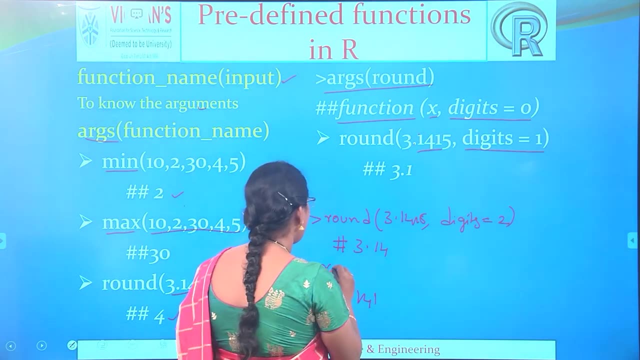 command. Suppose: if you want to see, okay, if you want to write 3.141,, okay, So I want these three digits. So then at that case you have to write okay, So you have to specify the digits. 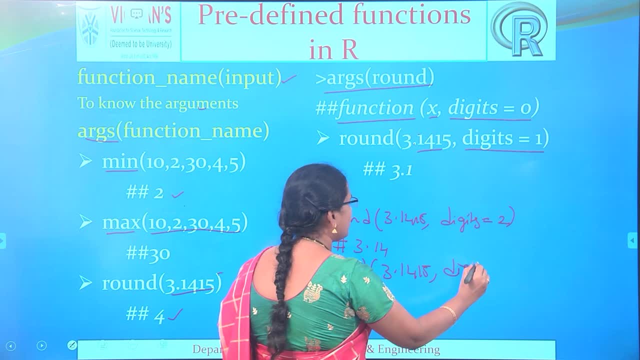 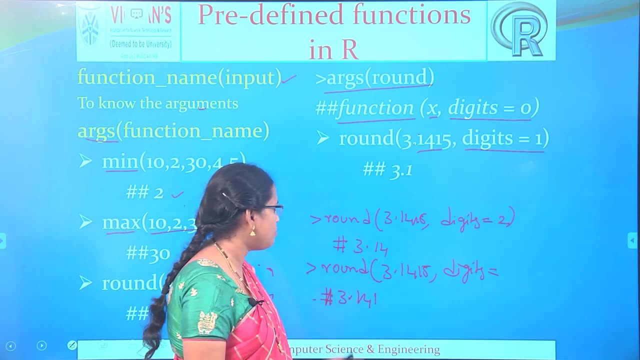 okay. So that is digits is equal to what is the number that we need to write here. So I want three numbers after the okay, after the point, So I have to write the digits as 3.. So like this we: 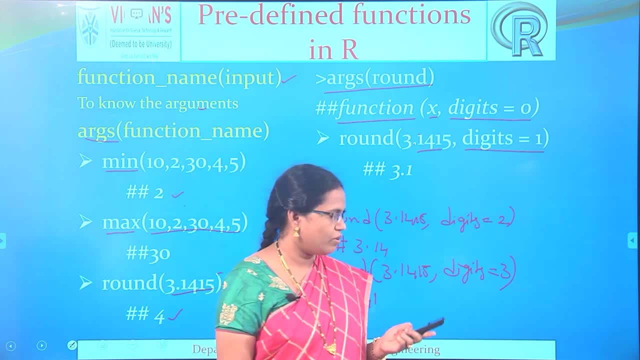 will work. the predetermination. So I have to write the digits as 3.. So I have to write the digits in r. Okay, So next let us see some of the predefined functions in r, Suppose, if you want. 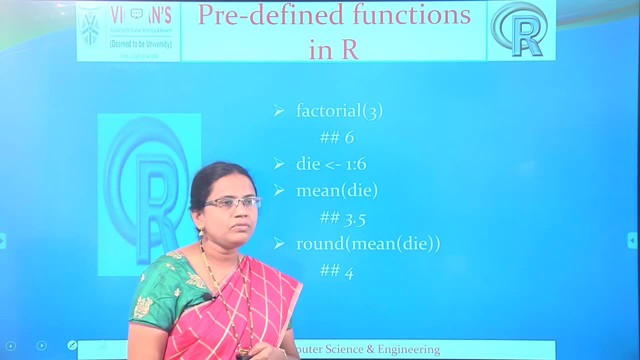 to find out the factorial value for a given number. right, factorial value for a given number. then there is a function that is called as factorial. okay, So, factorial of 3, factorial of 3, okay, So factorial of. you have to pass the input: that is 3, okay. So when you execute this, 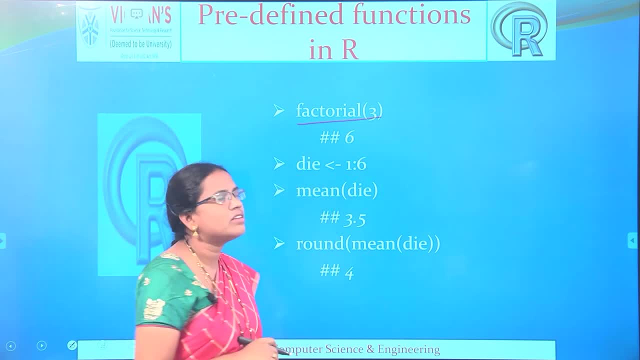 command factorial of 3, okay, So when you execute this command factorial of 3, okay, So when you it is printing the value as 6.. So let us see the other example. So this is the command die is. 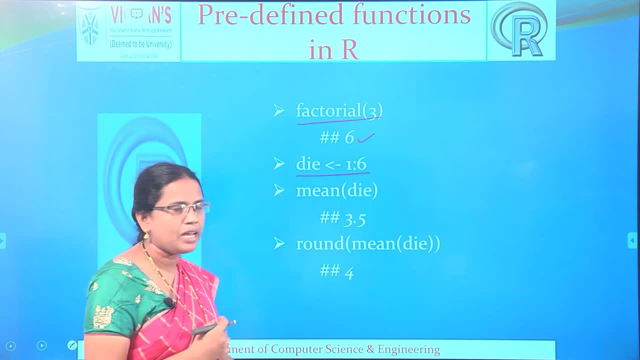 equal to 1.6.. So this is my input and I am going to pass this input to the mean of die. Suppose there are numbers. So when you write, die is equal to 1.6, 1 colon 6.. So that means you will have: 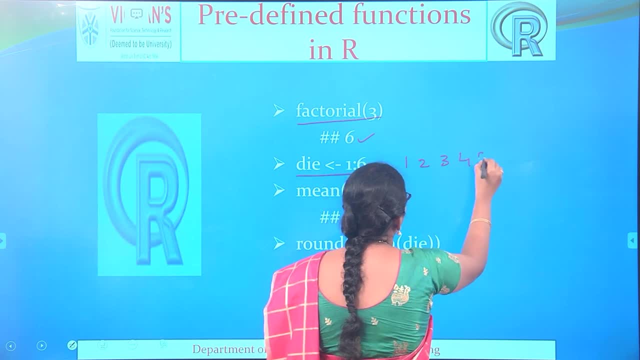 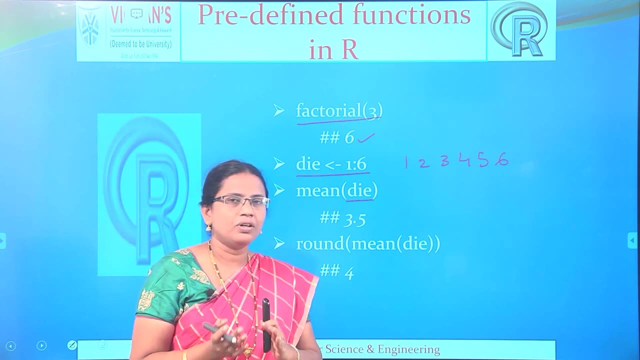 a numbers 1,, 2,, 3,, 4,, 5, as well as 6.. That means you will have a numbers starting from 1 to the 6.. So 1, colon 6.. You are going to start your number with 1 and then ending with the number 6.. 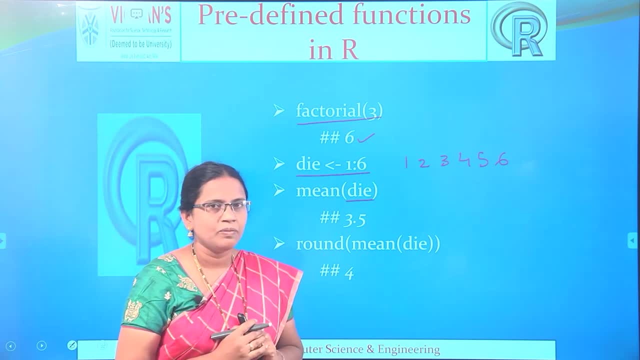 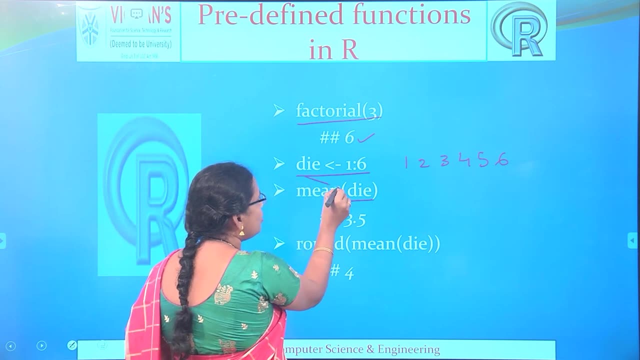 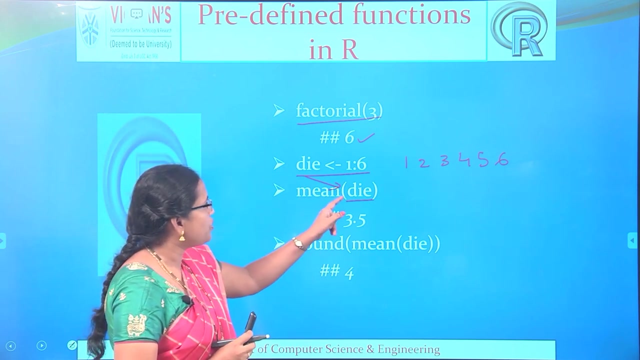 Suppose, if you want to find out the mean value for those given numbers, then at that case we have a function that is called as mean, So mean of die. So this is the input that I have passed here. I have stored my input So in one variable and I am going to pass that input to the mean. 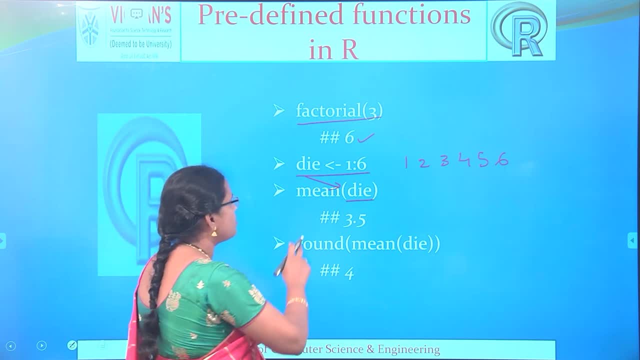 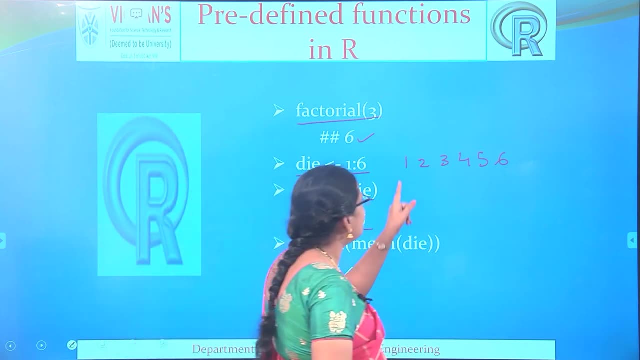 function. So mean of die. So when you do this mean of die, you will be able to know that this is the mean value. So mean of 3.5.. What is the mean value for the given numbers? So the mean is nothing but 3.5.. The average of the given numbers that 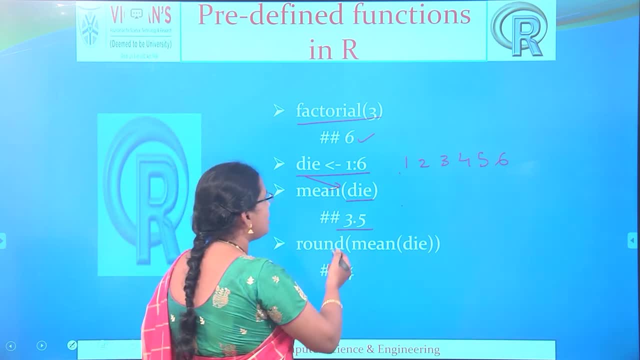 is the 3.5. And then next, if I want to see, if I want to round this 3.5. So the obtained input is 3.5 and if you want to round that mean value, then what you have to give, So round of mean of. 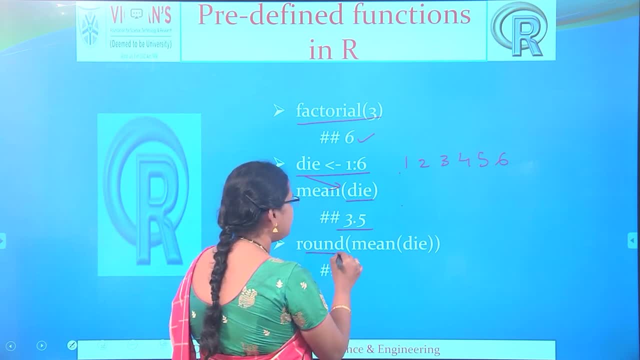 die, So you will be able to know that this is the mean value. So if I want to see, if I want to round this 3.5.. So what you have to do, You are going to round and for which you are going to do. 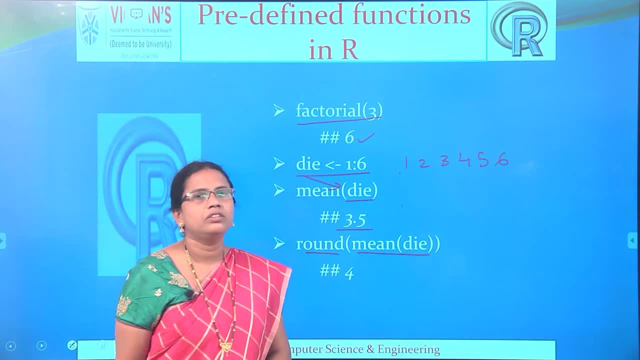 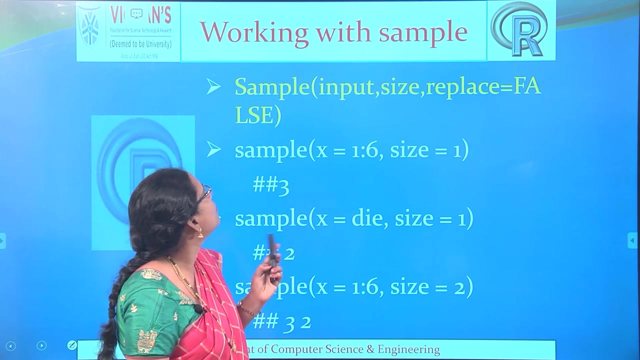 the rounding operation for the calculated value of the mean of the die. So when you executed this, when you executed this in R console, it will be able to get the value as 4.. So this is the advantage with the, this is the advantage with the R programming. So next term, 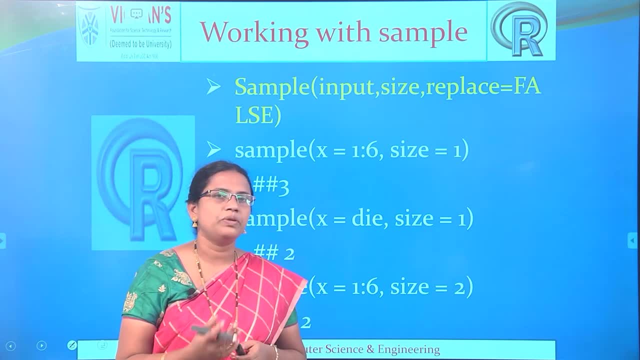 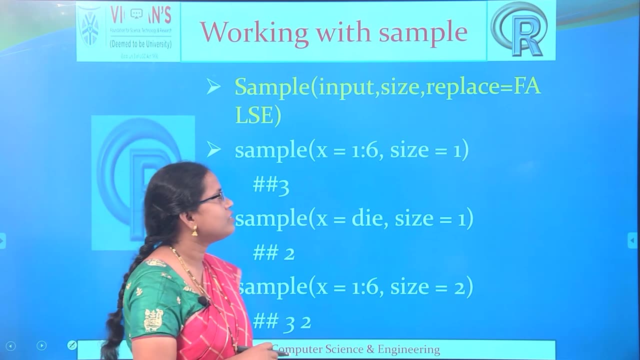 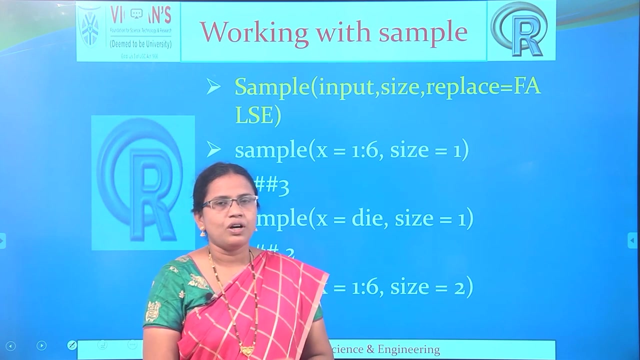 So like this we are. we have seen several examples. several predefined functions in are ok. So the next concept is working with the simple, ok, working with the sample. Suppose, so if you have, if you have 10 numbers, ok, so in your data set, then if you want to, 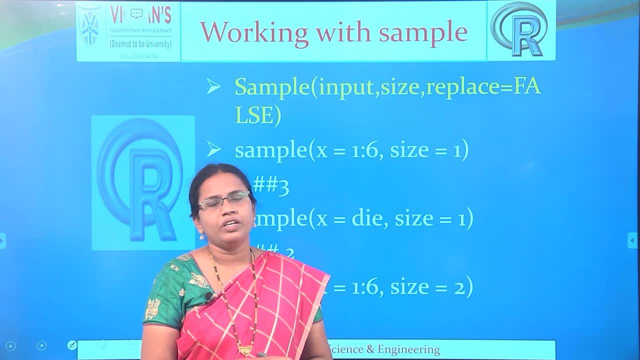 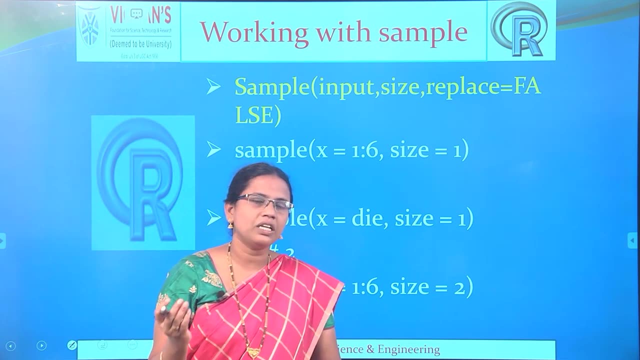 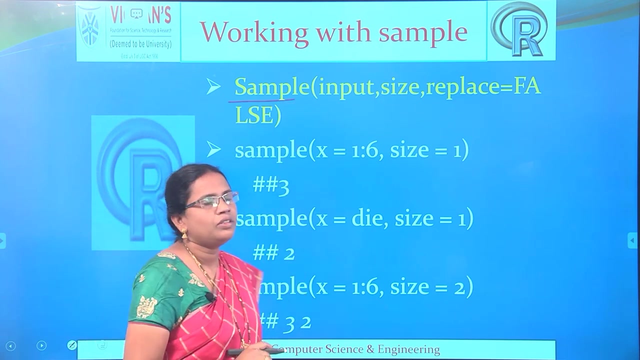 extract 2 numbers or some set of numbers, then ok. if you want to extract some set of numbers randomly, then there is a function. ok, so to select the numbers randomly from a given set of input. ok, so that function is called as sample. ok, So sample is a function by using this. 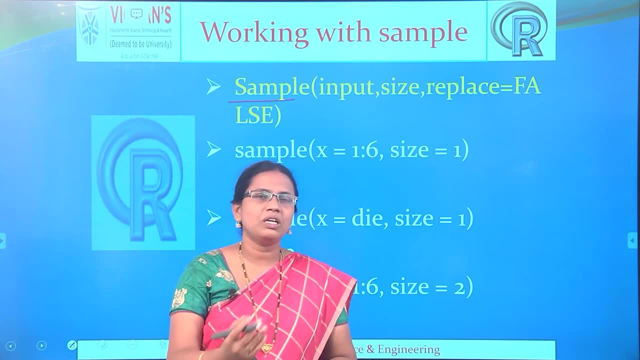 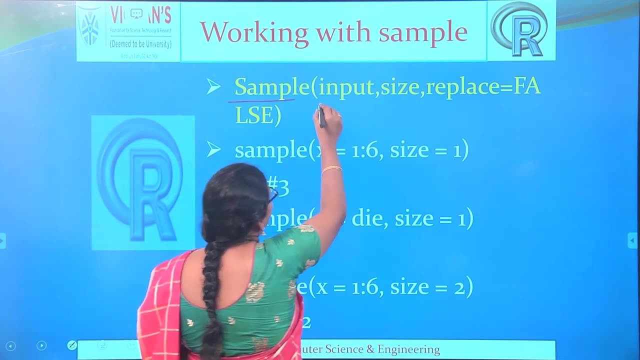 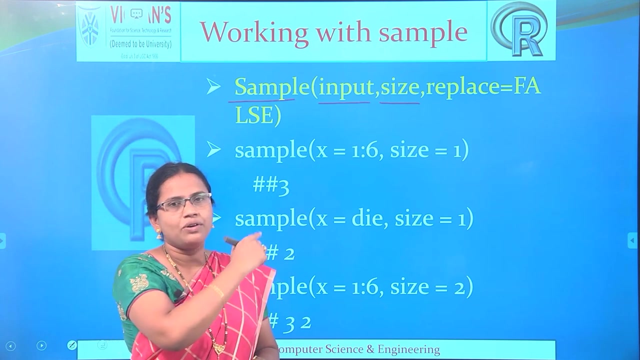 function. we will extract some numbers randomly from a given set of the input. ok, So, sample of input comma. so the syntax is: sample of input. you need to pass the input here and the size. ok, so how many samples or how many numbers that you want, you have to, ok, specify the size over. 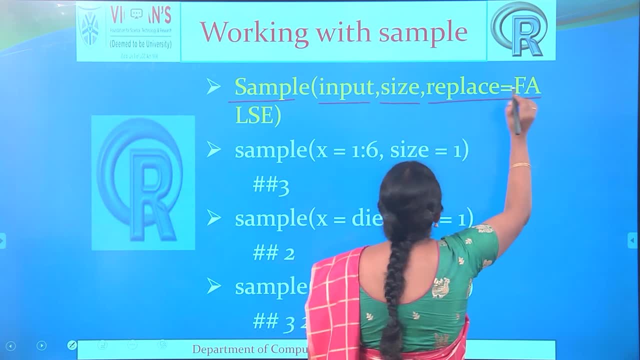 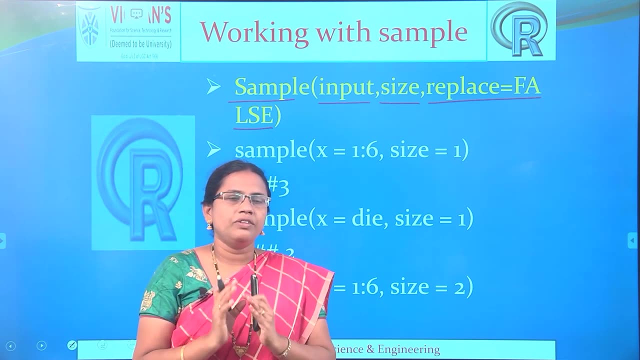 there size comma. replace is equal to Replace is equal to false. ok, So by default. ok, so false is there for the replace. that means that if there is some, if there is a data and if you want to extract some numbers from that, 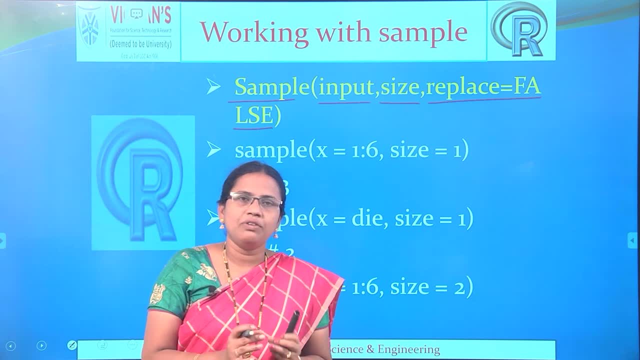 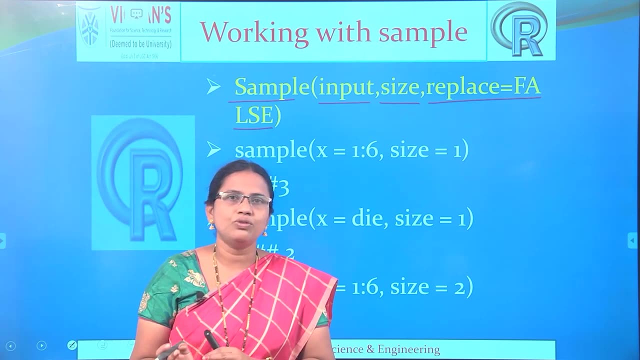 and after performing some operations on that data, if you are going to place, if you want to place those numbers into the data set, then you have to write it as: replace is equal to true. ok, So by default, false will be there, ok, So if you want to include those sample, ok, if you want. 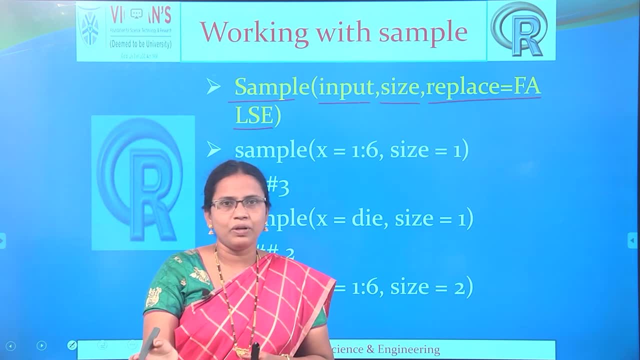 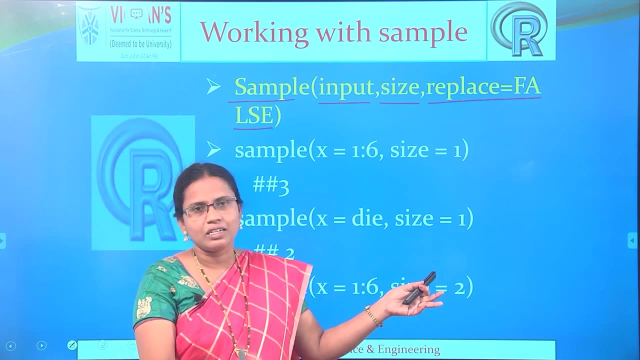 to include the selected sample, then you need to place that sample by making use of the replace. So replace is equal to true means ok, you are going to place that selected sample into the data. and replace is equal to false means you are not going to place that selected sample to the data. 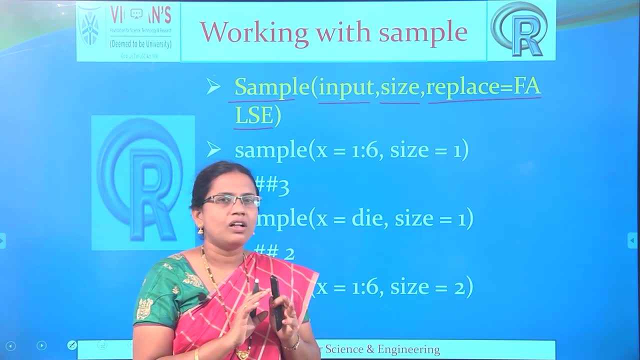 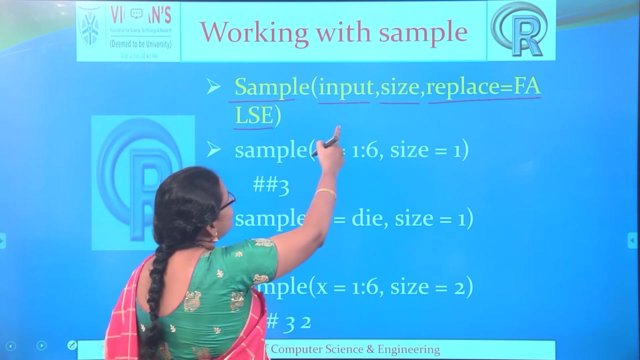 ok, so to try to understand. So replace is equal to false means we are not going to include the selected sample. ok, to the given data set. Replace is equal. replace is equal to true means we are not going to include the selected sample to the given data set. right, So sample of input. 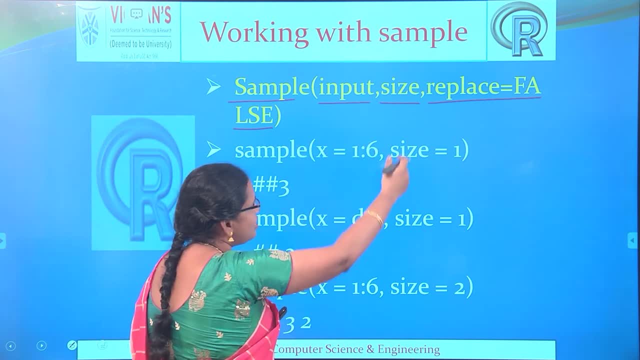 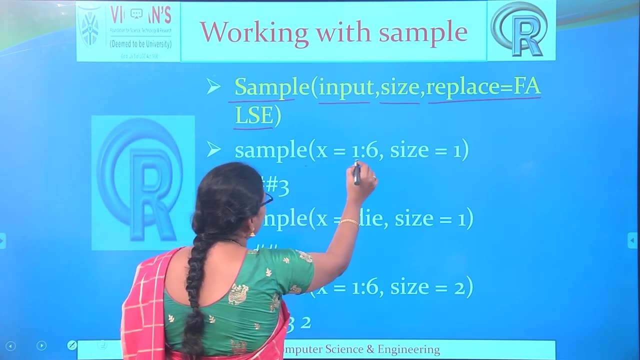 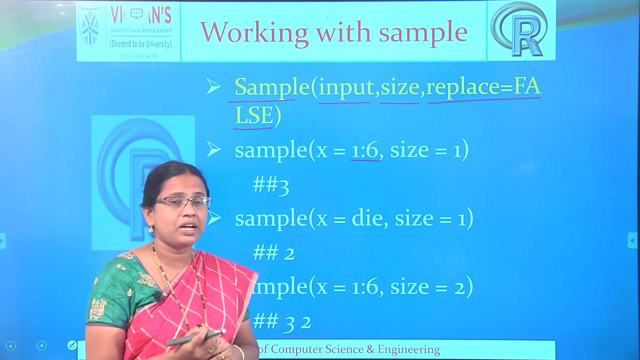 comma size. replace is equal to false. ok, So let us see it again. let us discuss about the replace later and let us see the first sample. of x is equal to 1 colon 6.. So what is the input given? x is equal to 1 colon 6,. that means we are going to have the input, the numbers. 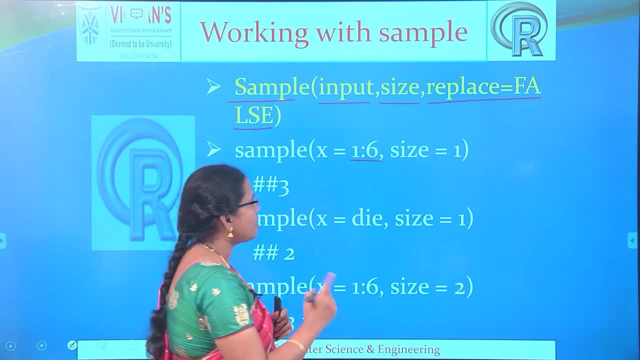 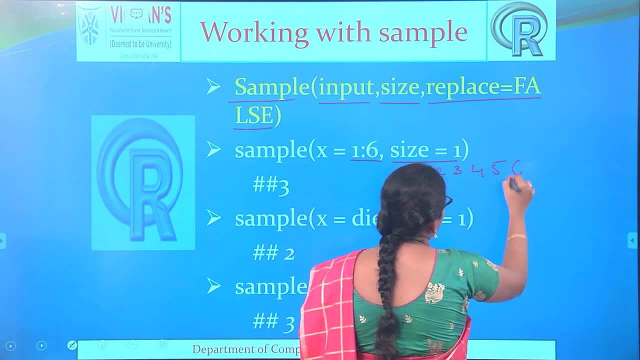 the set of numbers from 1 to 6, ok, So, and size is equal to 1.. So, from the out of 6 numbers, 1,, 2,, 3,, 4,, 5, as well as 6,, assume that this is the input and if you. 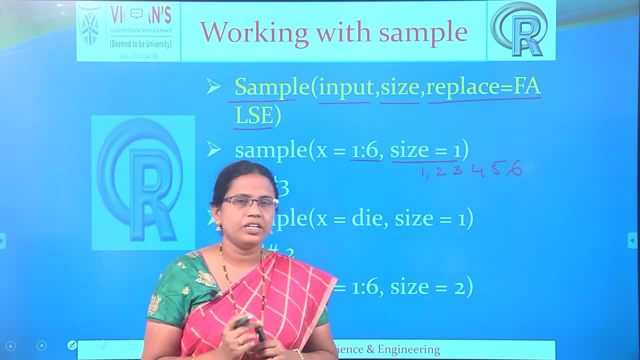 want to extract only one number from that. ok, so then you need to write: you need to specify the size as 1, size is equal to 1, ok, So if you specify the size is 1 and when you execute this, 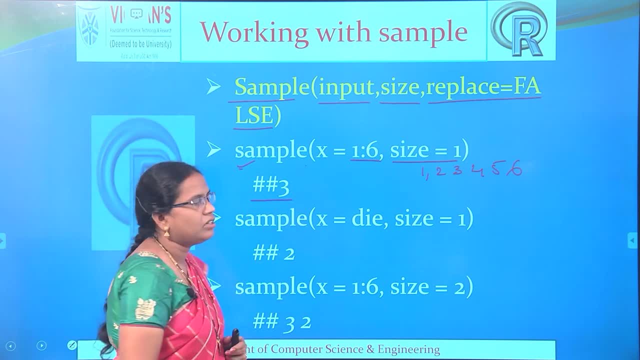 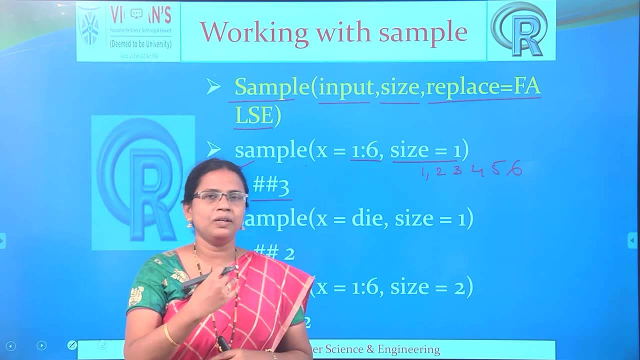 command in the R console, you will have the output like this: ok, So when you execute the same command once again, you will have the other number. ok, When you execute the same command, you will have the other number Like this: you will select the random numbers, ok, from a given. 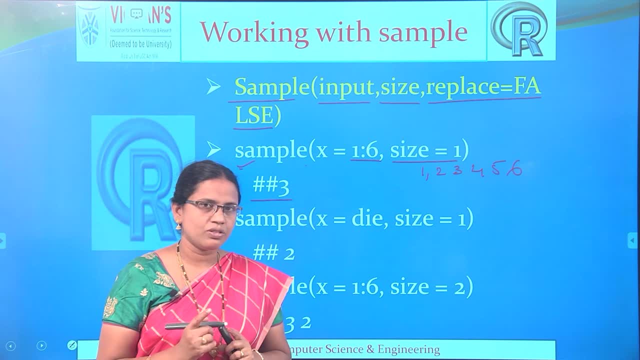 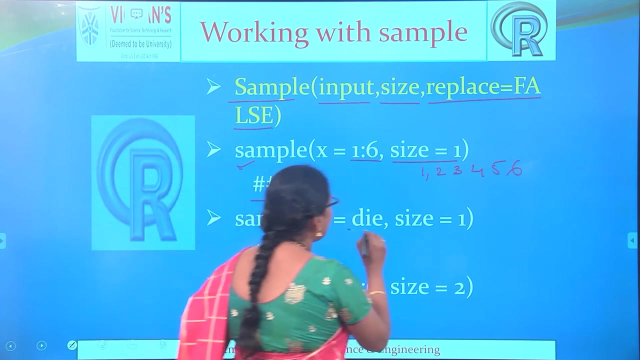 set of the input by making use of the sample function. ok, So try to remember: if you want one number, then specify the size as 1, if you want other number, specify the size as the required number. ok, So I have executed the same command. So now x is equal to die. So here my die input. 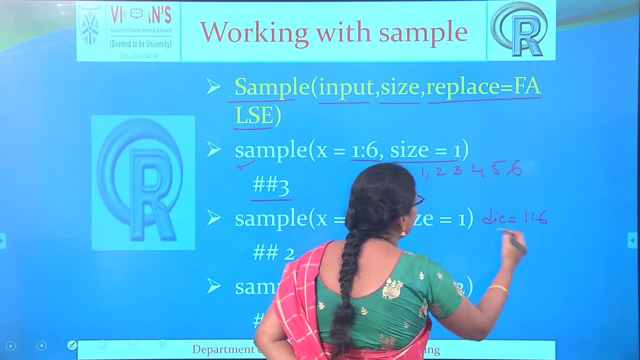 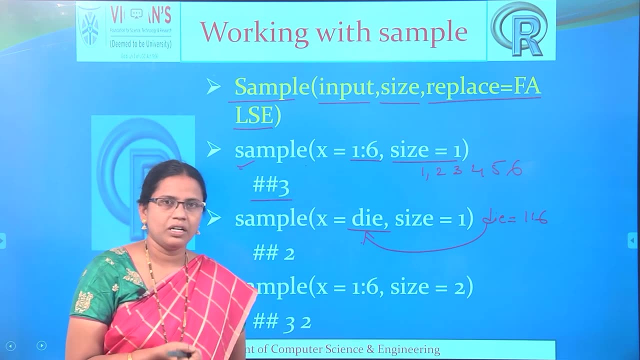 is same. So die is equal to 1 colon 6 and I have passed this die as input. ok, So x is equal to die. So die, die is nothing but one variable. It has the data, that is, 1 colon 6,. 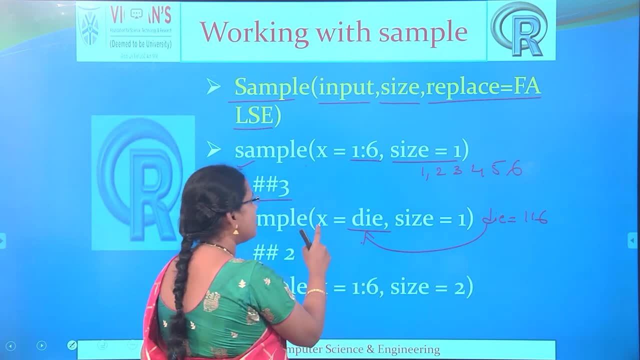 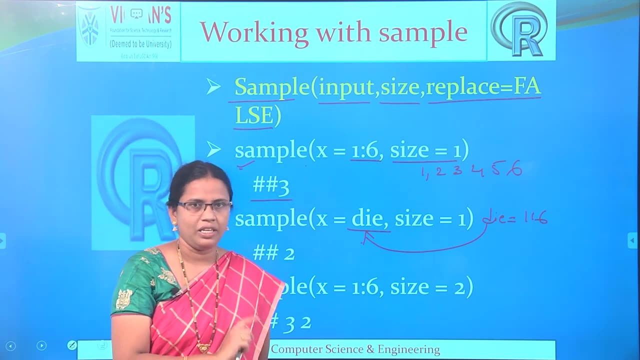 ok, So die is equal to 1, colon 6, and if you pass that die to the x input, then you are going to extract the. you are going to give the input to the x. ok, So when you execute this command, 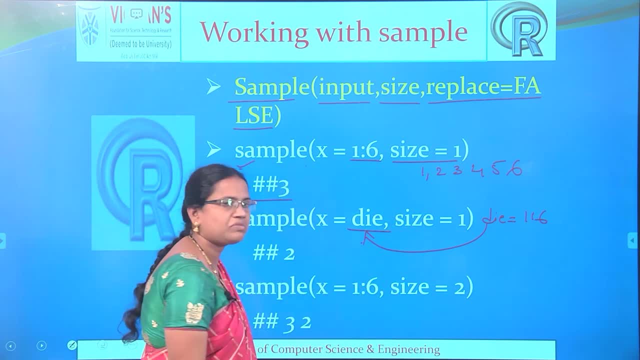 sample of x is equal to die and size is equal to 1.. You can also give the input like this: ok, So when you execute the same command, ok so you will have different output. ok, So next, if I want to see two numbers, 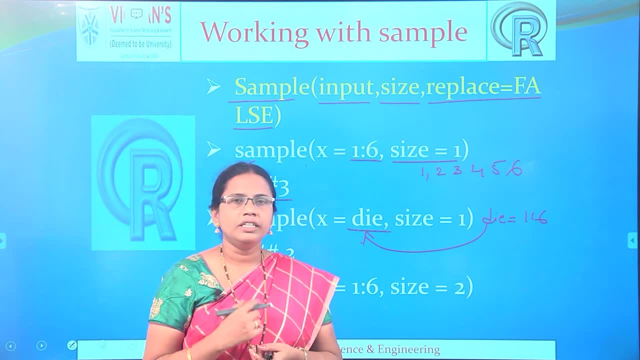 if you want to extract two numbers from the given set of the data, then at that case, ok, so size is equal to 2, ok. If you want to extract two numbers from the given set of the data, ok, from the given set of the data, then you have to specify the size value as 2.. So 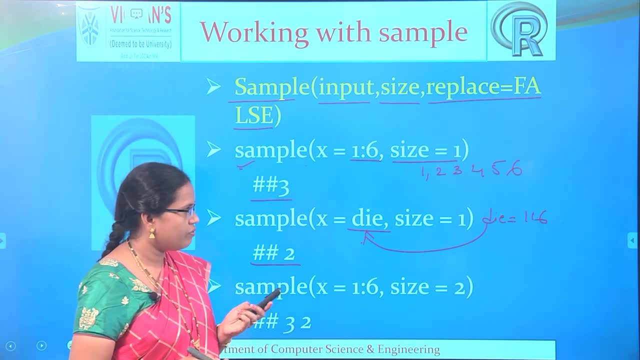 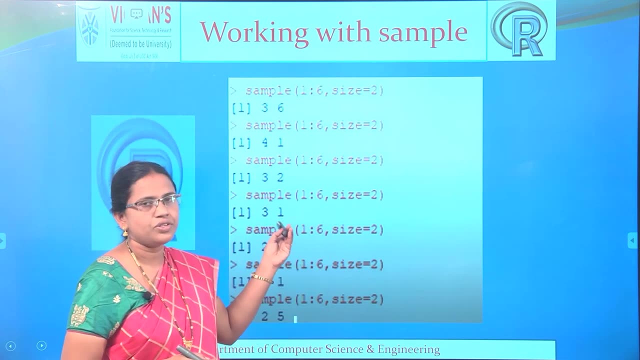 that is 3 comma 2,. ok, So for your, for your understanding, I have executed, ok, so, the same command In my R console and I have given the screenshot here. ok, you can see here sample of 1, colon 6,. 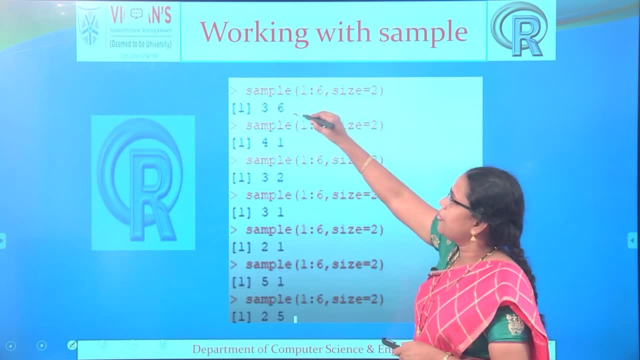 size is equal to 2.. So what is the first input? ok, So by using that command, you are going to extract two numbers, ok, from the given set of the sample, from the given set of the numbers, 1, colon 6.. So the first output, or the first sample that we obtained, is 3, 6.. The next sample: 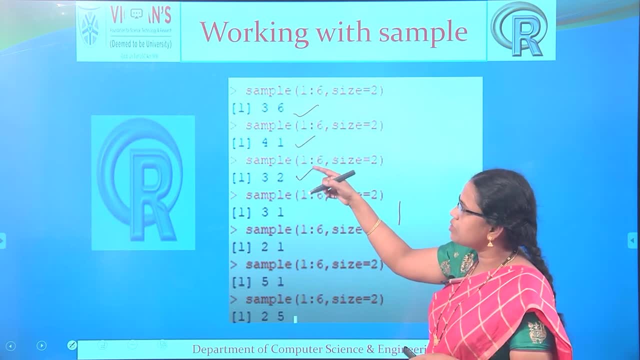 is 4: 1.. The next sample is 3: 2.. Just, I have executed all those one by one, ok. The next sample is 3: 1.. The next sample is 2: 1.. The next sample is 5: 1.. 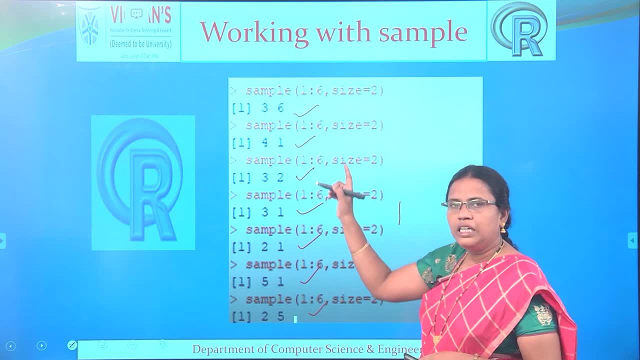 The next sample is 2, 5.. So any sample is repeated here. So nothing is repeated here. ok, So we have extracted and then we have performed some operation on that. ok, So we will extract and then we will. 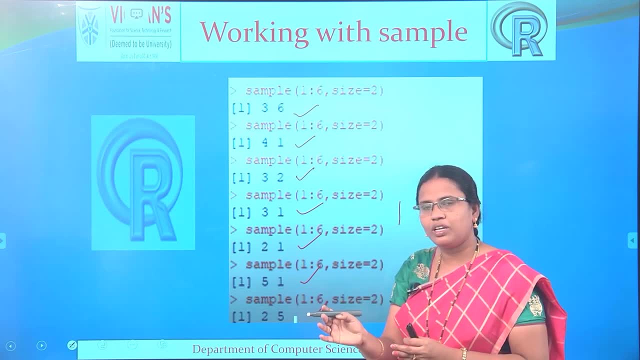 perform some operations on that. And if you want to include, ok, the same set of the sample to the data, ok, then you have to write: The replace is equal to true, ok, So by using the sample, ok, So by using the sample, you are. 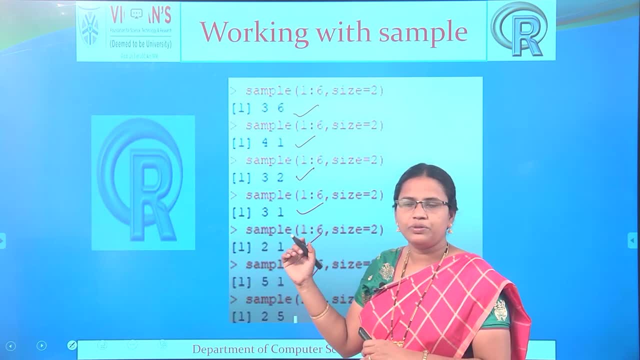 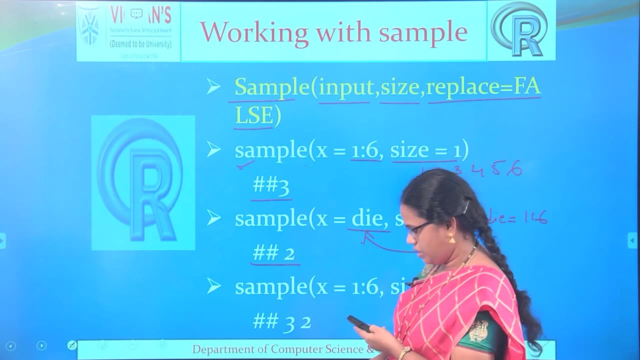 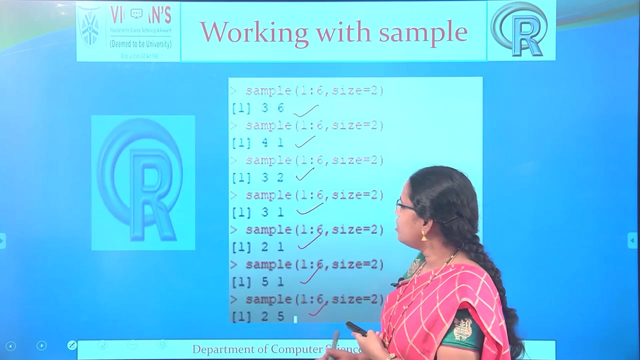 going to extract the numbers, the required numbers, or you are going to extract the required set of the samples by using the sample functions And next let us see: ok, So next let us see sample with replacement I want to in the previous. ok, So none of the sample elements. 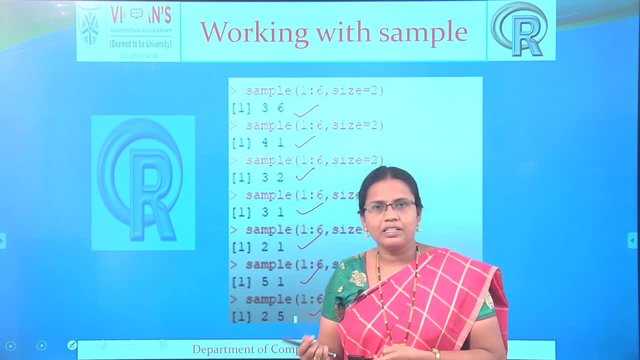 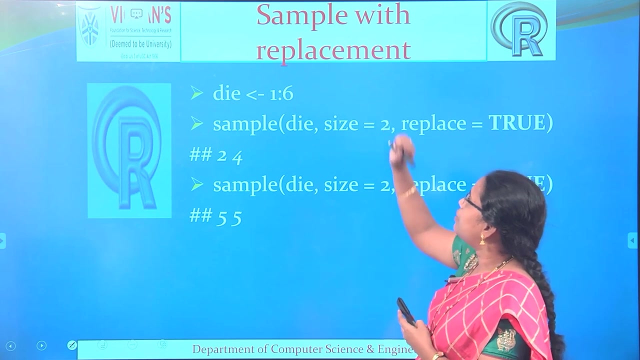 are repeated, But I want to repeat the. I want to repeat the same set of the samples to the next iteration. Then I have to write the replace value as true. I have to write the replace value as true. ok, So now let us see sample with: 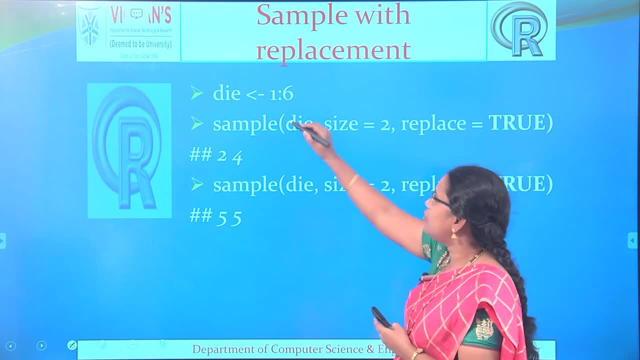 replacement. Sample with replacement: ok, So this is my input. die is equal to 1, colon 6.. And I am going to pass this die. ok, So to the sample function. So sample of die: comma And size is equal to 2.. So I am going to. 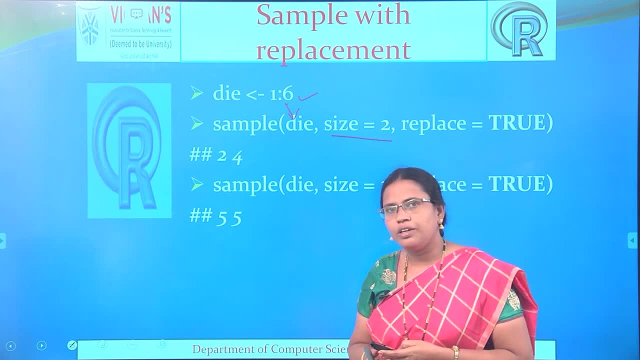 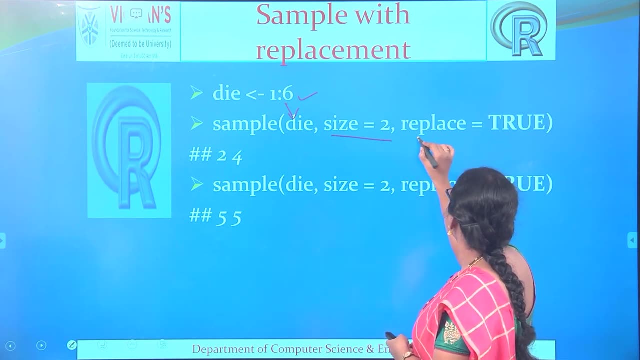 extract 2 numbers. ok, So size is equal to 2.. That means I am going to extract 2 numbers And then replacement is equal to true. So replace is equal to true. That means I am going to place the selected. 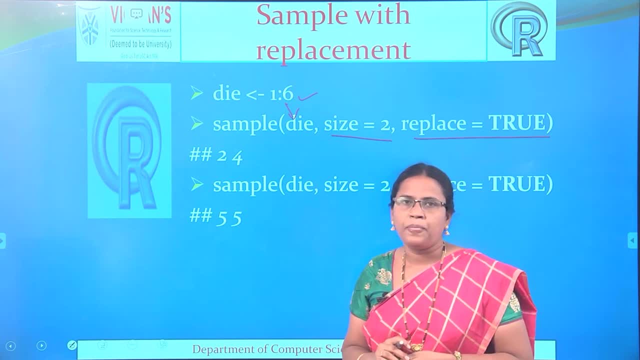 sample to the data set. ok, So once again. So replace is equal to true means, whatever the data is selected. ok, So that is going to be placed to the given data. ok, And then if I execute the command I got: 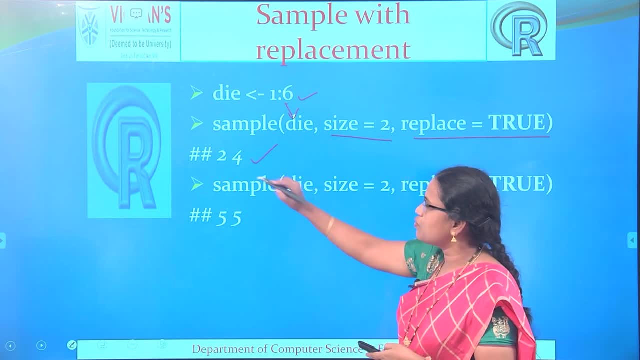 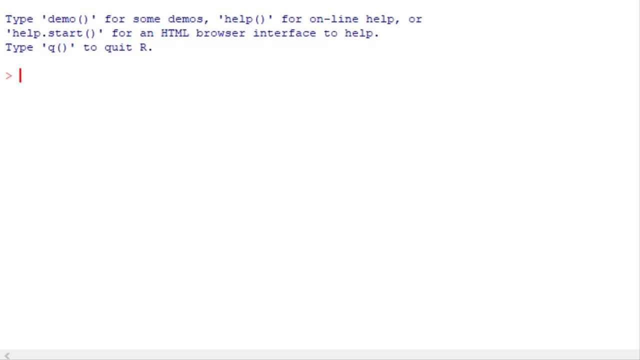 I got the values. I got the samples as 2 comma 4 and when I executed the same command, I got the value as 5 comma 5.. For your understanding, I am going to execute the sample function in R console. This is my R console and now I am going to execute the sample function. So sample of we need to take. 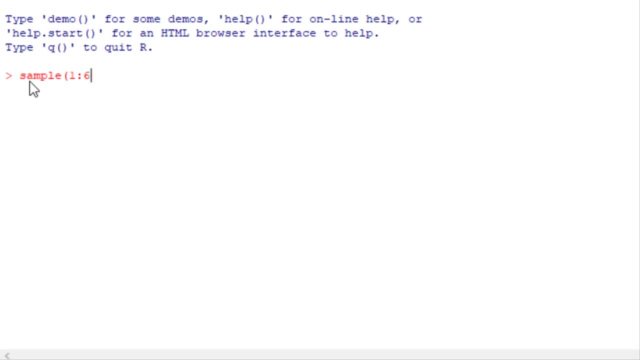 the sample and then after this we need to pass the input. I am going to pass 6 numbers, okay, as input, and after that I am going to extract. I require 2 numbers to extract as a sample. So we need to specify the size as true, and first let us see what is the use with the false. okay, So, 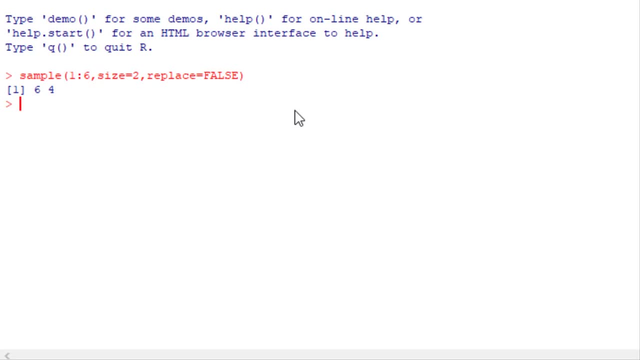 replace is equal to false. You can observe that I will execute the same command one by one. okay, So the first sample is 6: 4 and the second sample is 2: 5.. The third sample is 4- 5.. Fourth sample is: 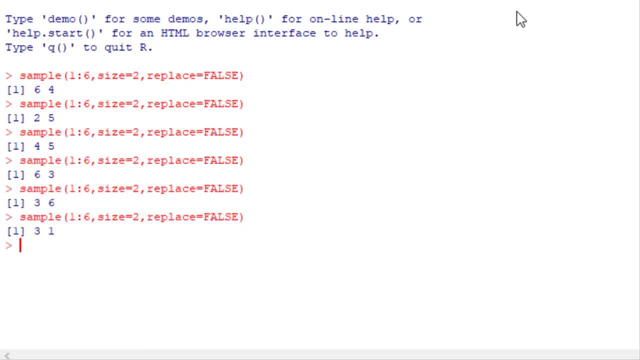 6, 5 and the fourth sample is 4, 5.. So I am going to execute the same command one by one, okay, So the first sample is 6: 3.. The next sample is 3: 6.. The next sample is 3: 1.. The next sample is 6: 1.. The 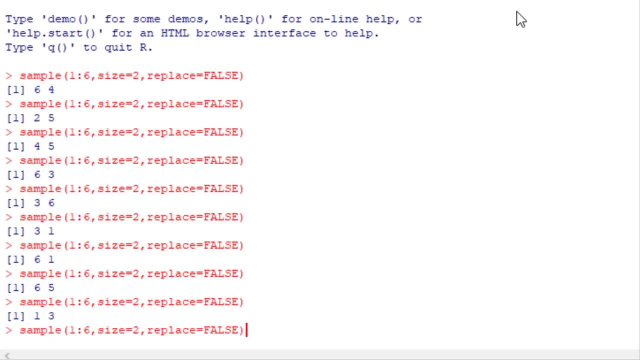 next sample is 6, 5. The next sample is 1, 3. The next sample is 3, 6 and then next sample is 4, 3.. You can observe here we have extracted 2 numbers from the given sample and observe that the first 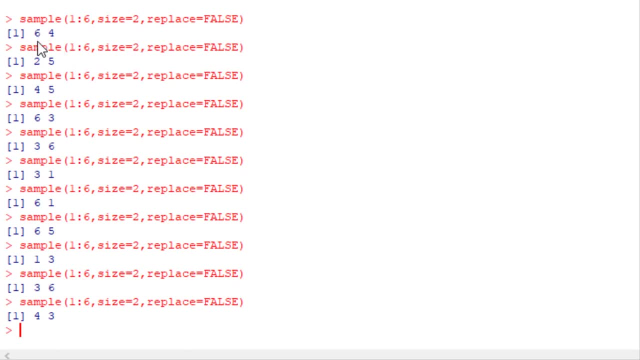 element as well as the second element. okay, So the first element, whatever is selected from the jar, that is not going to be repeated for the next time. okay, So you can observe here: the first sample is 6, 4.. The second sample is 2, 5.. The next one is 4, 5.. Next one is 6, 3.. Next one is 3, 6. Next one is: 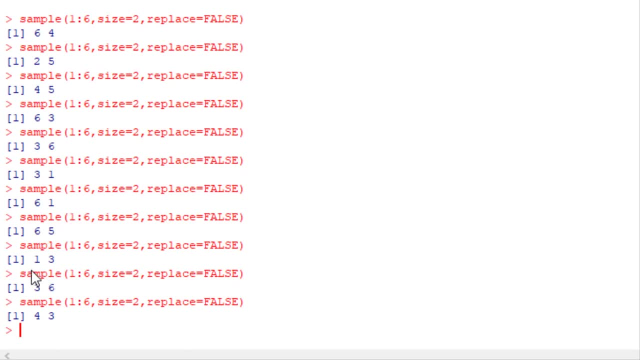 3, 1. Next one is 6, 1. Next one is 6, 5. Next one is 1, 3. 3, 6, 4, 3.. So, when you observe the samples, when you observe the samples, okay, So you can. 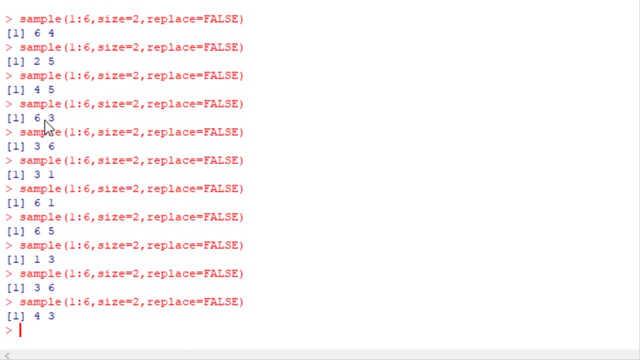 you can tell that the first element, whatever is selected from the, from the input, that is not going to be repeated for the next time. okay, So to have a repeated numbers? okay, So at that case you can make use of the. replace is equal to true statement. Now I am going to execute: replace is equal to true. 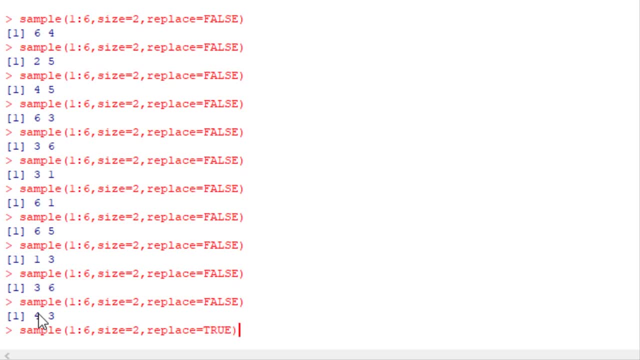 okay, and then I am going to execute it. The first input is 2- 3 and the second input is 2- 1 and the put is 2- 2. you can observe here. so the first element is 2 and also the next element is 2. 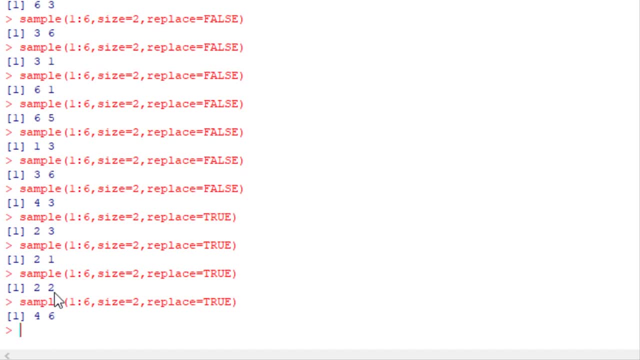 so elements are repeated here. okay, so to have a sequence, okay, so to have a repeated numbers. okay, so at that case you can select: replace is equal to 2, so you can observe that the previous, the previous one, is 6, 6, right, so the first element is same, the first, so the first element is 6 and 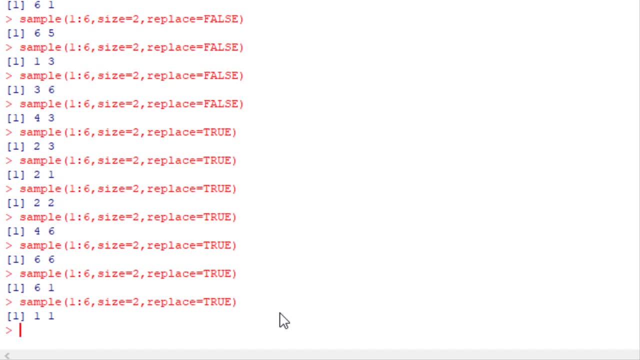 the second element is 6, 6, 1, next one is 1, 1 and the next one is 3, 6, next one is 2, 3 and the next one is 3, 4. so you can observe that 2, 2. so like this, like this, you can work with the. 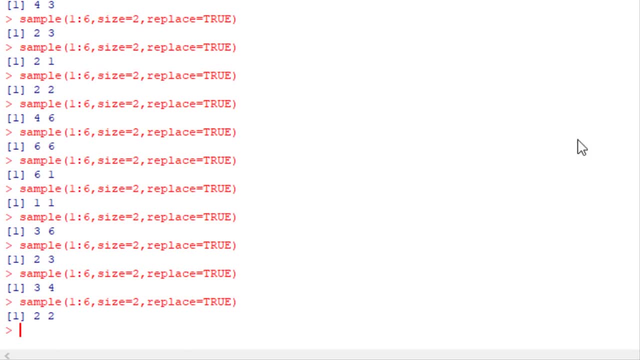 sample function. try to try to understand here. so when you replace, when you place the replace value as false, the first sample that, whatever is selected that is not going to be replaced, to be repeated. and when the replace is equal to true, that means that the first sample that 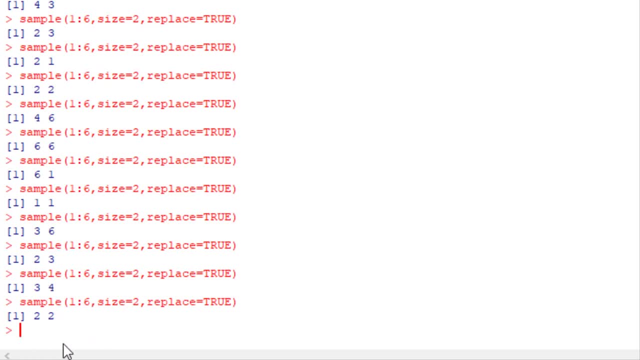 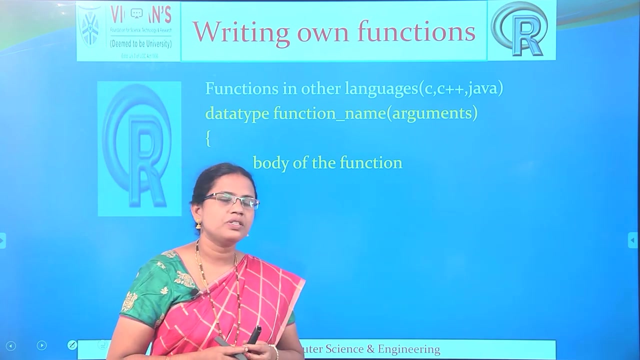 whatever is selected, that is going to be repeated. okay, so to have that sequence of numbers, to have that repeated numbers you can make use of, the replace is equal to true. now let us see how to create our own functions with our programming language. okay, i have given. 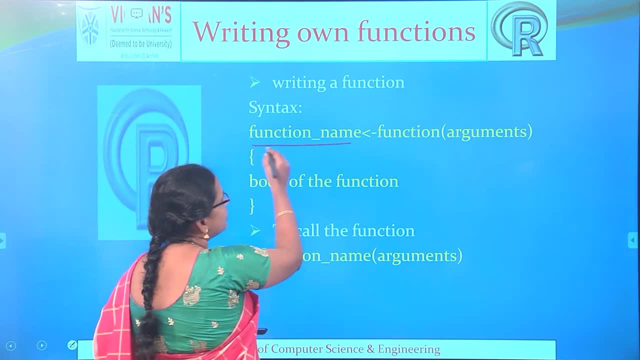 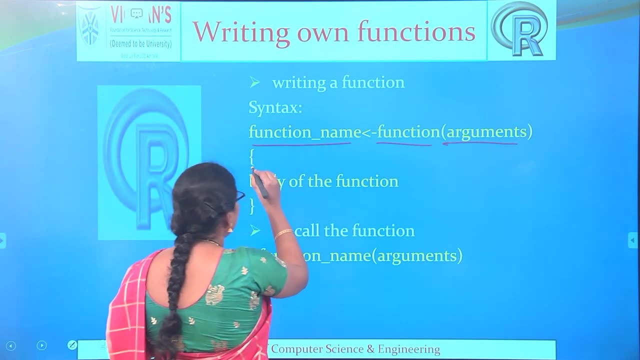 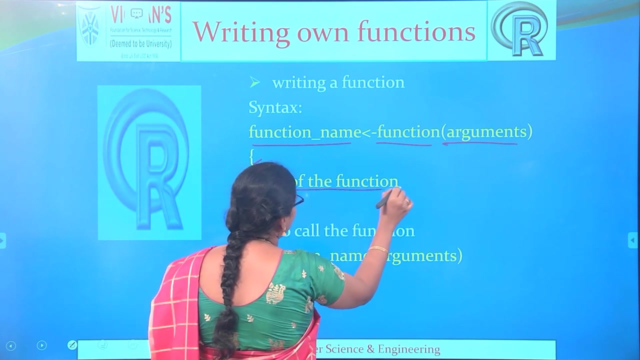 the function here in our programming language, see this- one function name is equal to. so this is your function. your function will starts here, function of arguments, and then you will write open and closed curly braces within this: closed, curly, closed, curly braces. okay, so you will write the body of the function and then now how to call this function? okay, so. 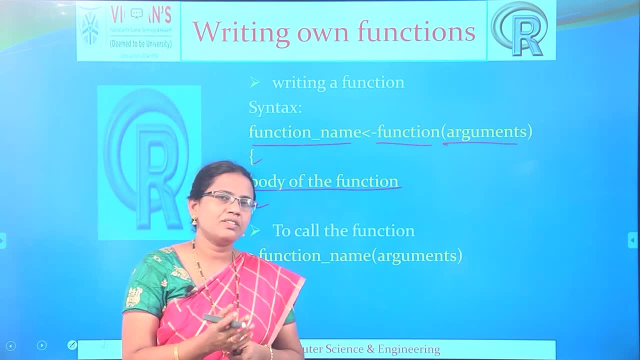 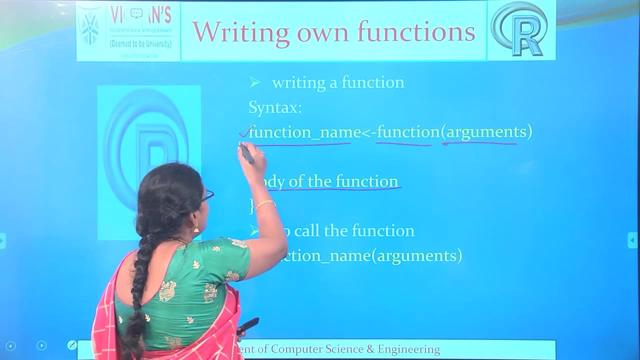 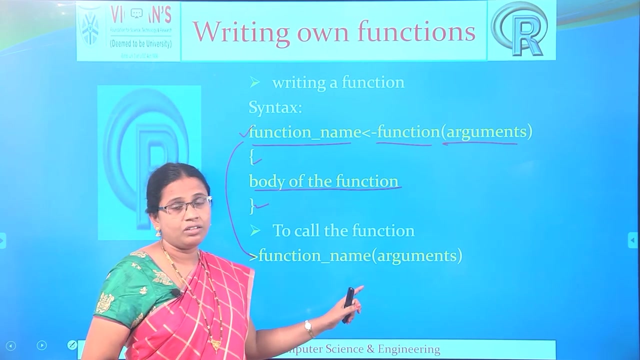 you will call the function in other programming languages also by specifying the function name. here also you will make use of the function name, that whatever you have given here, okay, so that. whatever you have given here, so function name when you execute the function name. okay, so your. 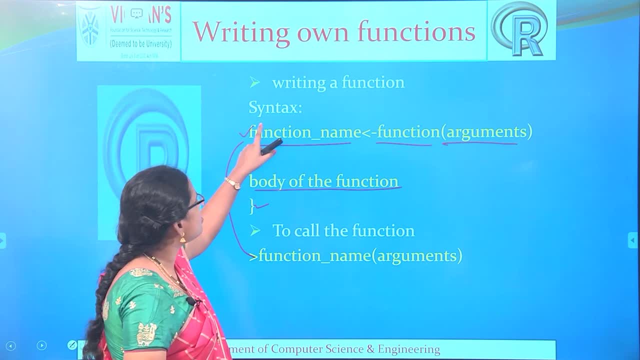 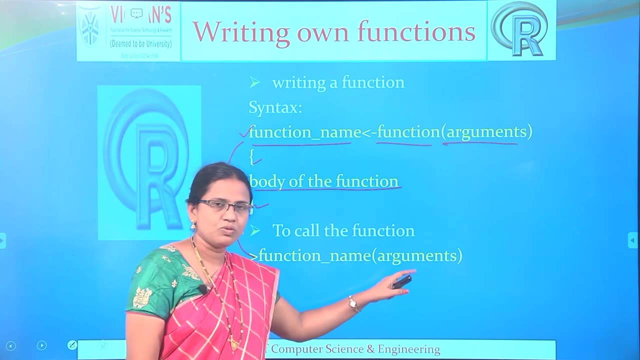 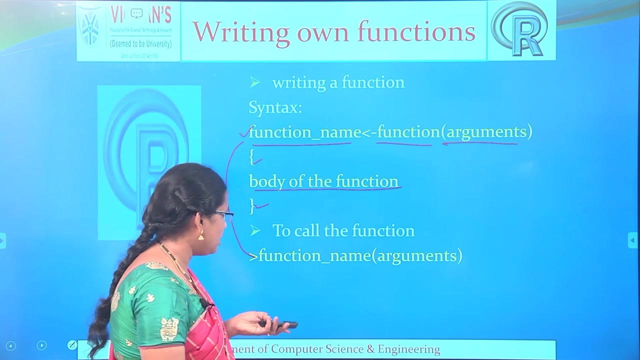 function is going to be executed. okay, so this is the syntax for creating the function and this is the syntax for calling the function. okay so. function. name of arguments: if you specified any arguments for the created function, then you need to specify. otherwise you need not specify. okay, so next let us see some examples for writing a, for writing our own functions, okay. 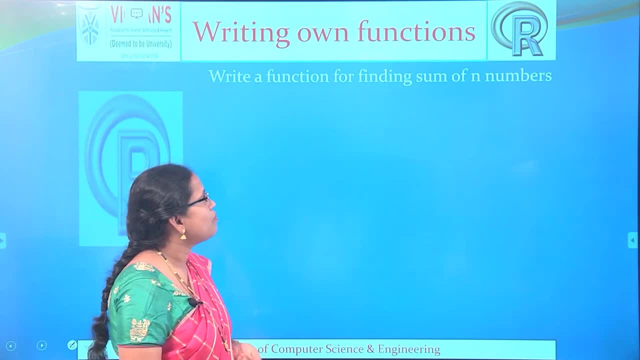 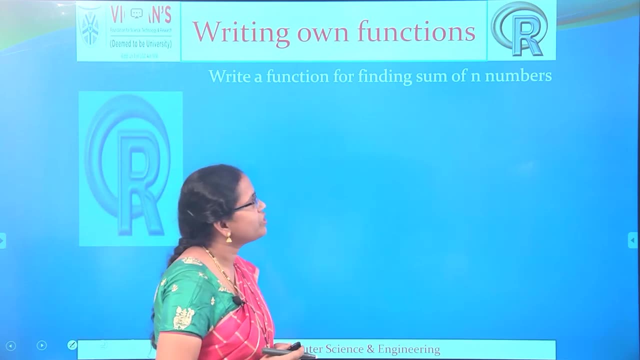 see this one. this is the question. so write a function for finding sum of n numbers. okay, so for finding sum of n numbers. so for this, okay, let us see how to write a function. okay, so i am going to make use of. our task is to find the sum of given n numbers, or sum of 1 to 10 numbers. okay, so we. 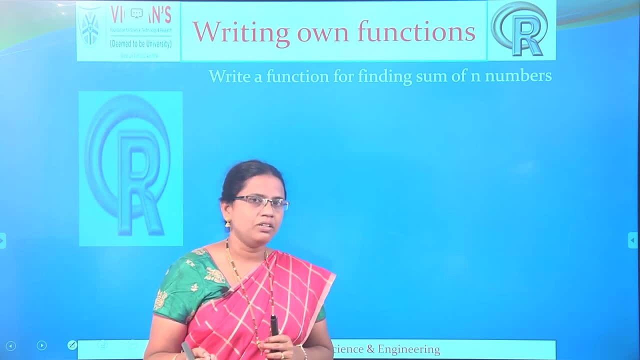 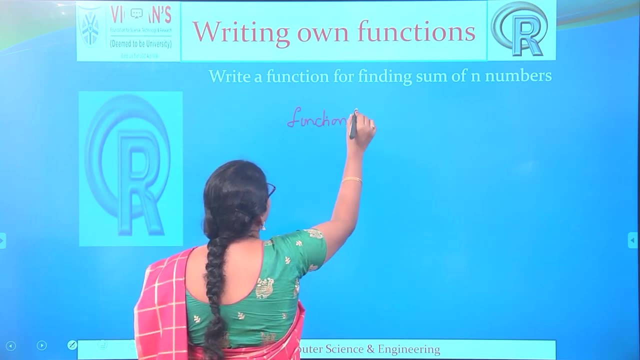 need to, i am going to make use of the sum function, which is already available. okay, so for that, i am going to write the function, so function. okay, so, to write a function, you just write function and i am not going to pass any arguments. okay, so for this, for for the 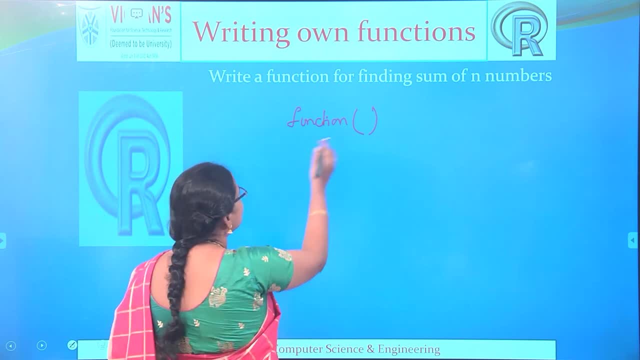 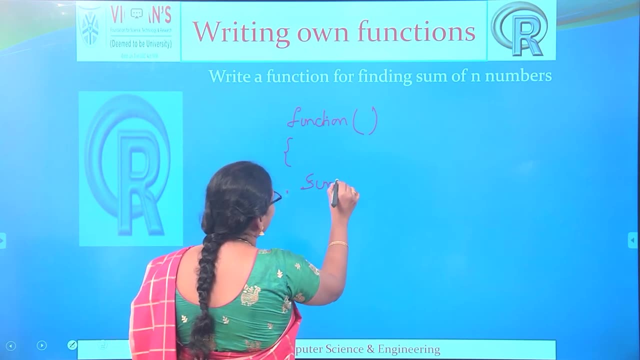 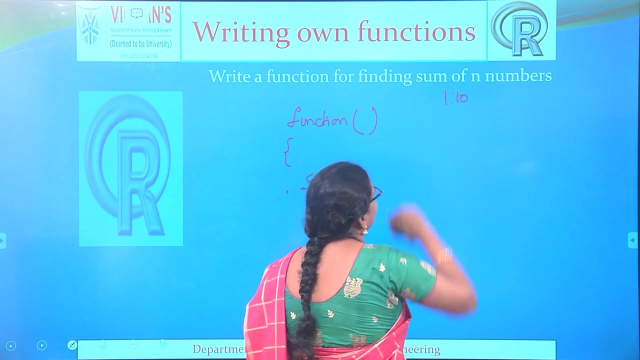 basic understanding. i am not going to pass any arguments, so function. okay. i am going to open the closed braces. okay, so i am going to make use of the sum. okay, so sum of if. if i want to find the sum of numbers from 1 to 10, okay, so then just give the command sum of 1, colon 10. 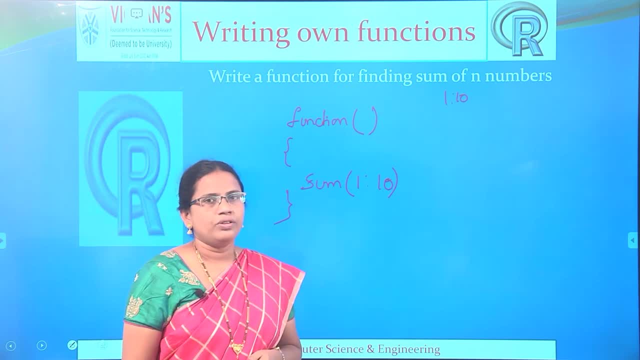 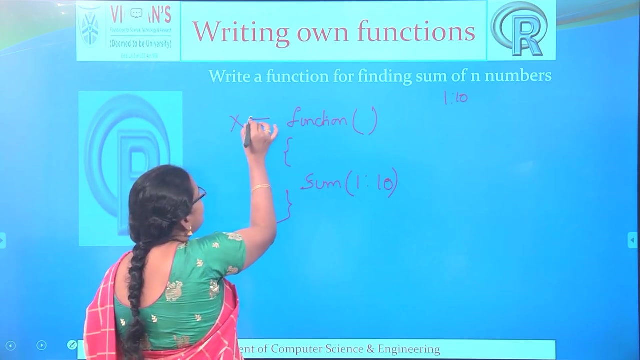 and then close this function. okay, so function. this is created. the function is okay. writing of the function: writing the function for a given task is completed. next you need to store this function in one variable. so i am going to store this function in one variable, so that let the function. 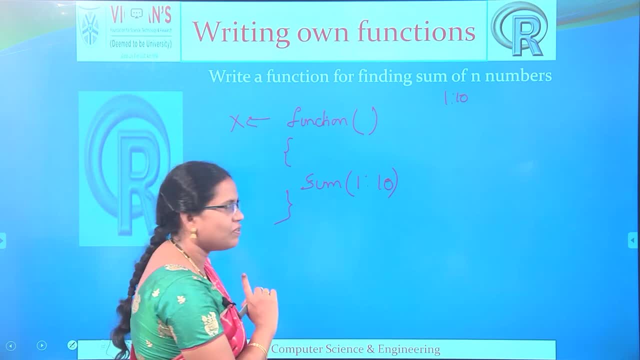 name is now it is x. okay, so if you want to call this function, if you want to execute this function, then one what you need to give. so just write the function name. what is the function name? function name is x, and then any arguments passed here. so no arguments passed here, so just you need. 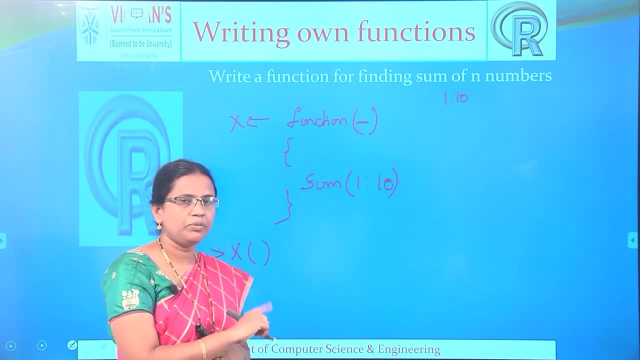 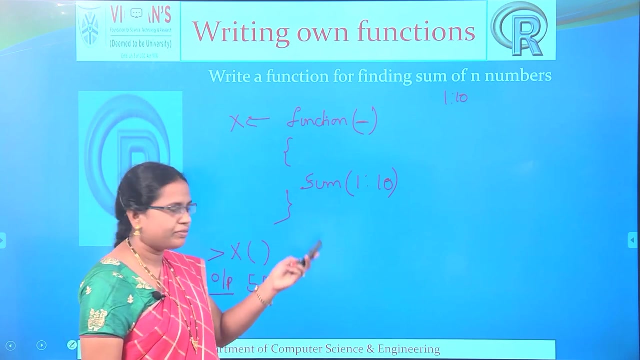 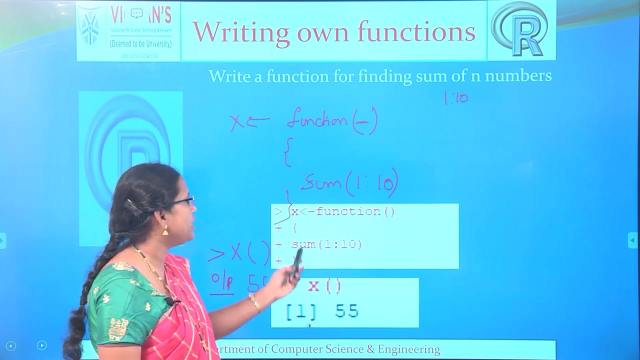 to write the empty, empty parenthesis. okay, so when you execute this, you will have the output here. so what is the sum of n numbers? that is 55. okay, so next let us see. okay, so, for your understanding, i have given the screenshot for you. okay so, so see this one i have created. the function x is equal to function of. i have not passed any. 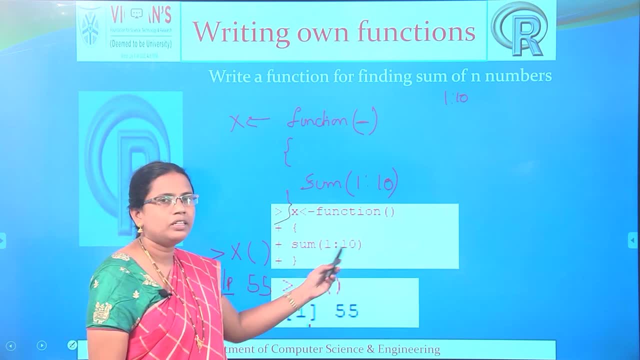 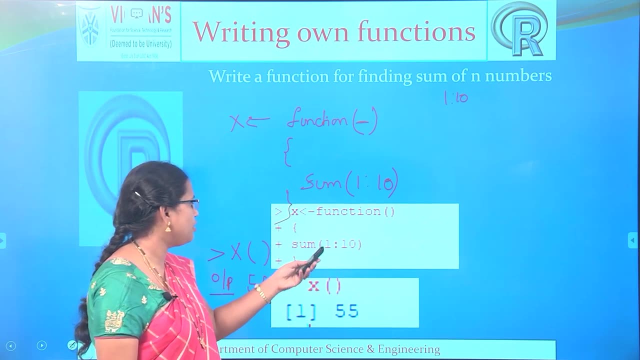 parameters here, and then sum of 1, colon, 10. okay, you need to execute like this in your r console: okay, so, x of. okay, so this is the function. and to call this function you have to write x, open and closed parenthesis, and when you execute this you will have the output like this: okay, so next let 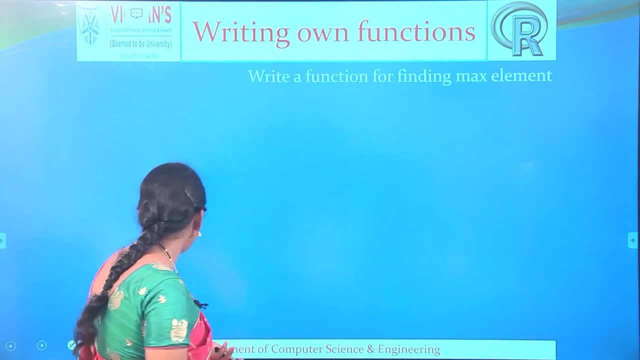 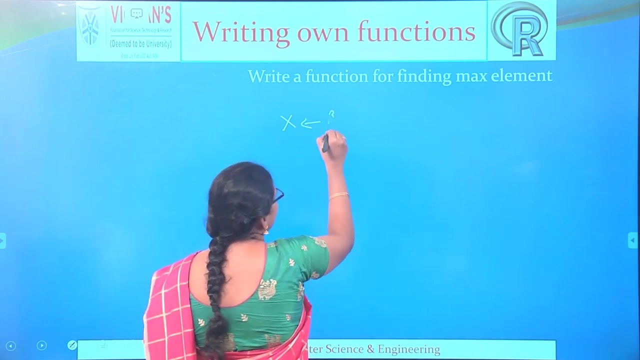 us see. so next, let us see other example. so write a function for finding maximum element. okay, so for a given set of numbers you need to find out the maximum element. okay, let us write the function here. so i am going to write my function. name is x. okay, so x. x is equal to. so what is the thing that you have to write first? so x is equal. 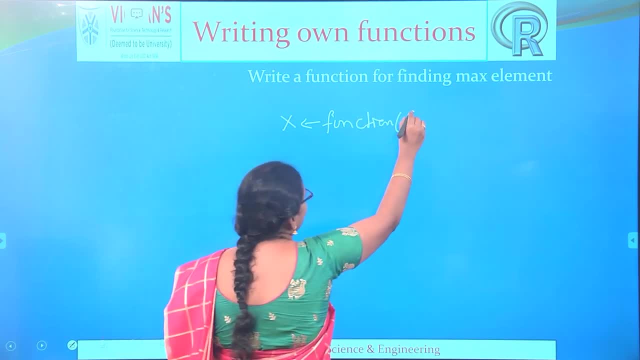 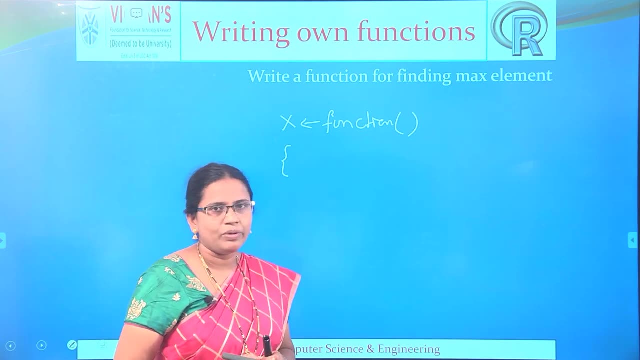 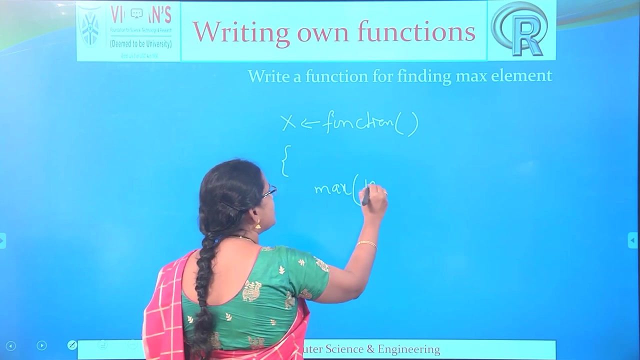 to function of okay, so i am not going to pass any parameters here. function of okay, so just open the and then our task is finding the maximum element. so i am going to make use of the max function. so max of okay, so i am going to pass the input here. so i am just writing some random number. i am going 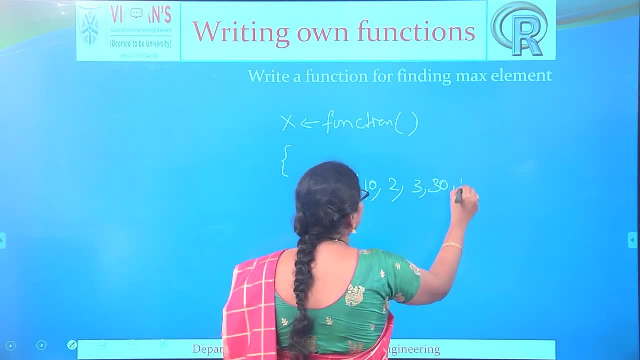 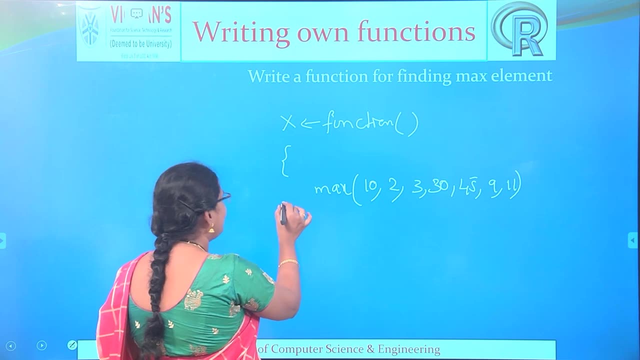 to write some numbers here. okay, like this, i am going to close the function. okay, so this is the function that is creating the maximum element. okay, so i am going to write the maximum element for finding the maximum element for a given set of the elements. okay, so to call this function. okay. 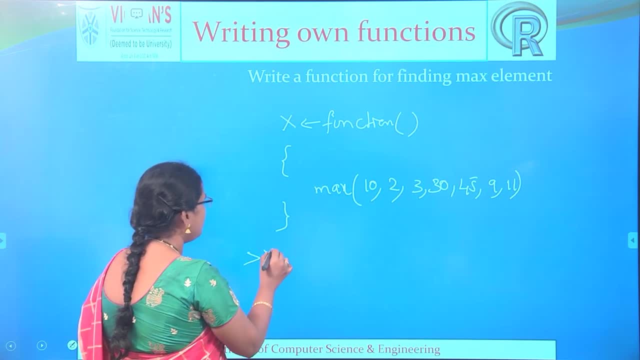 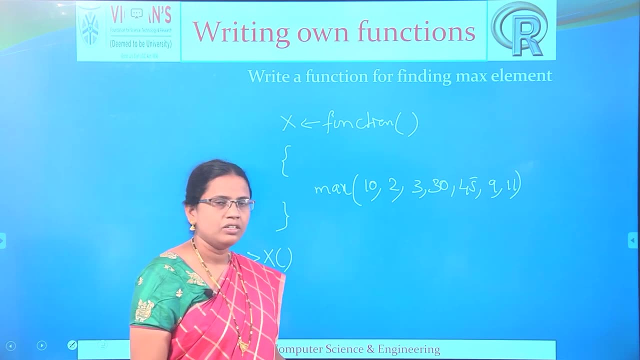 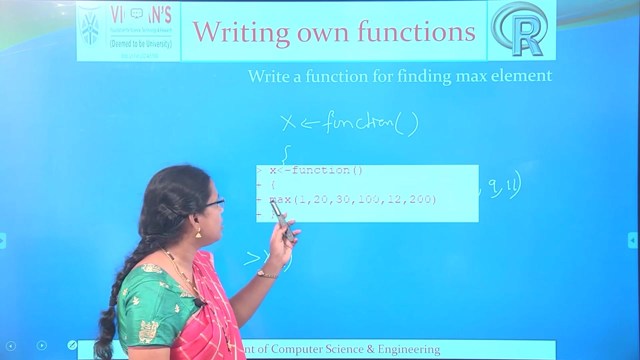 so to call this function, what is the command that you have to give? so x. okay, so the function name is x, just call this function. okay, so let us see it. i have given the screenshot here. so this is the function that i have created. so x function. so max of this is the input that i have given, okay, and 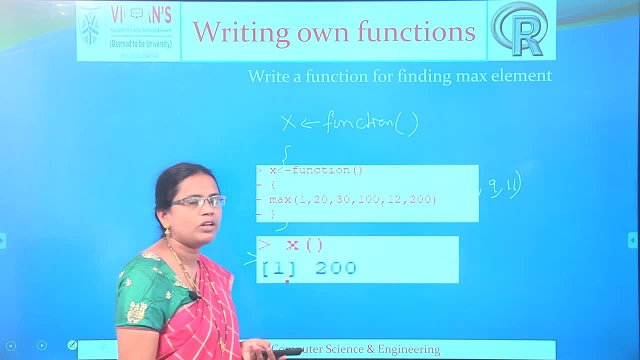 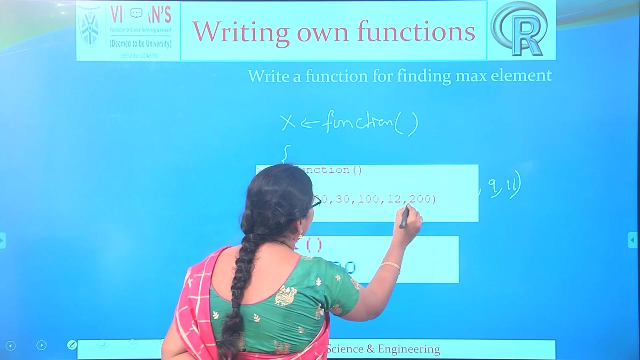 then next: okay, so this is the calling of the function. so what is the maximum element for a given set of the elements? so this is 100. okay, the maximum element for a given set of the elements is so 120, 30, 100 and then 200. so the max element for a given function is 200. 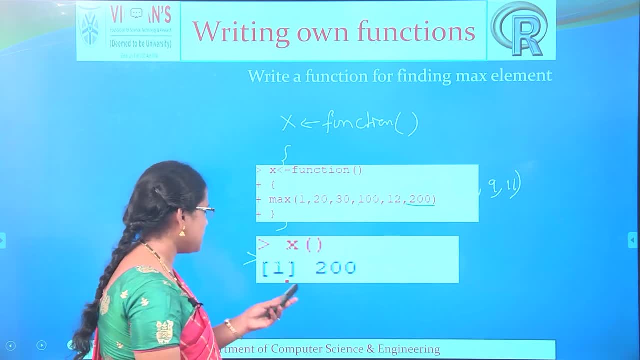 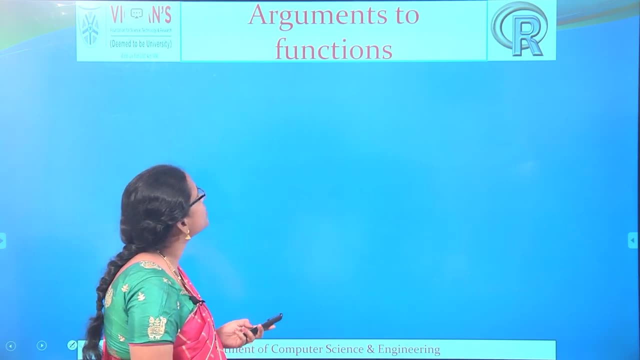 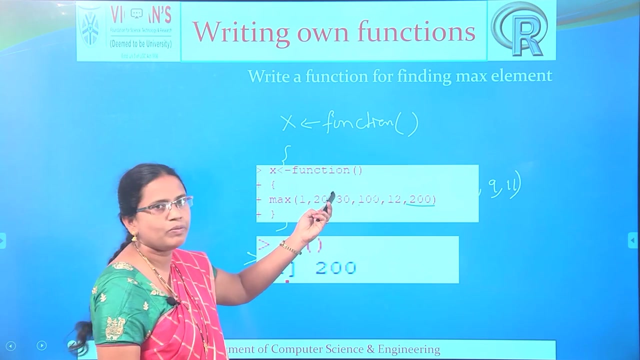 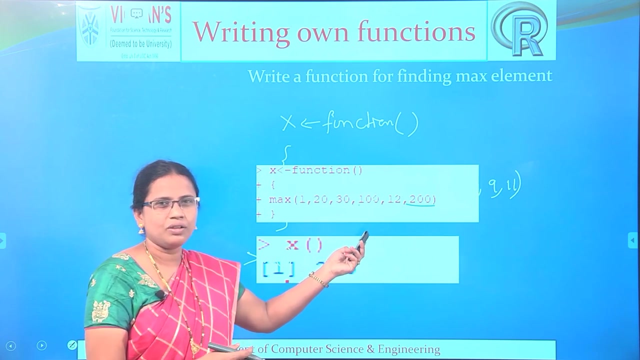 okay, so next, let us see other tasks. so next, let us see other tasks. so arguments to the functions. okay, so previously we have seen: okay, so we have created a function here for finding the maximum elements. we have not passed any parameters here. okay, so there is some disadvantage, okay, if you are not working with the arguments. okay, that means that. 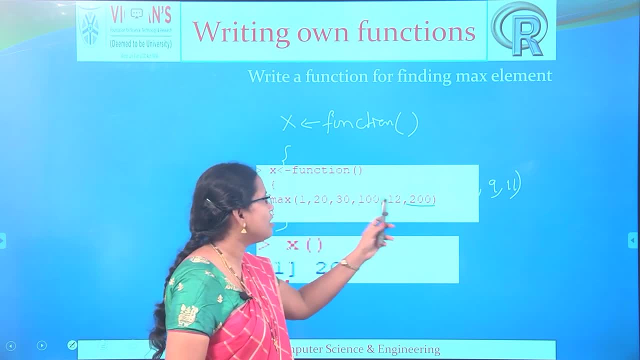 you can. we can find out. you can perform the task only for a given set of the input. if you want to pass the same, if you want to execute the same, you cannot do that, okay, so that you need some set of arguments that you have to pass, okay, so now let us see how to pass the. 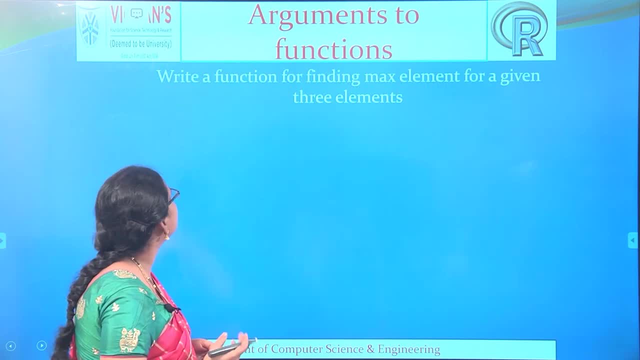 arguments to the functions. okay, so i am. here is a task, so what is the question? write a function for finding maximum element for a given three elements. okay, so our task is: we need to read three numbers. okay, so from that numbers, okay, so we need to find out the maximum element. let us start. 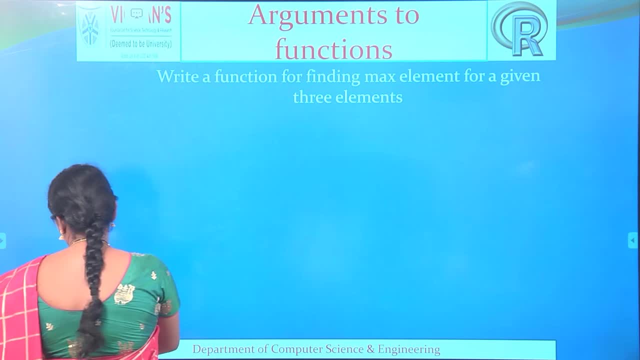 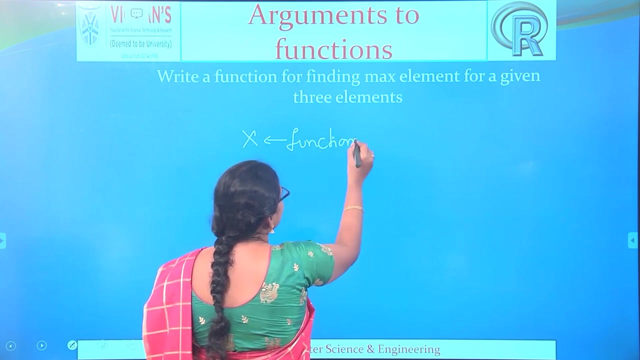 okay, so what is the function name? so i am going to give the function name. okay, so always, i am going to give the function name is x. okay, so let my function name is x and you need to write the function by writing the function function keyword. okay, so, function of. so what are the inputs? how? 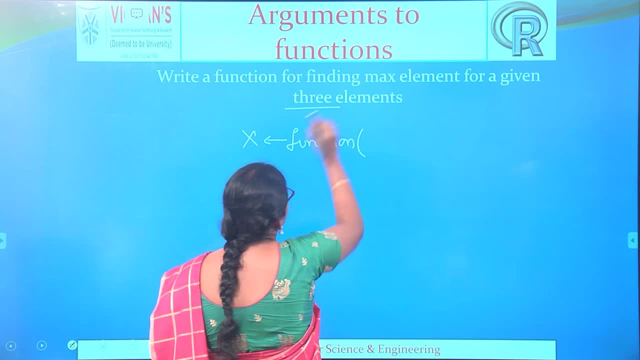 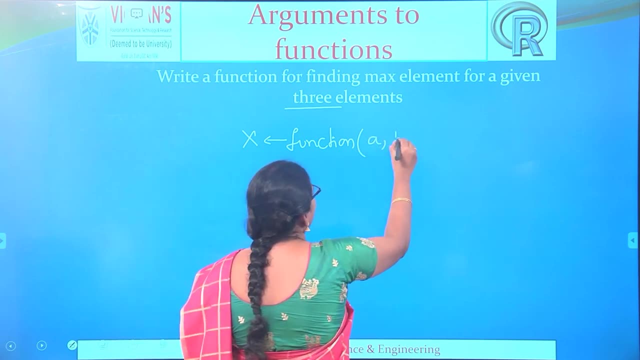 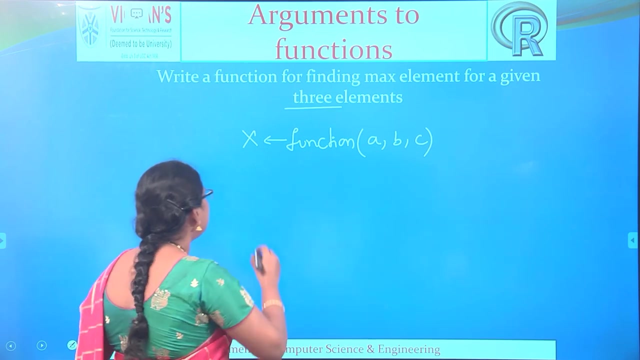 many inputs you required. your inputs required are three. okay, so you required three inputs. so let my input names are a b, c. okay, so a comma b, comma c. i am going to take three inputs because these for the given three elements, and then after that i need to write like this: open and closed. 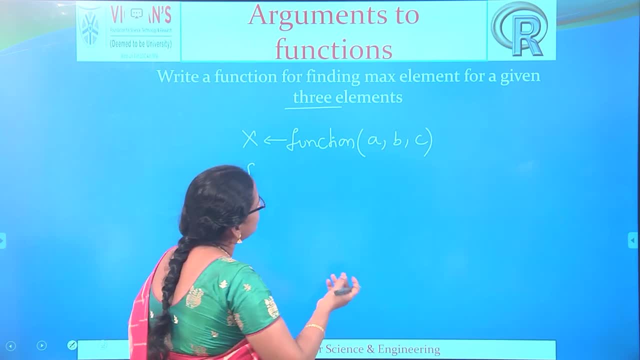 braces. okay, and then my task is finding the maximum element for a given three numbers. so i am going to make use of the max function. so max of. so i need to find out only these three. oh, i need to find out only the max function for these three numbers. so max of a, comma b, comma c. 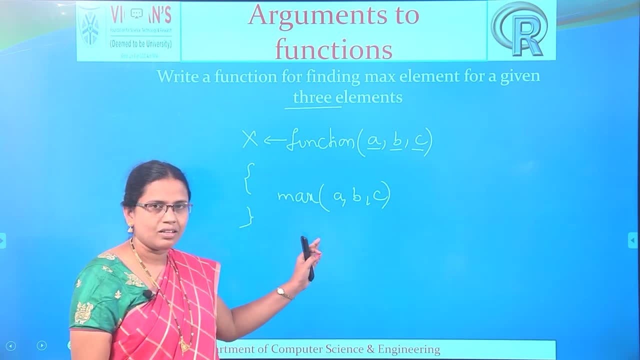 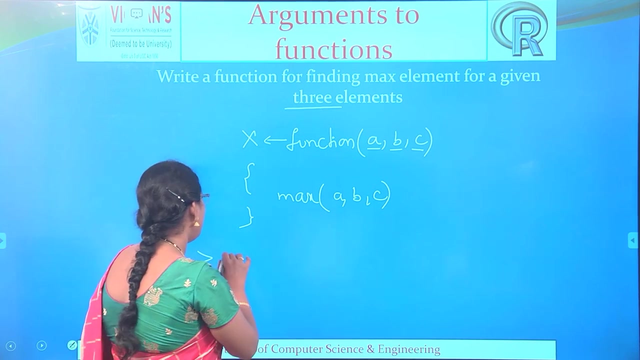 okay, so, task is completed. so, by using these function, you are going to find out the maximum element for a given three inputs. okay, so, and if you want to call this function, then what is the command that you have to give? so x of okay, so how many parameters that you have to pass? how many parameters are? 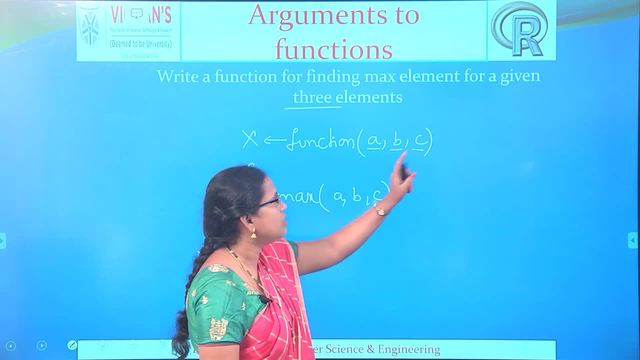 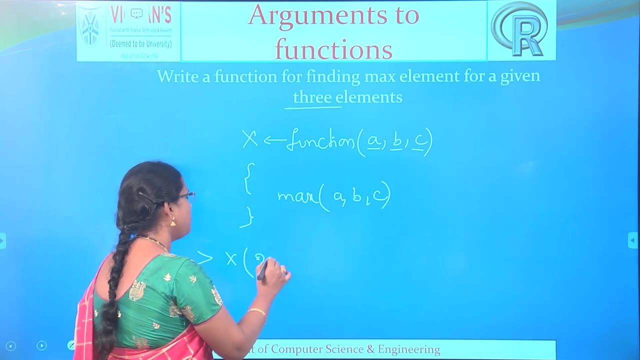 given for the function. three parameters are given: a, b, other one is c, so you have to give the values, three values for the function. okay, so i am going to give 20, 12, other one is some 19. this is my input. okay, so now, when you give this, okay, so a value will be. 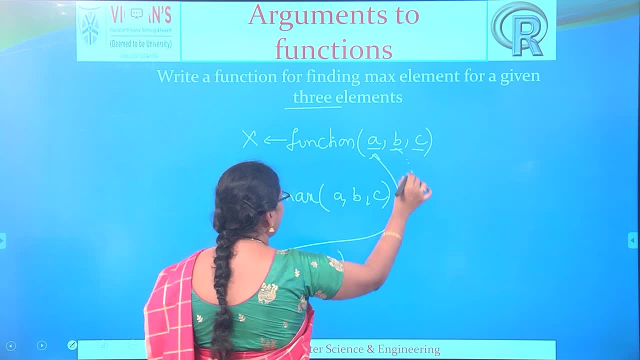 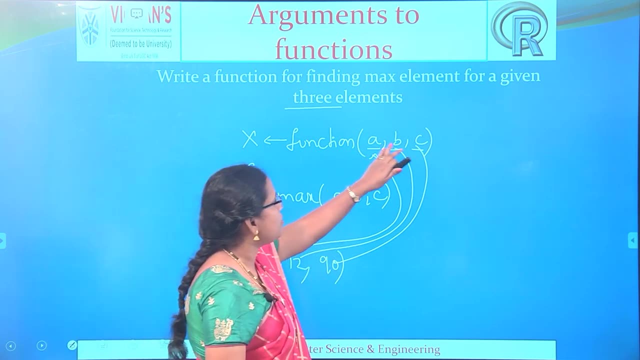 okay, so the 20 will be the a and b value will be 12 and c value will be 19. okay, so this is taking the inputs. a, b, c are the inputs now and these are going to be given for the max function. so max of. 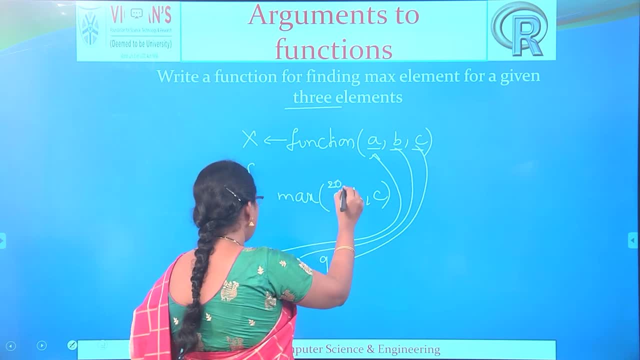 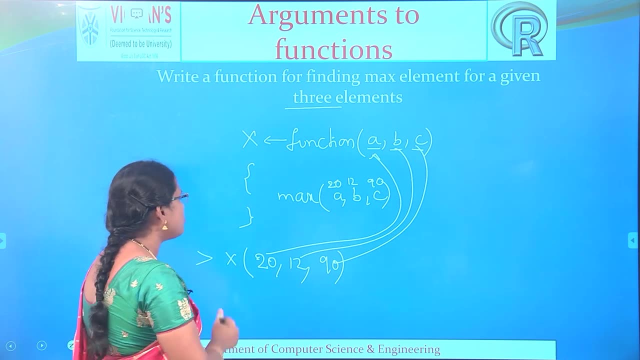 a, b c. now what is max of a, b, c? max of 20, so 20. so this is the input, so this is the input. so this is 12. other one is 19, okay, so what is the max answer? max answer is 90, okay, so next, if you want to, 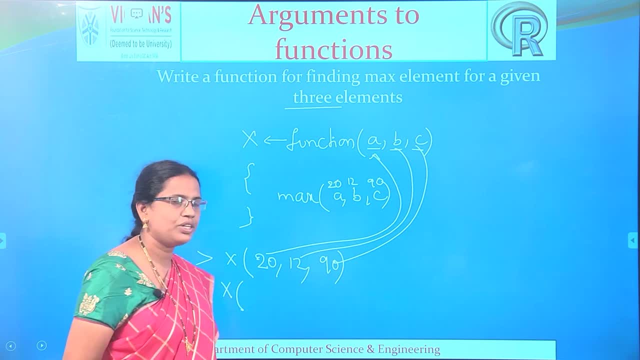 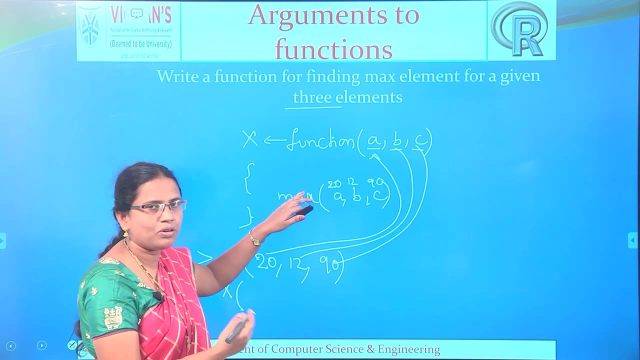 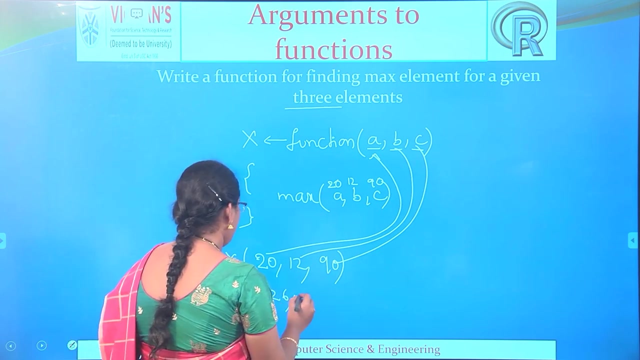 perform the maximum element for other three numbers, then what you need to write? then you need not write the function. that is already created. you can give other input, okay, so just you need to call that function with other inputs. okay, so let my input is 19, 26 and then 9, so this: 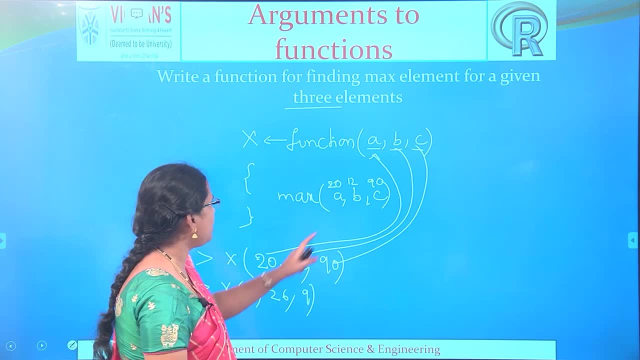 is my input when you execute this. okay, so now a value will be 90, b value will be 26, c value will be 9, and then i am going to pass abc. okay, so max of abc, that is max of 19, 26, 9. you will have the different output. okay, so next for your. 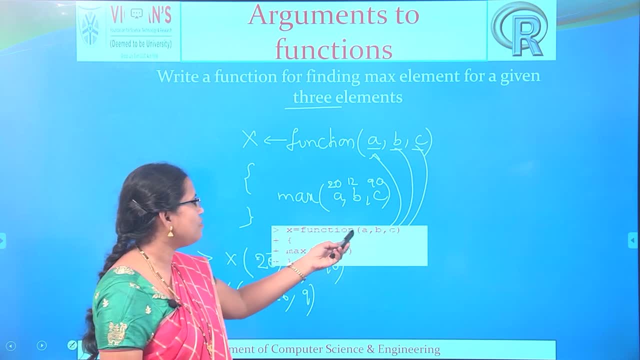 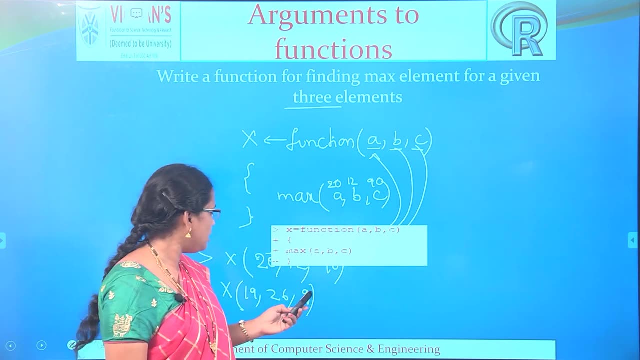 understanding. i have given the input here. so x is equal to function of abc and then max of abc the same. whatever i have written here, i have given as a screenshot and then when you execute this, when you call the function like this, and then you will get the input of the function like this: 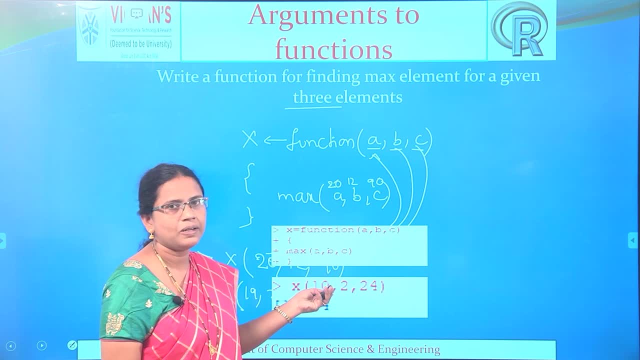 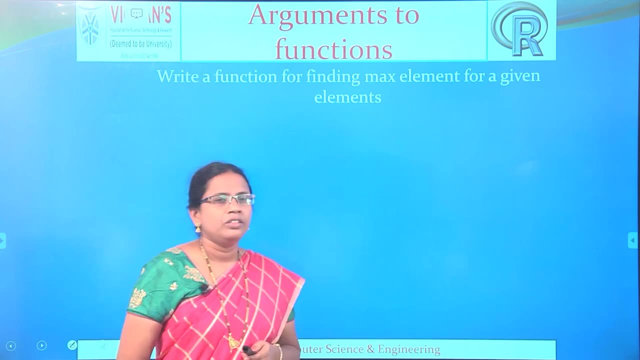 this x of 10 comma, 2 comma 24,. we are going to have the output like this: And then next let us see other example. okay. Next let us see other example, that is, write a function for finding maximum element for a given elements. okay, for a given elements. So in the previous example, 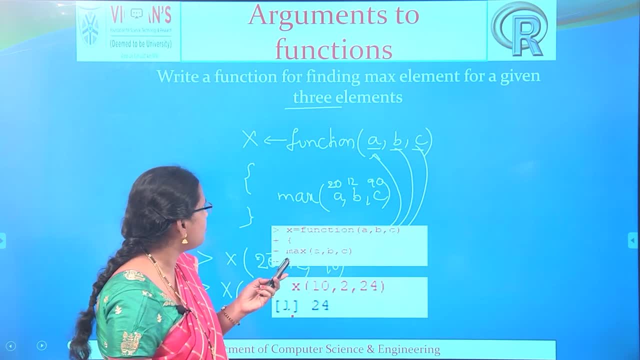 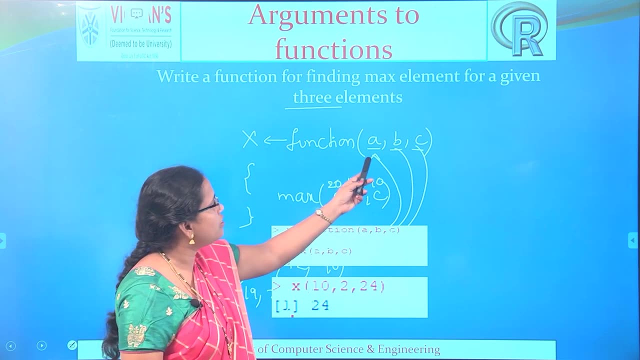 so we have seen previous example, right. So the same question. I have given the same question. Here I have given three elements. okay, So when you have here I have given three elements- If you do not know the size of the input that we are going to give for a function, 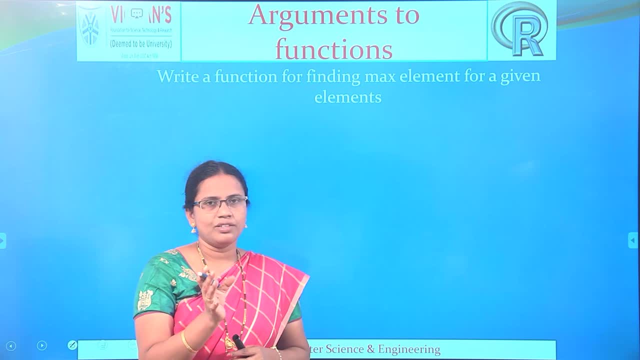 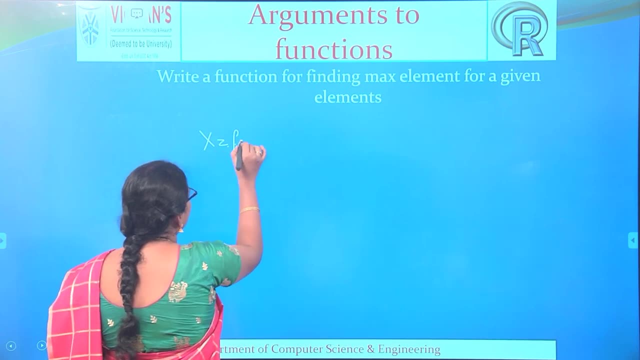 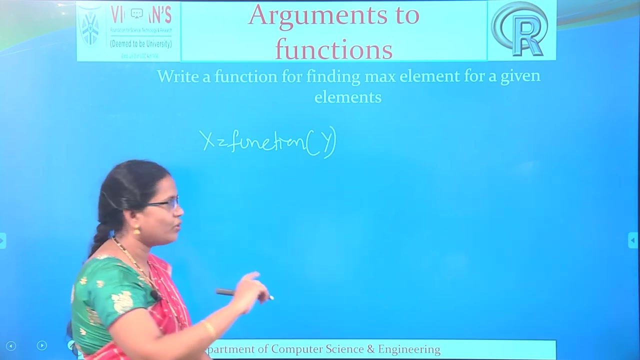 then at that case you need to give the input. okay, At that case you need to give some variable as argument to the function. okay, So let us see it here. So x is equal to function of. okay, So function of y. I am going to make use of this y for the input. 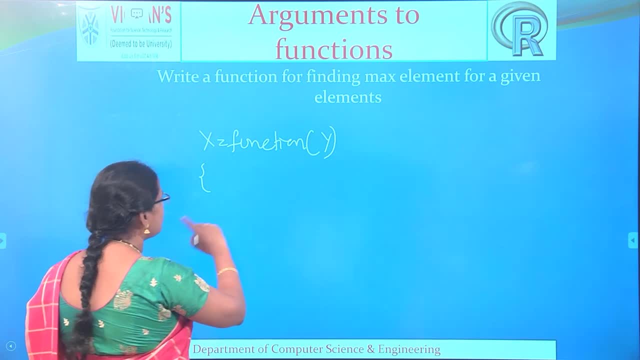 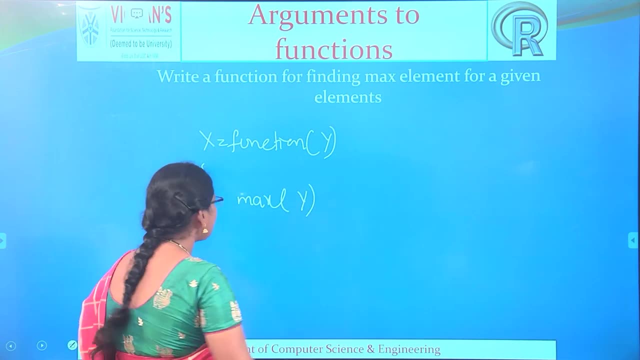 okay, So, and then I am going to open the open trace and then our task is finding the maximum element, So max of okay, So we need to give the max of y And then let us call how to. 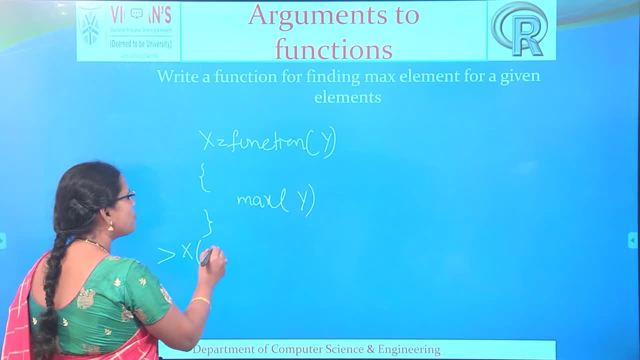 let us see how to call this function x of. okay, So, to pass the multiple values, we need to make use of the c. okay, So this is a function which holds many values. okay, So this is a function. this c is a function which holds many values. okay, So? 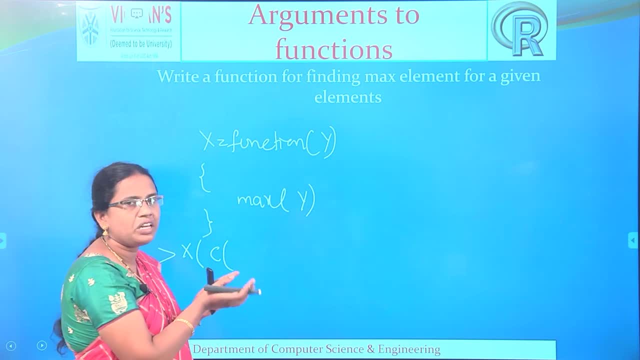 I am going to make make use of this. okay, So, because I am going to pass many values to the function. okay, x, So, x of. let my function name is x, x of c, open parenthesis. okay, So 2,, 4,, 5,. 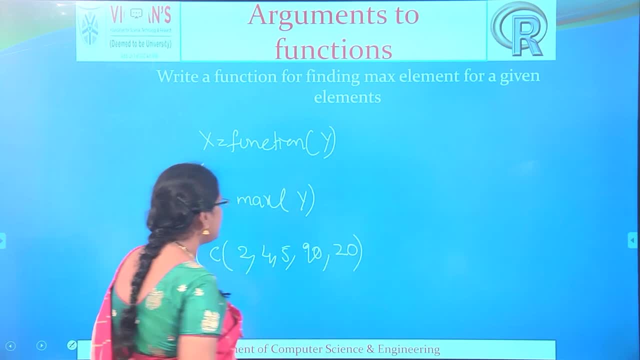 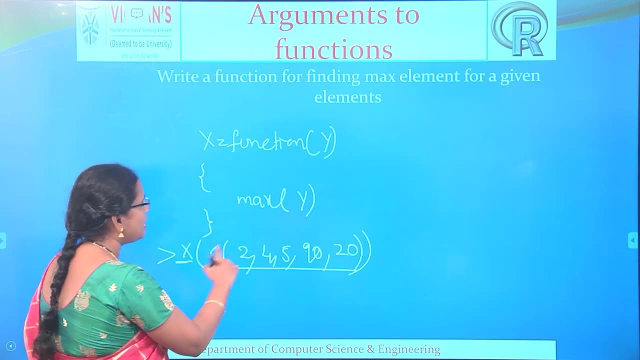 okay, So 90 and then 20.. So this is my input. I need to close this one. So this is my input. And when you execute this command, this entire input will be passed to the y. okay, So when you? 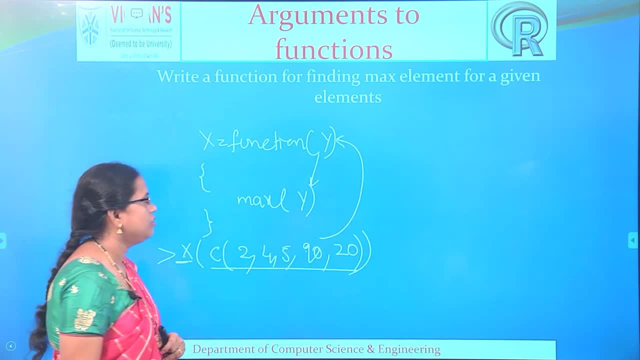 execute this max of y you are going to have. you are going to have maximum element, okay, So like this, we will execute. And if you want to see, if you want to pass more values, x of c of, okay, So 14,, 41,. I am going to give other input: 22,, okay, So 32,, 19,, 76,. 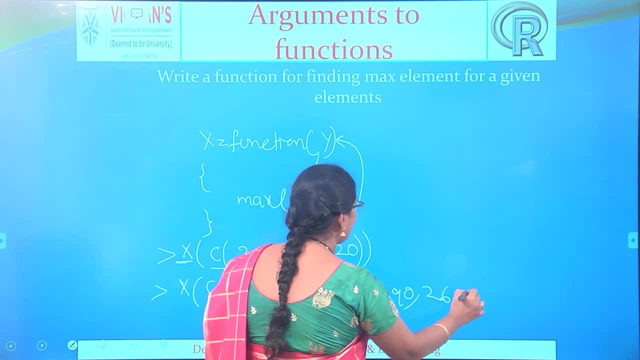 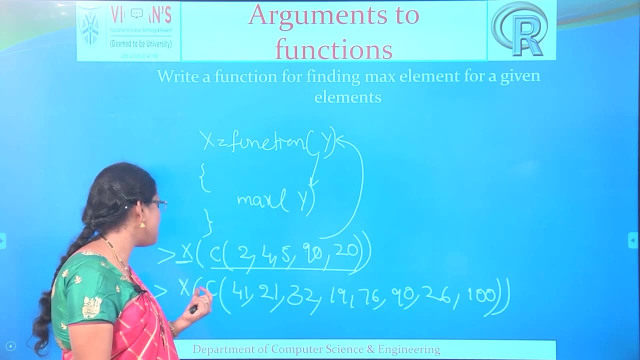 okay. So like this, I am going to pass the input: So 12. So 12., 12. 12.. I do not know the size of the input here, so I am going to pass the multiple elements. 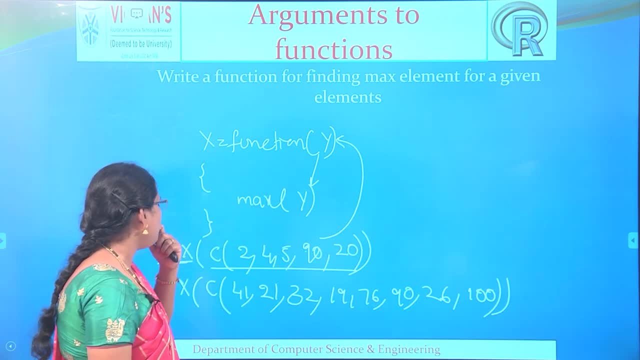 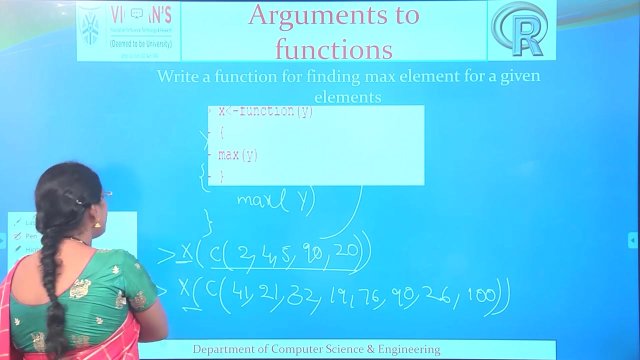 here x of c of. okay. so when you pass this, okay, this entire input will be the y value, okay. so for your understanding, I have given the screenshot here. this is my input: x is equal to function of. okay, so x is equal to function of y. so max of y. our task is: 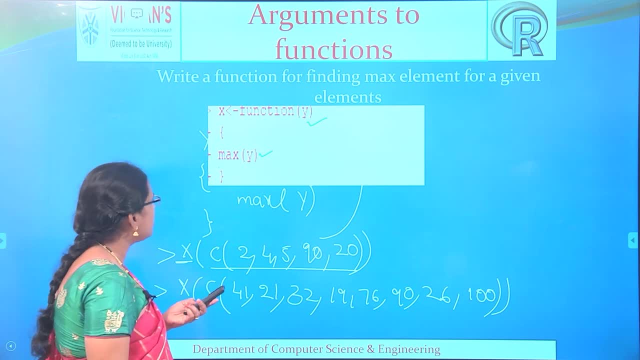 finding the maximum element for a given element. right, so, and then next, this is the calling function. okay, so x of c of. for the first, I have passed 1,, 2, 3 as my input to hold. 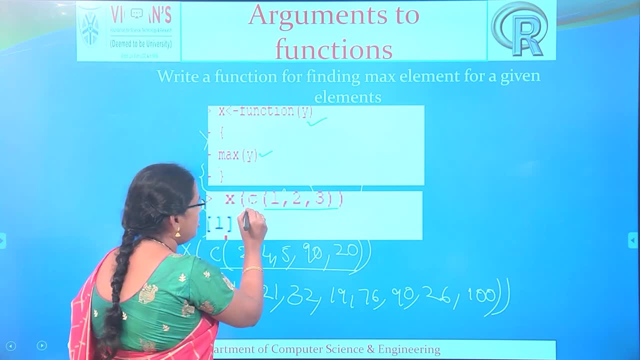 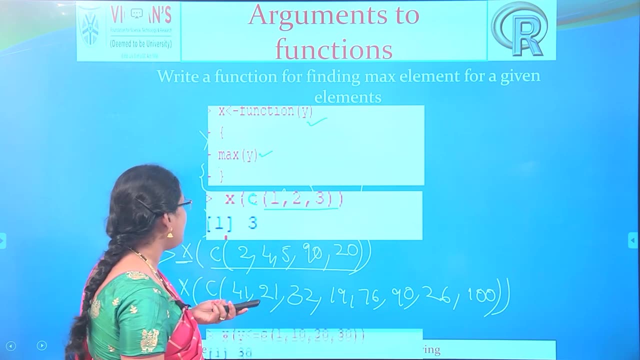 multiple inputs. you need to give the value as x of c. okay, so you need to make use of the c function c of 1,, 2,, 3 and then next. if you want to pass other input, you can also. 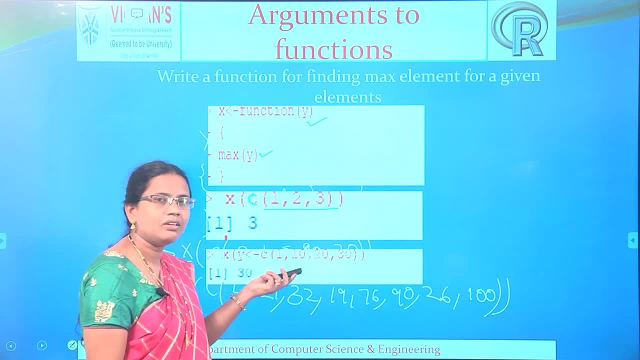 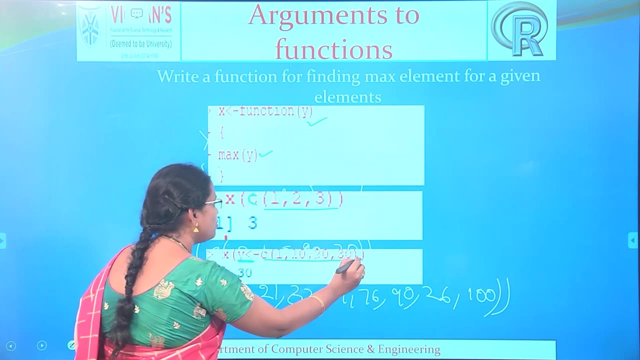 pass other input like this: you can also pass other parameters like this: x of c of x of y is equal to. I have specified the y value. I have stored all these values, all these set of values, in y. I can also call the function like this: so x of y is equal. 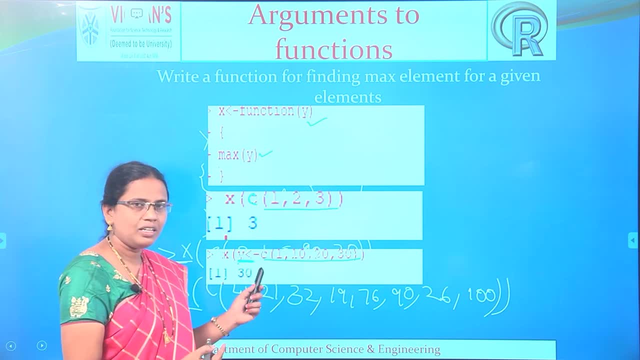 to c of. I have stored the set of elements for y here and then I am passing. okay, so next I can also call the function like this: so x of 1, 10, so I can pass some set of numbers. 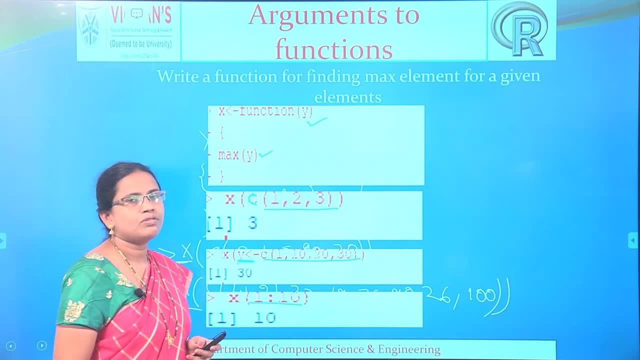 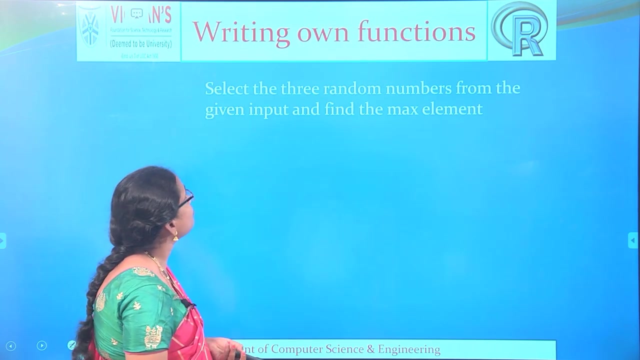 here. so x of 1, 10,. so if I want to find out the sequence of numbers, maximum maximum elements from a sequence of numbers, then in that case x of 1, 10,. these are all the different ways for passing inputs to the arguments. okay for a function, and then next writing. 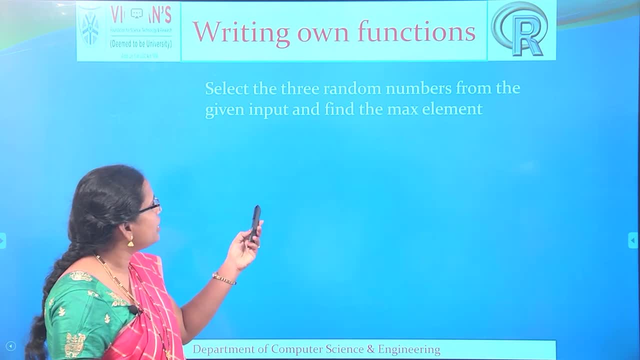 our own and then next let us see, okay other example to understand it clearly. this is the given task, so select the 3 random numbers from the given input and find the maximum element. okay, so the question I am going to repeat. so select the 3 random. 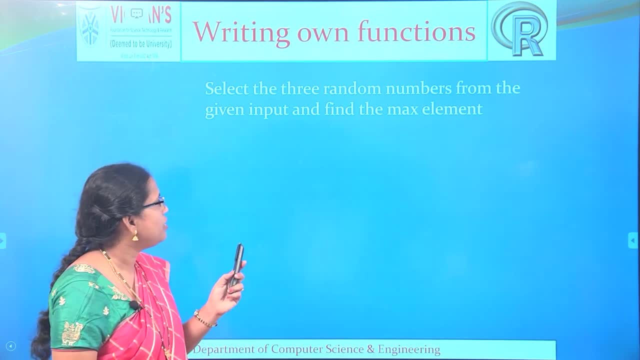 numbers from the given input and find the maximum element. okay, So there are some set of elements. you need to select random 3 random numbers from it, from it and then after that, you need to find out the maximum element. okay, so let us create. 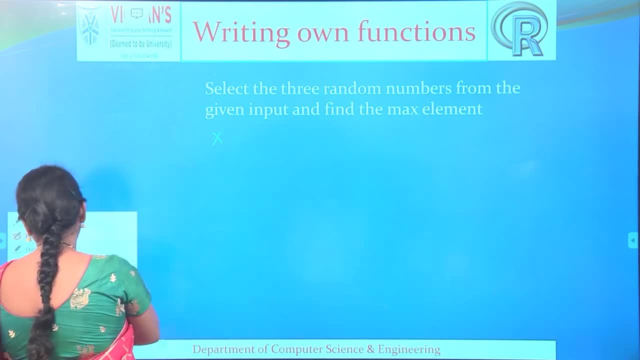 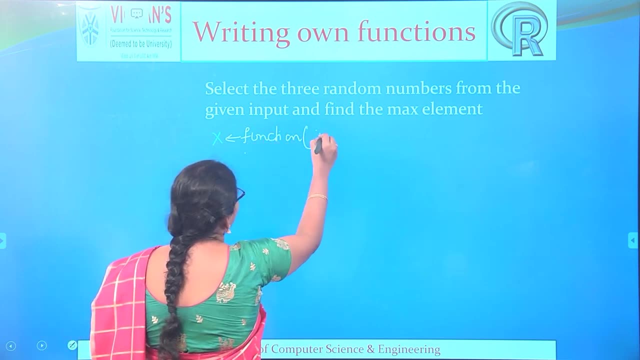 it. so x is equal to. let my variable name is x. let my variable name is x. x is equal to. so function of. okay, so function of. I am going to pass this as y, input as y, okay. 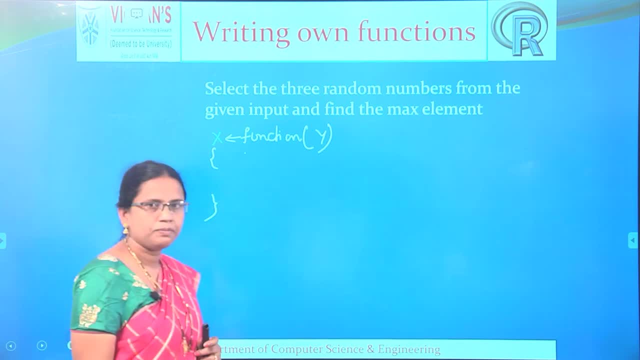 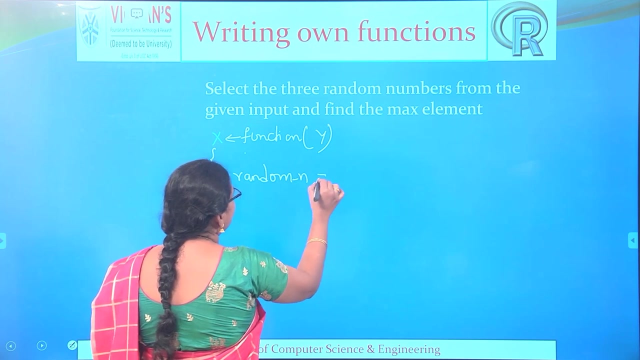 Now the size of the input. that is why I am going to give y. and then after that, what is our task? we need to read 3 random numbers from the given input. okay, so let us take- I am going to take- one variable, that is, random numbers. okay, so random n or random numbers. 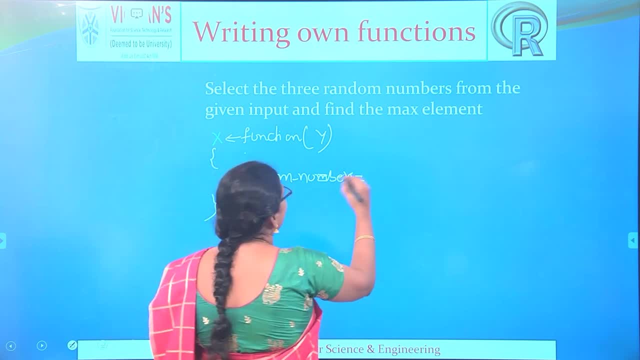 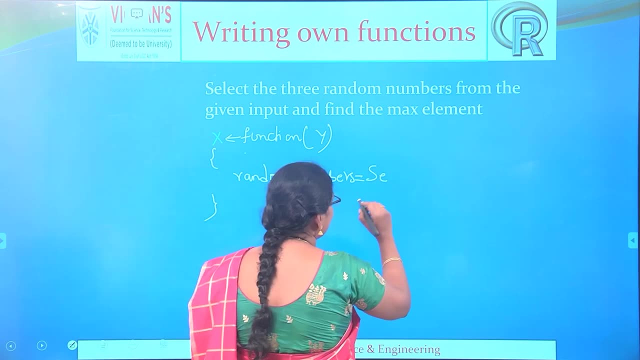 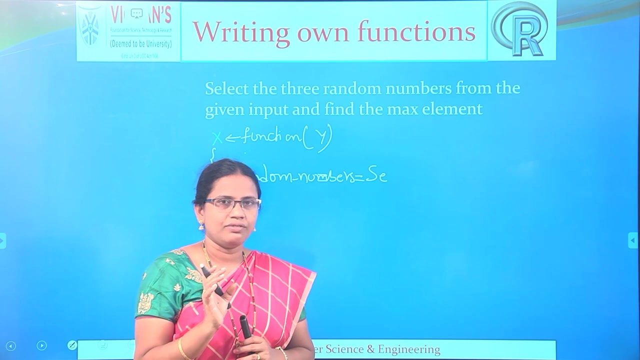 random numbers is equal to okay. so what is our task? from the given random number, from the given input, you need to select 3 random numbers from the given input. okay, so what is the function that you can use for finding the random numbers? you can use sample. 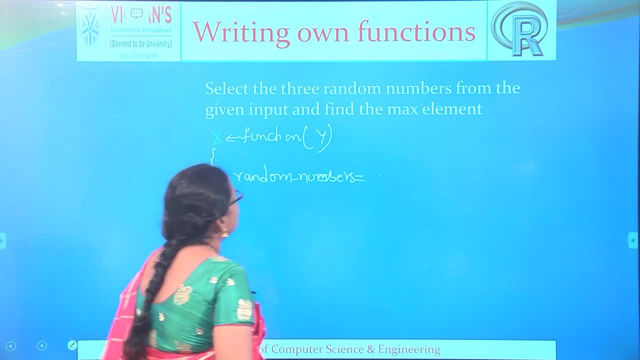 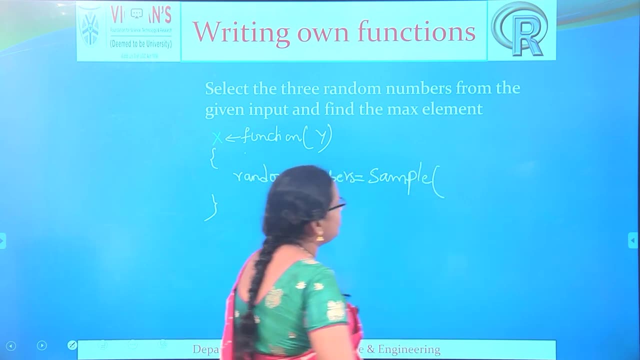 function. okay. so sample of. so random numbers is equal to. I am going to make use of the sample function, so sample of: okay. so how many numbers you want? you want 3 numbers, right? okay, so for that you need to give. 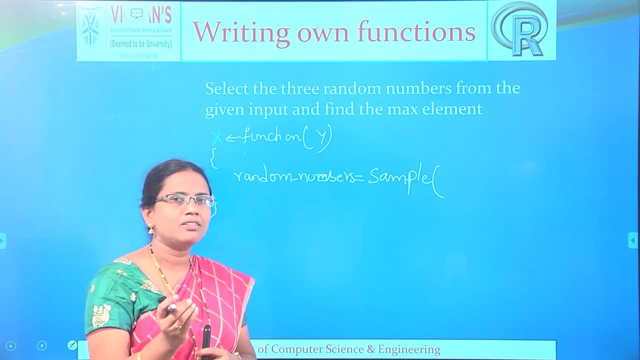 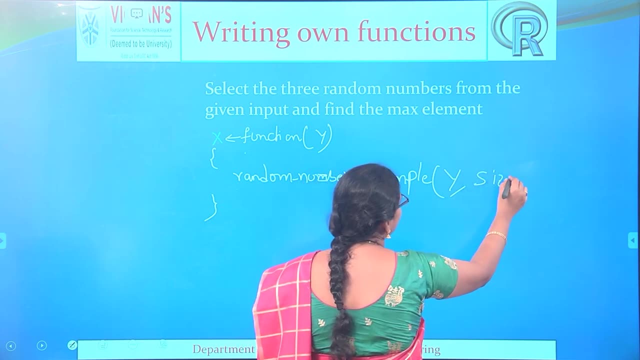 What is the input? From the input, you need to select 3 numbers. okay, so your input is y. okay, so from the input, you need to select 3 numbers. so you have to specify the size as 3, so y comma. 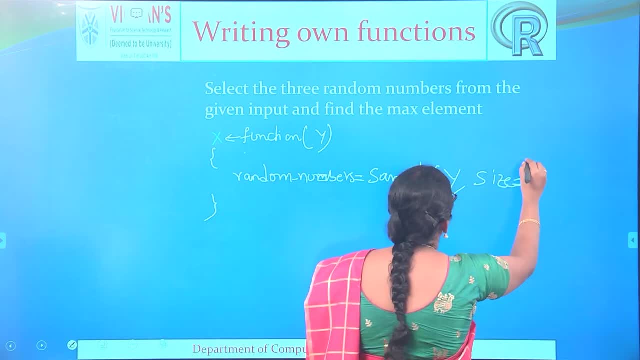 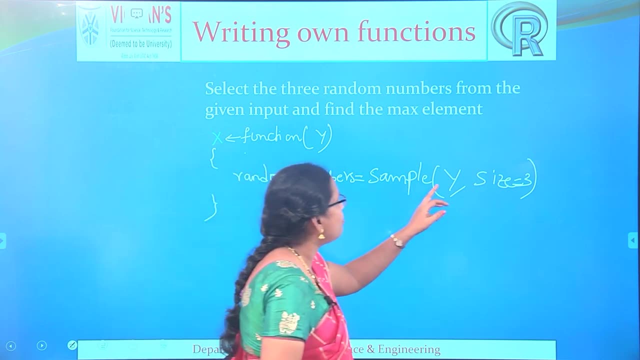 size is equal to 3,. okay so, and then I am going to close it. okay so, random numbers is equal to sample of y. comma size is equal to 3, that means that I am going to select 3 random numbers from the given input. 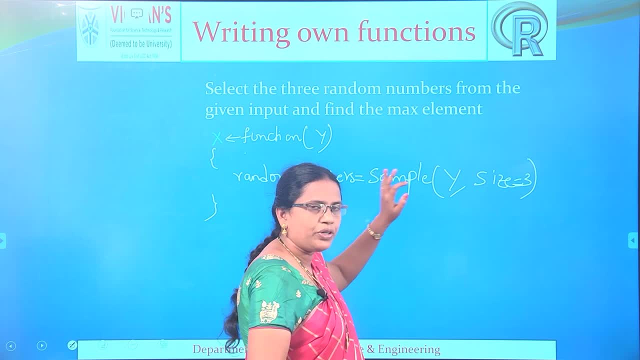 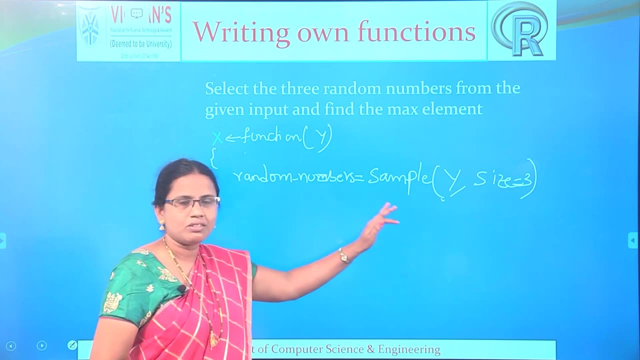 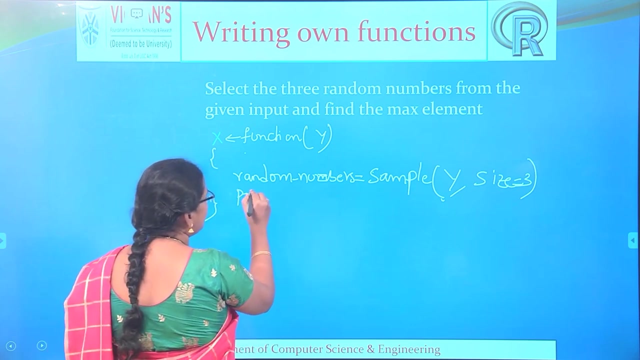 And I am going to store these input. okay, so I am going to store this random numbers with the variable. okay, random numbers. okay, so I am going to store these random numbers in the variable as random numbers. okay, After that, if you want to see the random numbers which are selected, then what you? 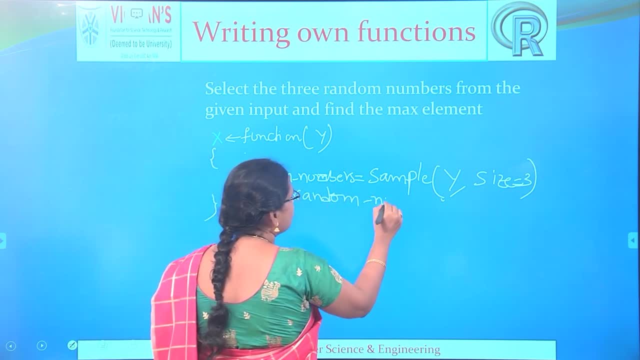 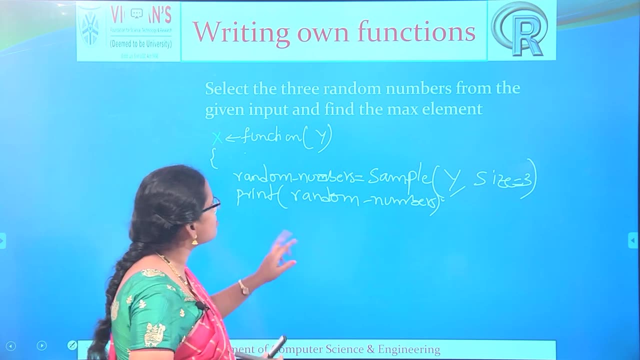 will do. You have to write the command like this. so print of random numbers, right, and if you want to find the maximum element, Our task is completed. Okay, First task is completed: selecting 3 random numbers. so we have selected 3 random numbers. 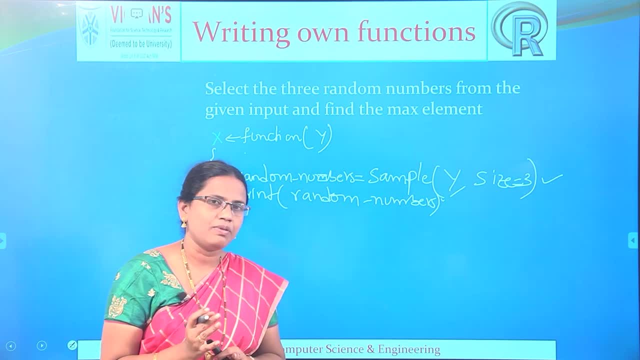 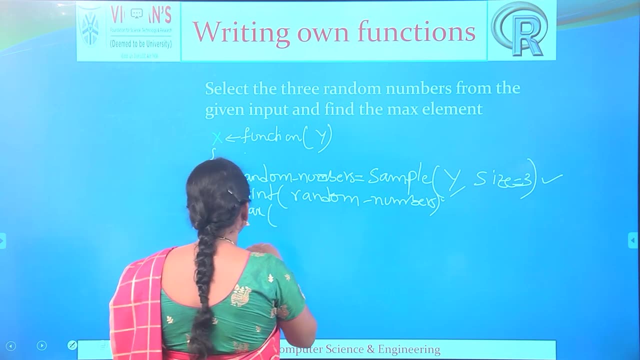 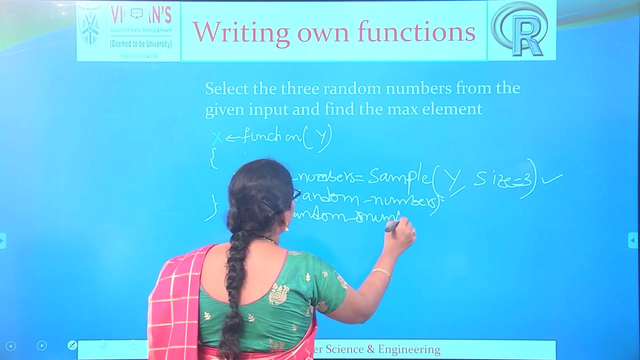 by using this command and after that you need to find out the maximum element from those numbers, right? So how to do that? okay, so, max of. you have to write max of. okay, max of random numbers. your input is: your selected numbers are stored at maximum numbers, right? okay, so max of. 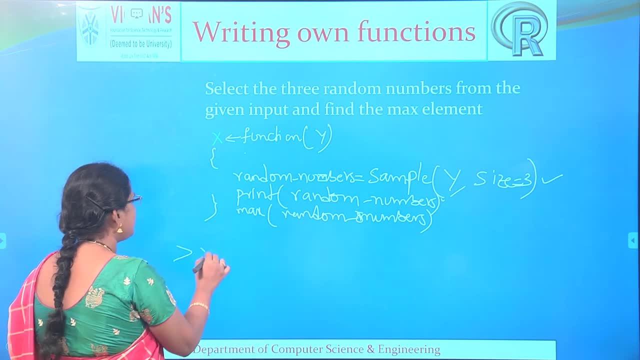 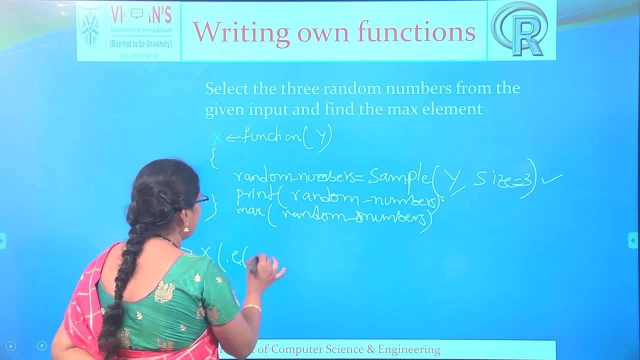 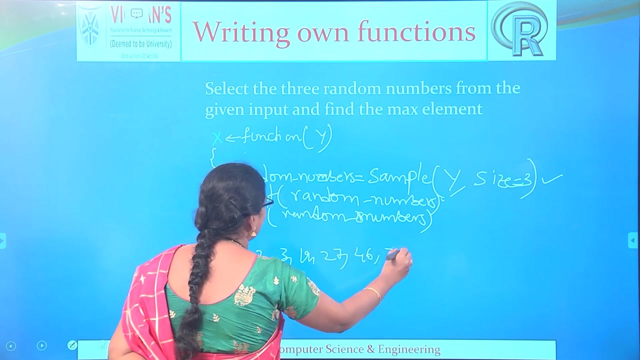 random numbers. Now let us see how this function is called. Next we need to close this function and how to call this function. So x of. I am going to pass some set of elements: X of C. okay. so X of C. okay. so like this: 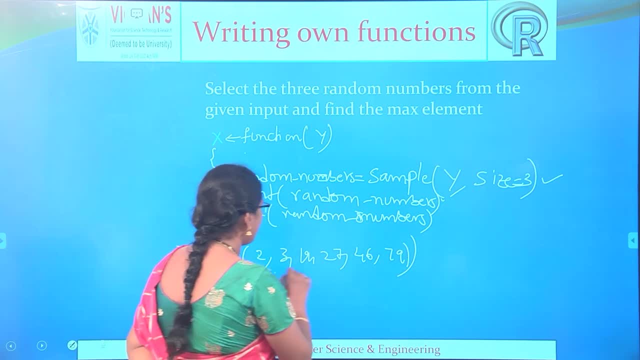 I am passing. So this C, this entire set of elements, are going to be given as input for the y. So this is the input that I have given. So from this input I am going to store the value of the, that is not the number, because 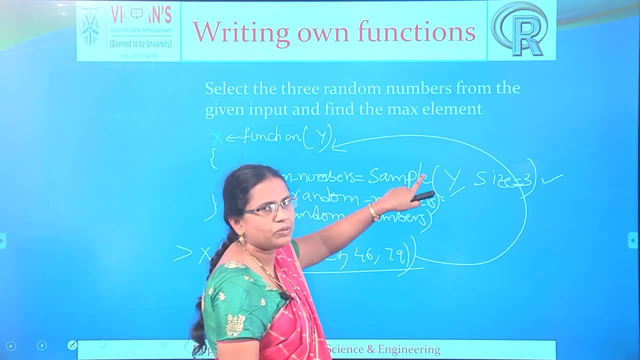 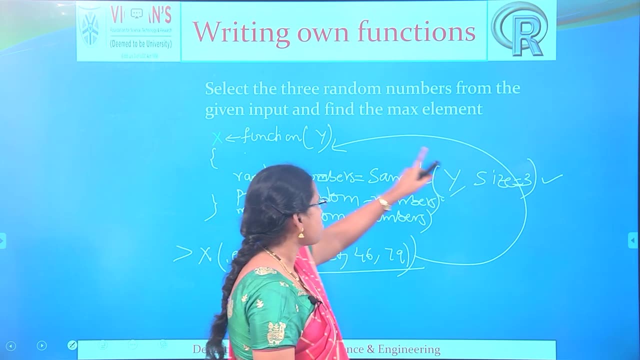 I have given the value, that is the value of the number. The number is 2.5.. select 3 random numbers. okay, by making use of the sample function. So you will select 3 random numbers by specifying the size is equal to 3 and store that numbers in one variable that is random. 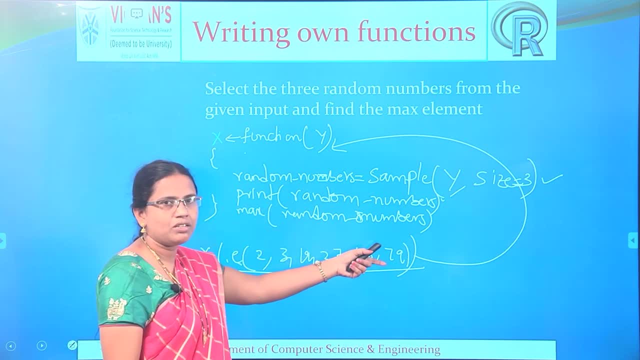 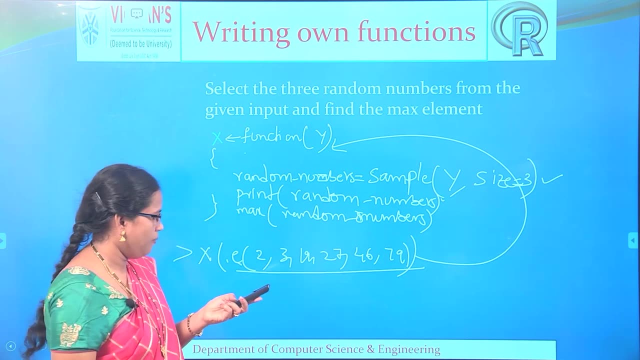 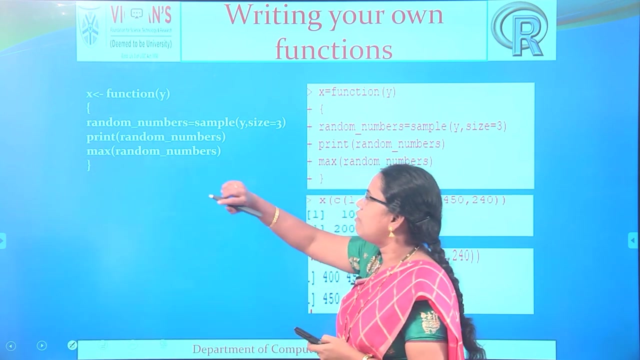 numbers and our task is to find the maximum element from the selected random numbers. So make use of the max function. so max of random numbers, right, okay. So next let us see see. this is the function I have written. So this is the function. So x is equal to function of y. 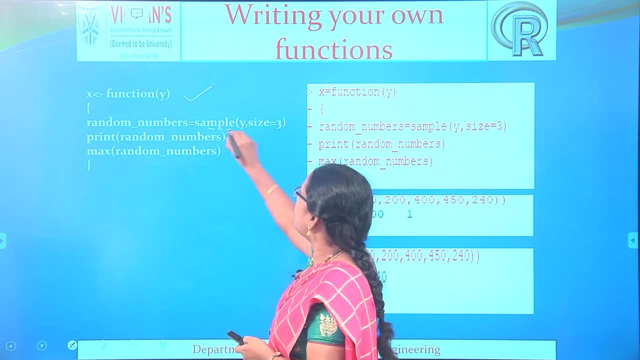 this is the function and then sample of y, comma size is equal to 3.. So this is my input. So from this input I have to select 3 random numbers. size is equal to 3, and then I want to find out the. 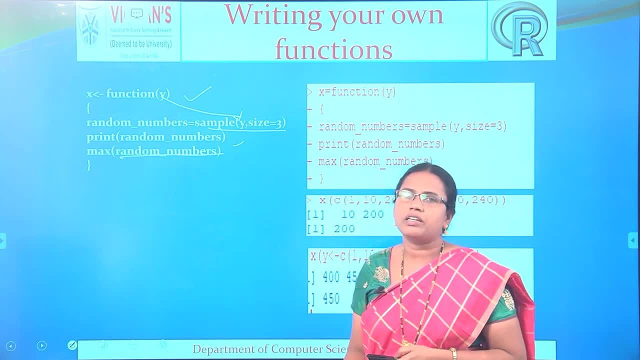 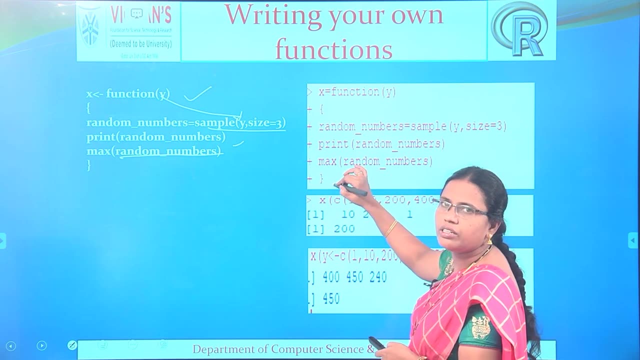 maximum element from the given random numbers. So I have to give the command as max of random numbers, right, and then if you want to call this function like this, okay, So this is my function that is executed in our console and I have provided screenshot here. and then, if you want to pass this, 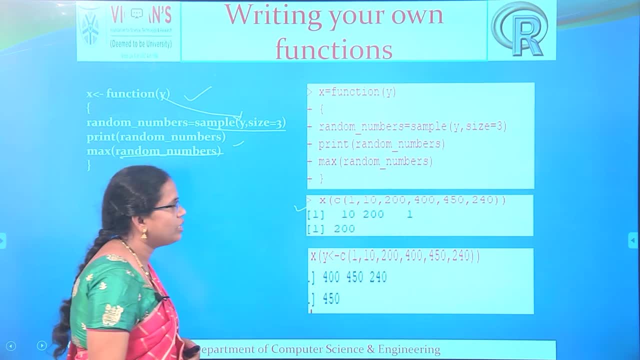 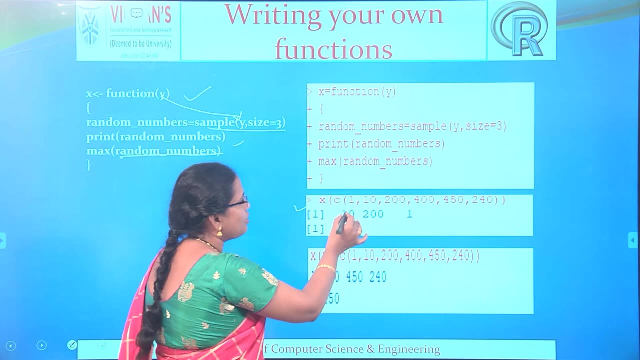 okay, So x, x of c of this is my input that I have given, and this is the one way of giving input. and then this is the other way of giving input. You can see here from 1, 10,. okay, you can see here from 1,. 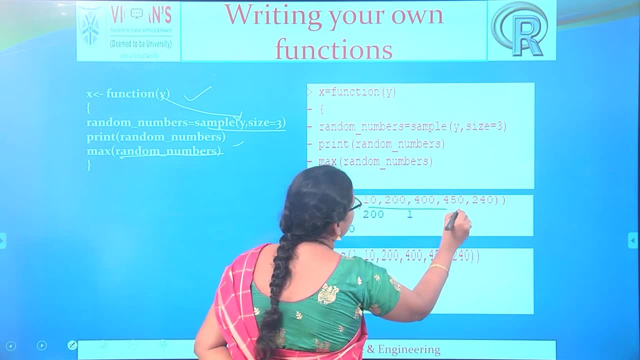 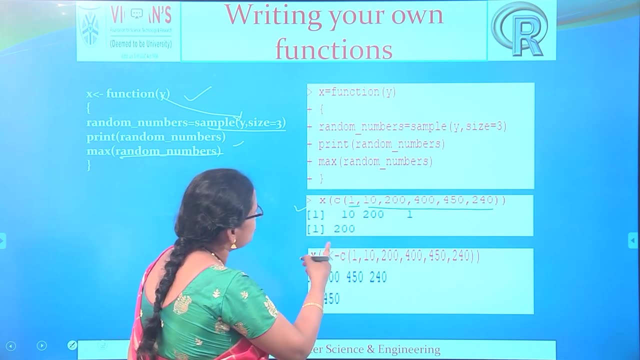 10, 20,, 200, 400,, 450, 240. we have okay. So the maximum numbers are: we have the numbers, that is 200, okay, and then next Other calling: okay. So I have called other function, I have called with other input, So 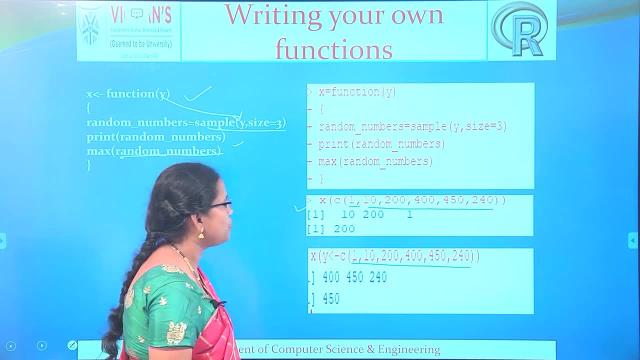 this is my input: 1, 10, 200, 400, 450, 240.. So for the next sample I have 3 numbers. Those are, these are the selected numbers. I have printed. okay, So, because I have printed here. So. 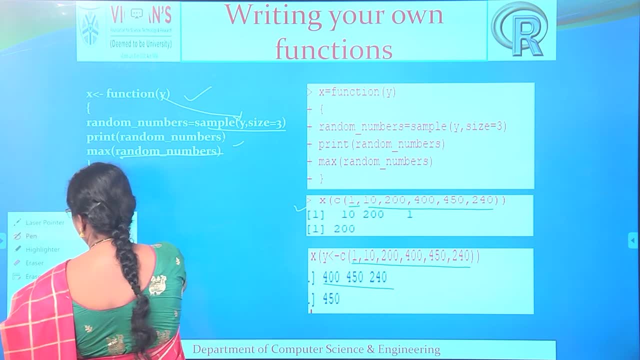 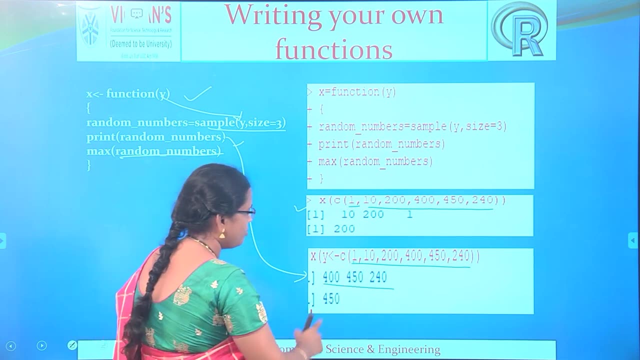 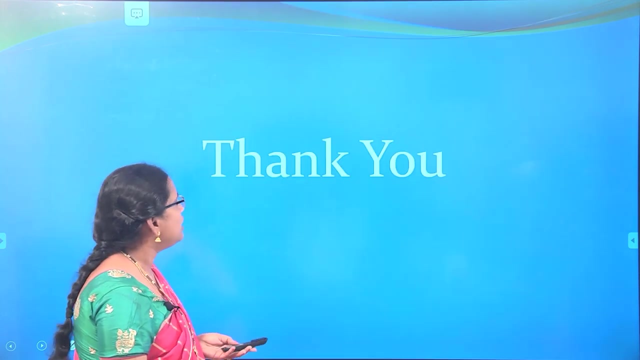 the numbers are printed here. So I have printed. So the numbers are printed here. print of random numbers. So 400, 450, 240.. So what is the maximum Here? 450 is the maximum here. Like this: you will write your own functions, okay, And then by this: 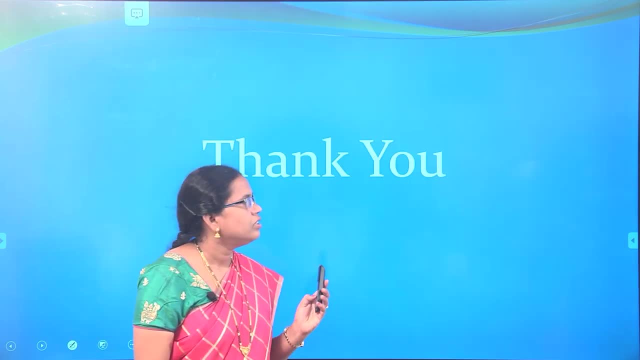 okay, So this is the end of the class. So in this class we have seen: we have seen how to work with predefined functions in R and how to work with a sample function and how to work with sample with replacement function. and then we have seen how to create our own functions. and then we have 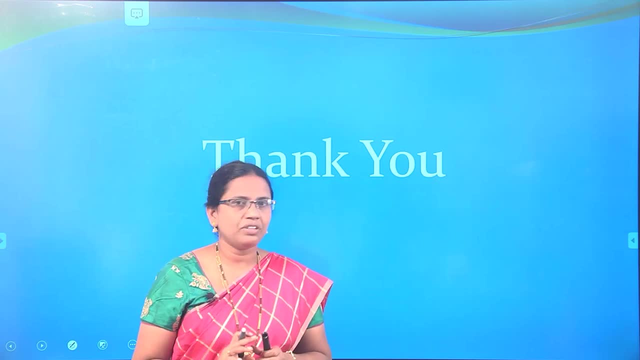 seen how to create, how to pass some arguments to the functions. okay, So this is the end of the class. You need to practice all the given questions in your R console. okay, Thank you. 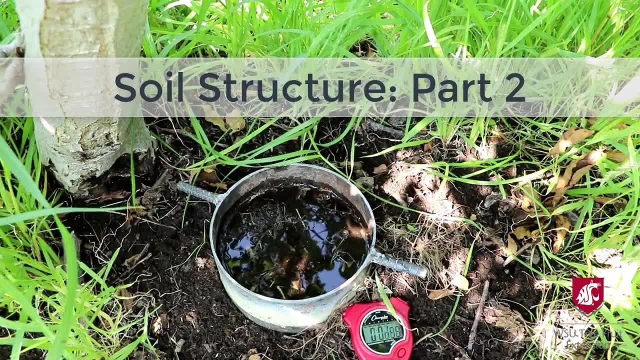 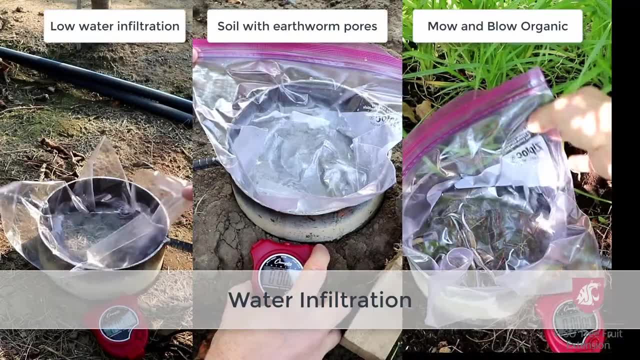 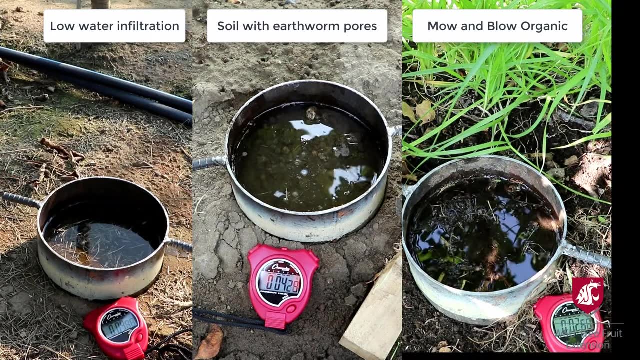 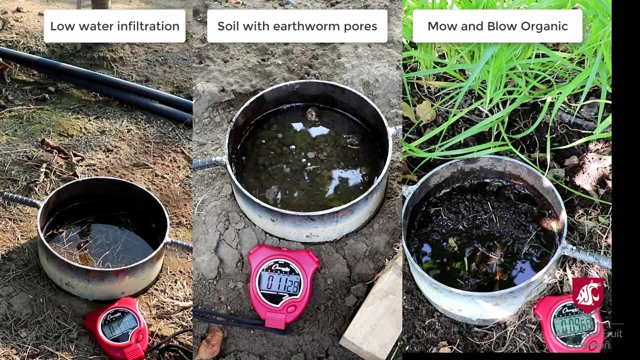 Another indicator of soil structure is water infiltration. We measure water infiltration by pounding a ring into the soil and recording how long it takes for one inch of water to infiltrate. In soils with lots of aggregation and low compaction, large pores caused by earthworms and plant roots will allow water to infiltrate quickly and little water will run off. 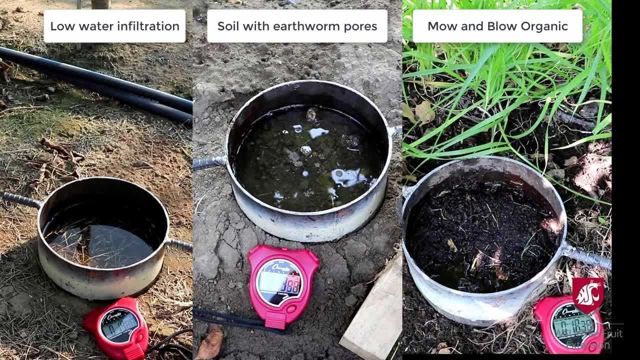 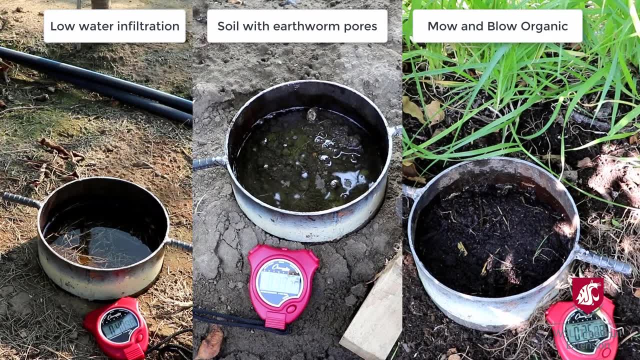 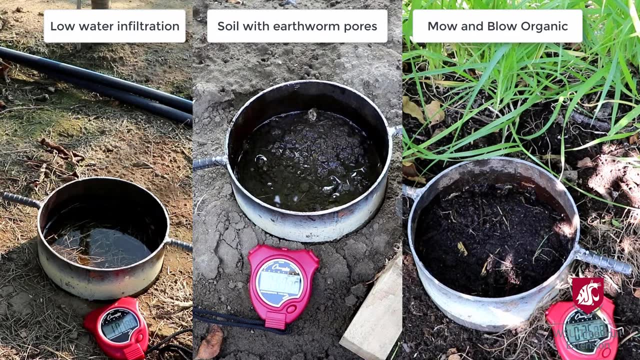 Management practices in orchards can impact soil structure. For example, in this soil at right, the tree row is mowed and mulched and soil organisms have created good soil structure. In the center panel, plentiful earthworms have created channels for water infiltration. In the left panel, surface compaction is likely limiting water infiltration and likely root growth. 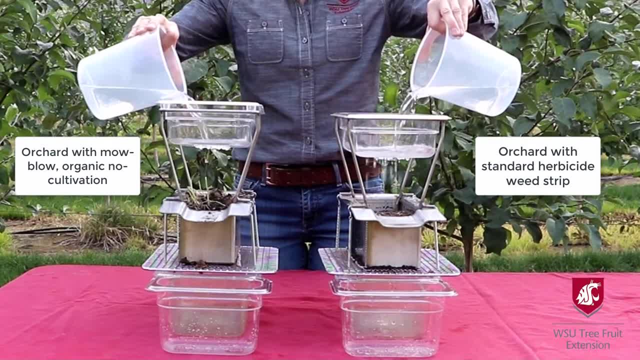 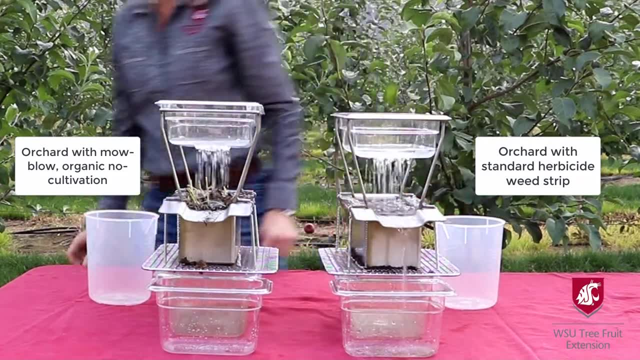 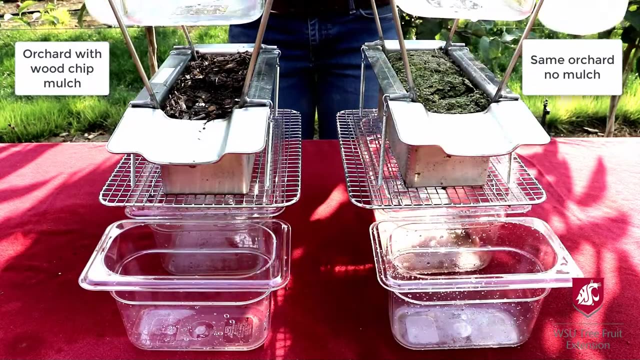 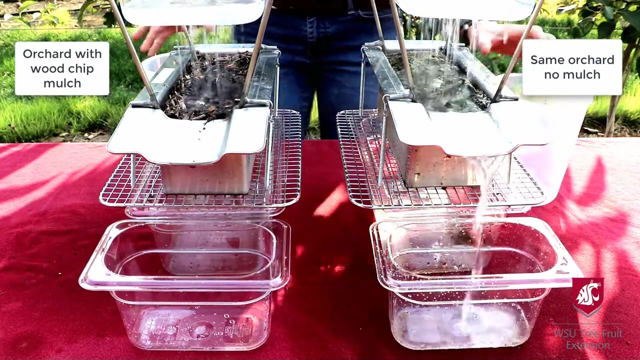 We can also see soil structure differences. with these runoff boxes In the orchard at left, a much greater portion of water infiltrates into lower soil depths. Greater pore space creates a good environment for tree roots and soil microbes. In multiple studies we have seen that wood chip mulch can also increase water infiltration. 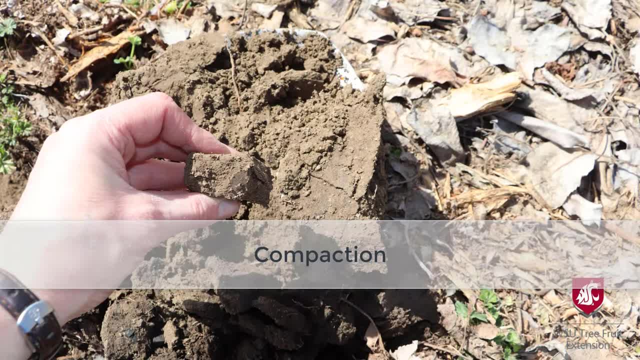 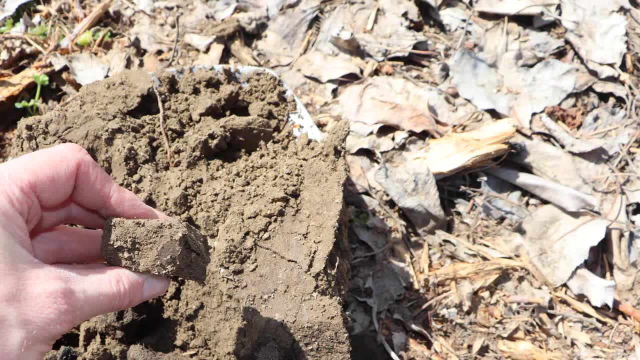 Soil structure can be disturbed by compaction. Soils may have a soil structure that is not suitable for the soil. We can also see a surface or deep compaction layer where soil particles are pushed close together, limiting root growth as well as access to water and nutrients. 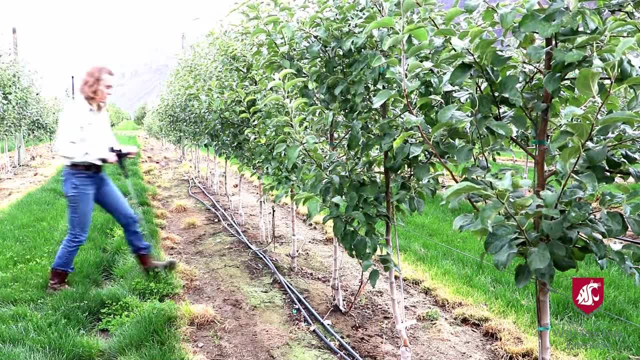 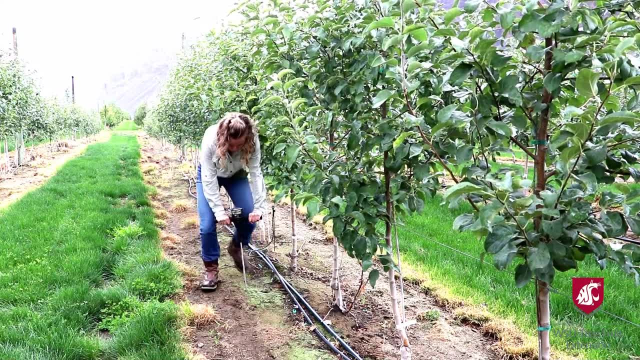 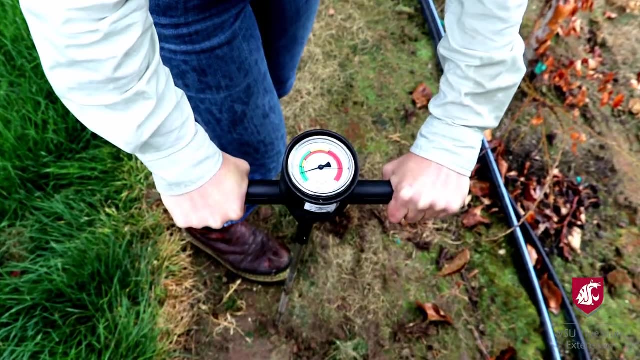 We can estimate compaction by measuring the force required to penetrate the soil using a soil penetrometer. Push the tip of the penetrometer into the soil using slow, even pressure when the soil is at field capacity. When the gauge reaches above 300 psi, compaction may be impacting plant roots.